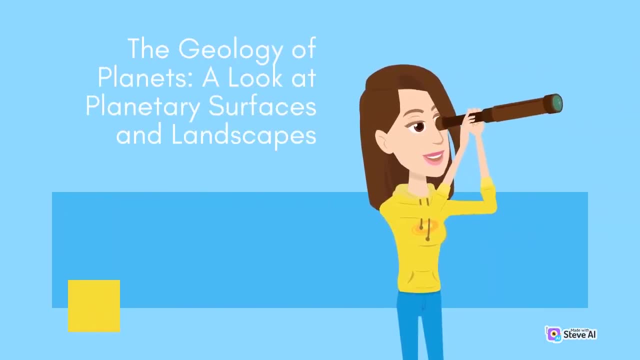 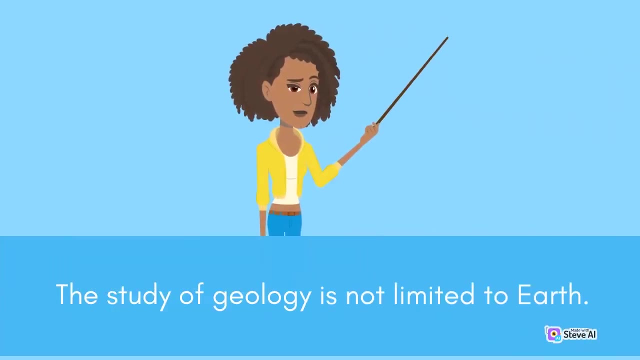 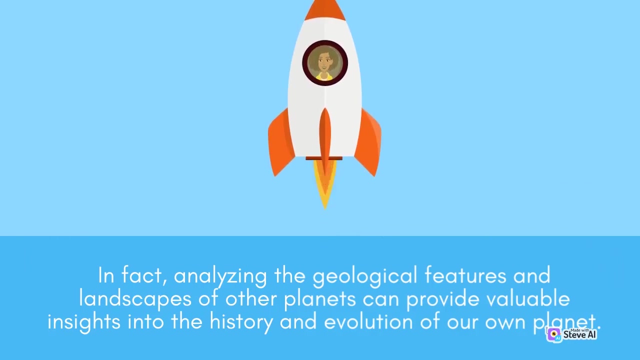 The Geology of Planets: a look at planetary surfaces and landscapes. The study of geology is not limited to Earth. In fact, analyzing the geological features and landscapes of other planets can provide valuable insights into the history and evolution of our own planet. 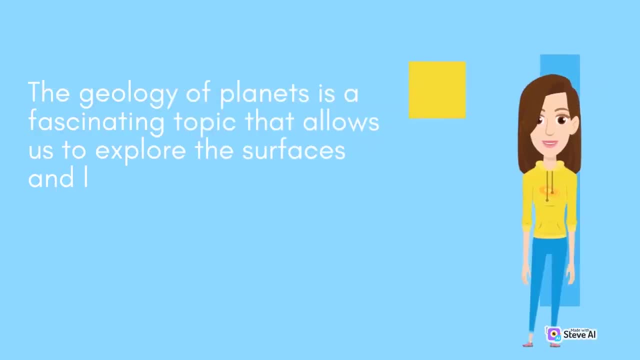 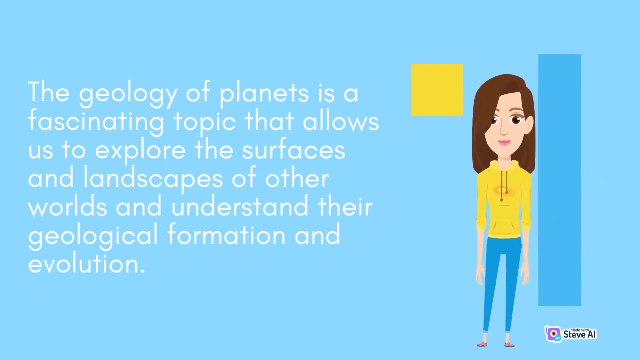 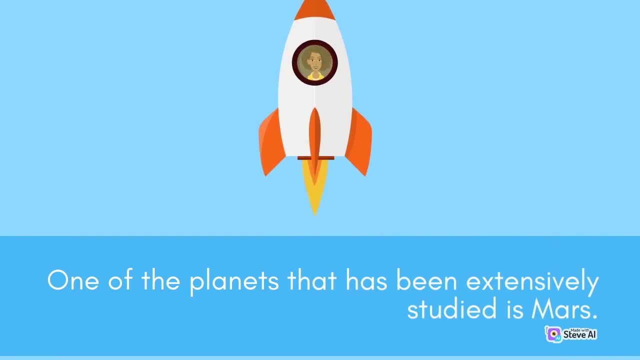 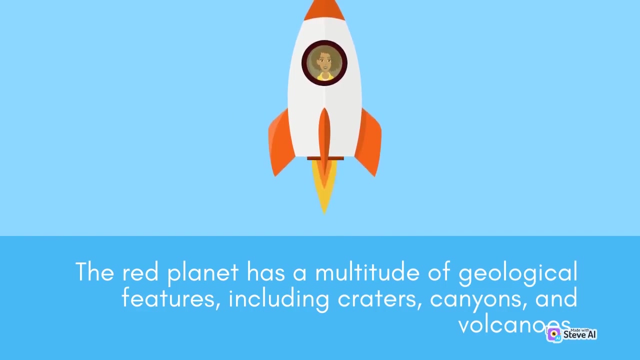 The geology of planets is a fascinating topic that allows us to explore the surfaces and landscapes of other worlds and understand their geological formation and evolution. One of the planets that has been extensively studied is Mars. The red planet has a multitude of geological features, including craters, canyons and volcanoes. 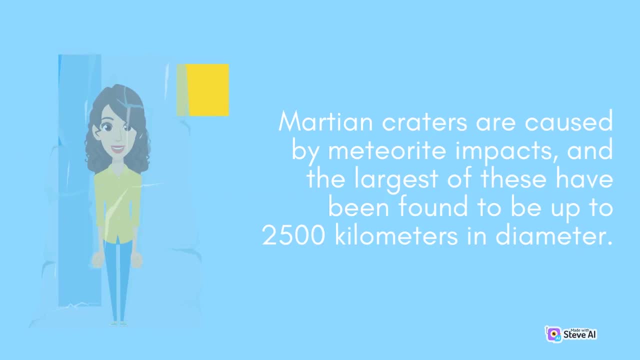 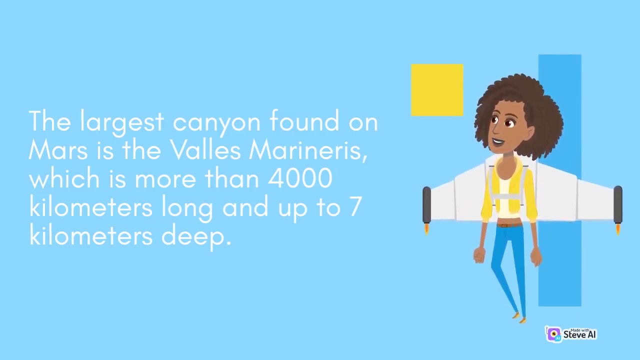 Martian craters are caused by meteorite impacts, and the largest of these have been found to be up to 2,500 kilometers in diameter. The largest canyon found on Mars is the Valles Marineris, which is more than 4,000 kilometers long and up to 7 kilometers deep. 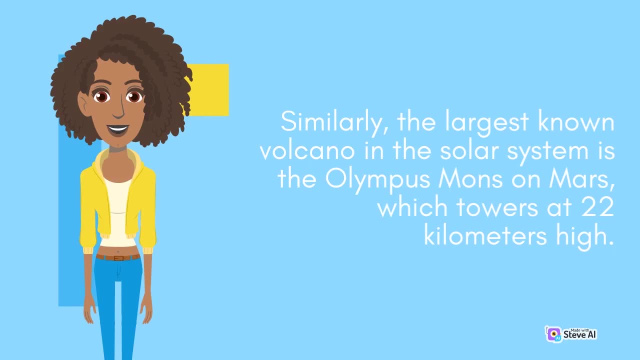 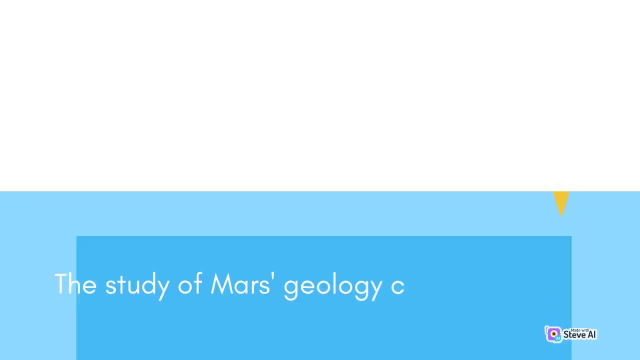 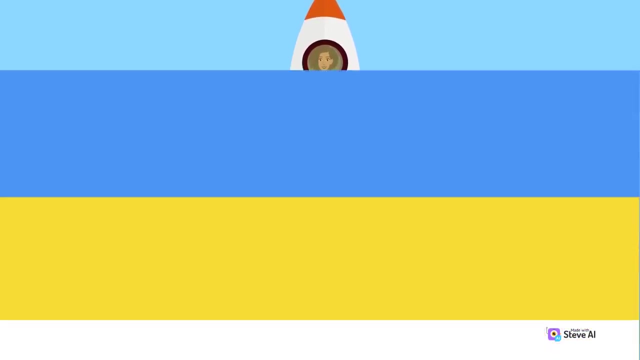 Similarly, the largest known volcano in the solar system is the Olympus Mons on Mars, which towers at 22 kilometers high. The study of Mars geology can also provide us with insight into the planet's history. For example, the presence of dried-up river channels and valley networks suggests that liquid water was once present on the planet's surface. 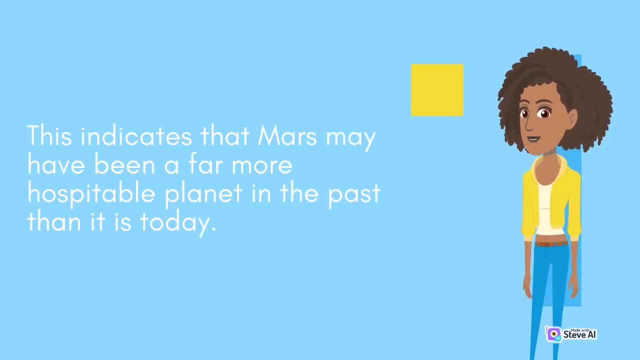 This indicates that Mars may have been a far more hospitable planet in the past than it is today. The formation of volcanoes on Mars also indicates that the Earth was more hospitable on Mars' surface. The formation of volcanoes on Mars also indicates that the Earth was more hospitable on Mars' surface. 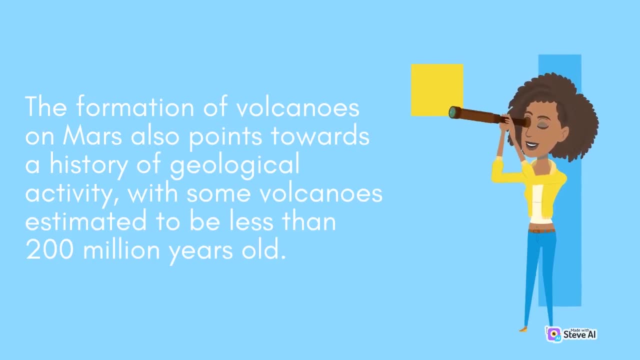 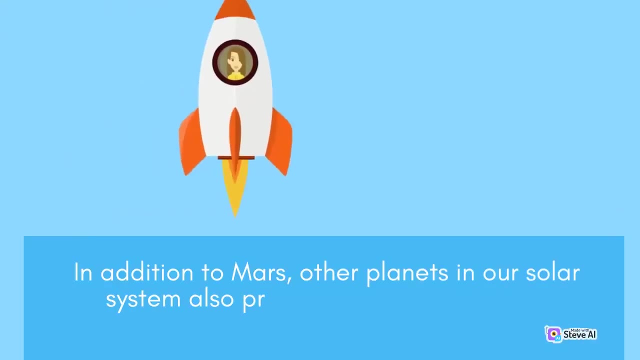 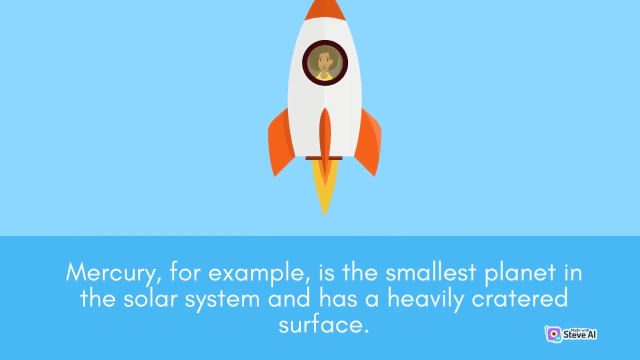 points towards a history of geological activity, with some volcanoes estimated to be less than 200 million years old. In addition to Mars, other planets in our solar system also provide interesting geological features and landscapes. Mercury, for example, is the smallest planet in the solar system and has a heavily cratered 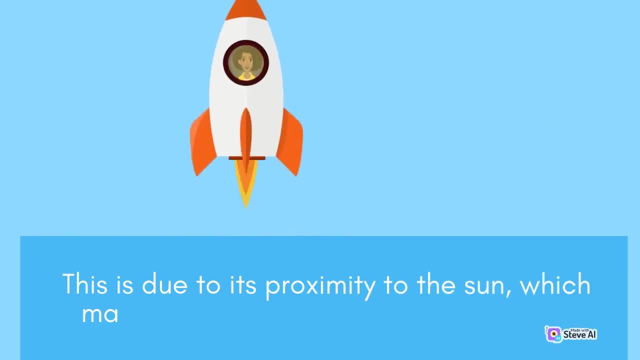 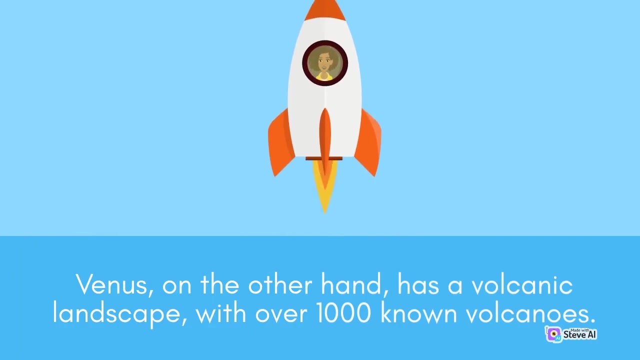 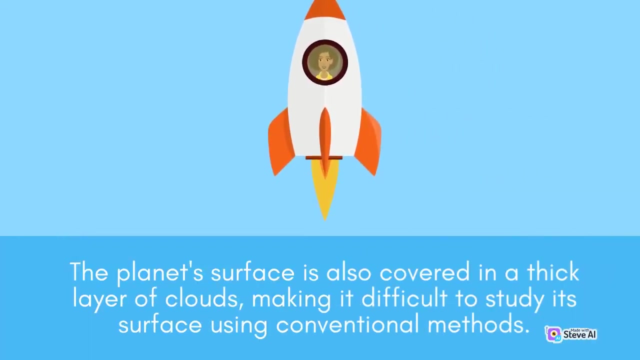 surface. This is due to its proximity to the sun, which makes it vulnerable to meteorite impacts. Venus, on the other hand, has a volcanic landscape, with over 1,000 known volcanoes. The planet's surface is also covered in a thick layer of clouds, making it difficult. 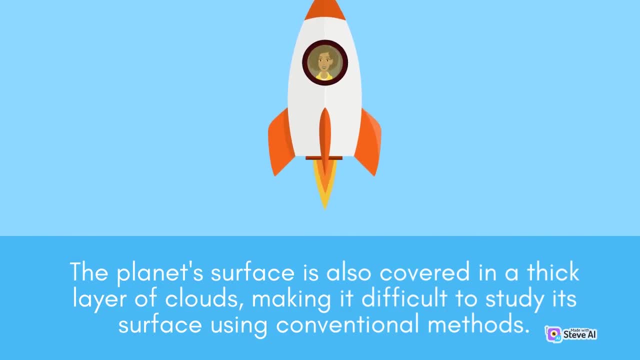 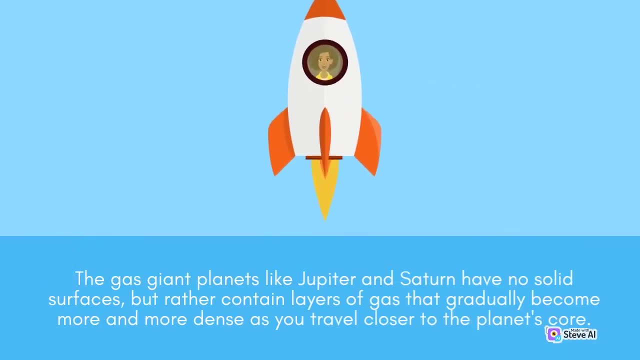 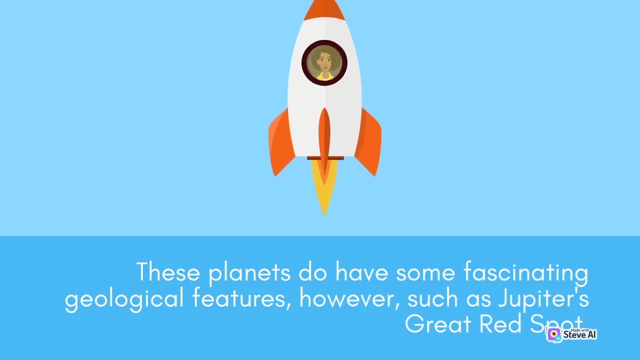 to study its surface using conventional methods. The gas-giant planets like Jupiter and Saturn have no solid surfaces, but rather contain layers of gas that gradually become more and more dense as you travel closer to the planet's core. These planets do have some fascinating geological features, however, such as Jupiter's Great 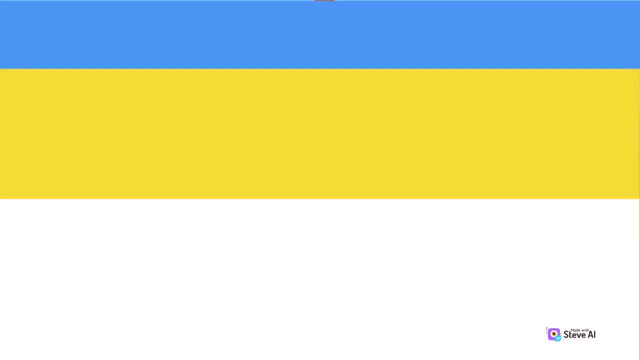 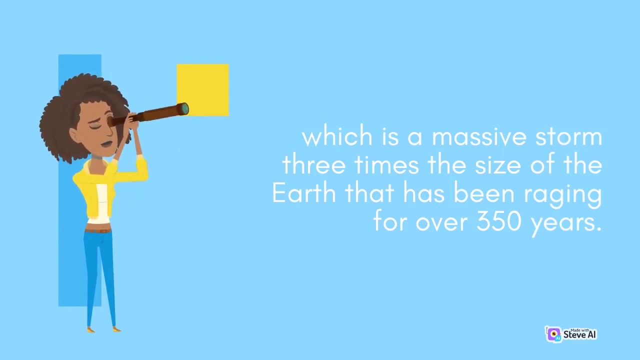 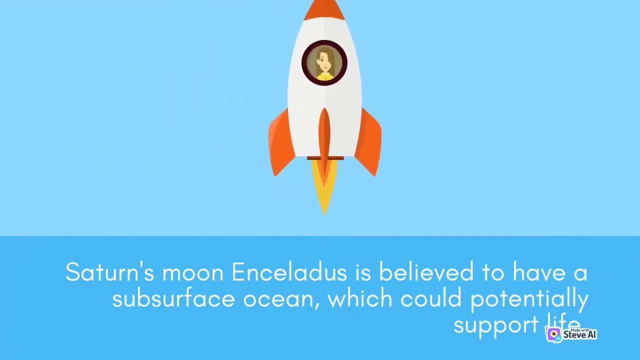 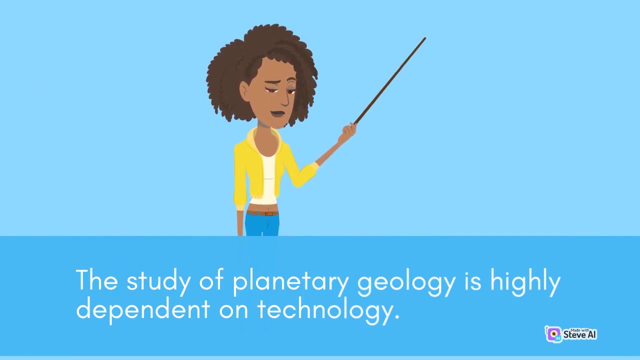 Red Spot, which is a massive storm three times the size of the Earth that has been raging for over 350 years. Saturn's moon, Enceladus, is believed to have a subsurface ocean which could potentially support life. The study of planetary geology is highly dependent on technology. 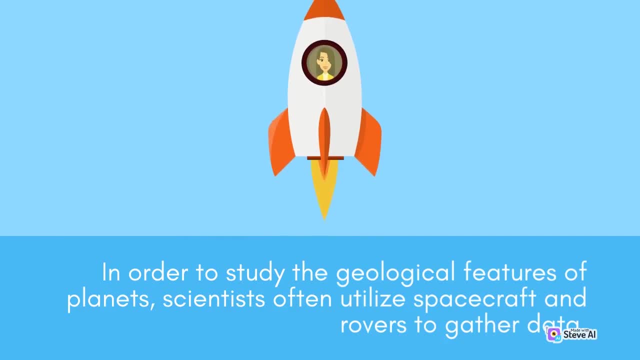 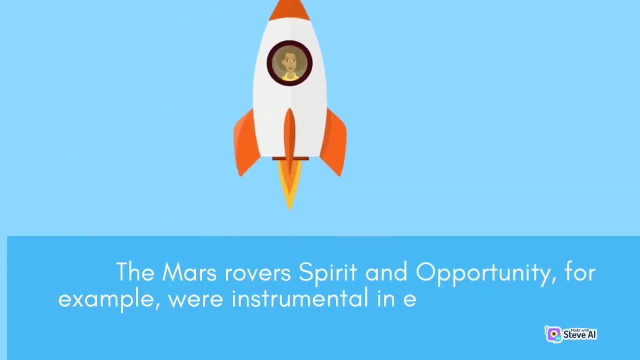 In order to study the geological features of planets, scientists often utilize spacecraft and rovers to gather data. The Mars rover's Spirit and Opportunity, for example, were introduced to the planet by a scientist, and its Mars rover was instrumental in exploring the red planet's Martian surface. 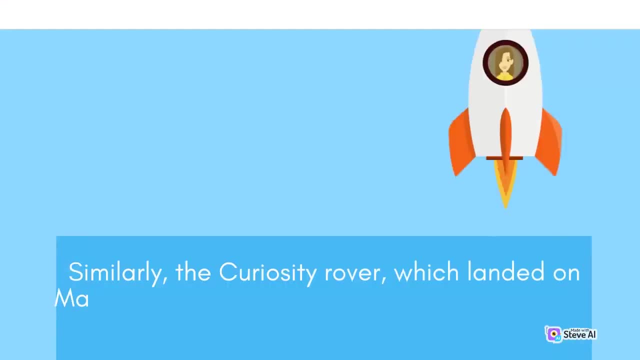 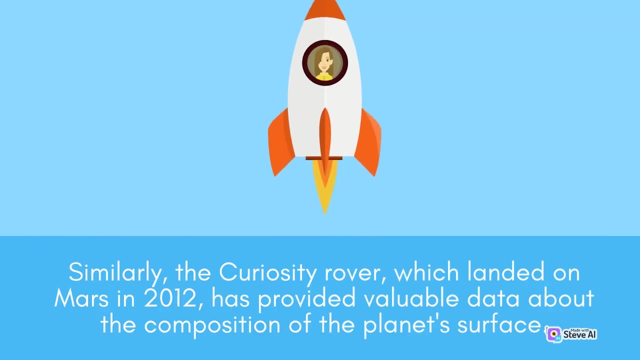 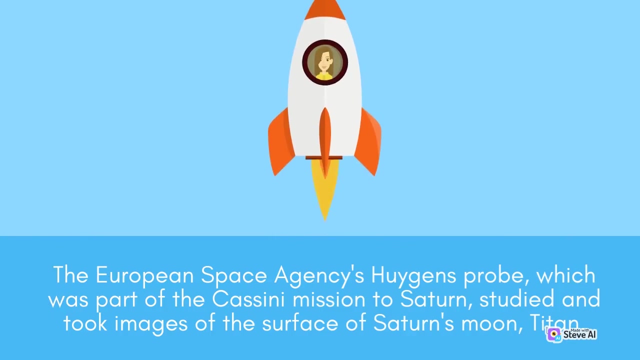 Similarly, the Curiosity rover which landed on Mars in 2012, has provided valuable data about the composition of the planet's surface. The European Space Agency's Huygens probe, which was part of the Cassini mission to Saturn, studied and took images of the surface of Saturn's moon Titan. 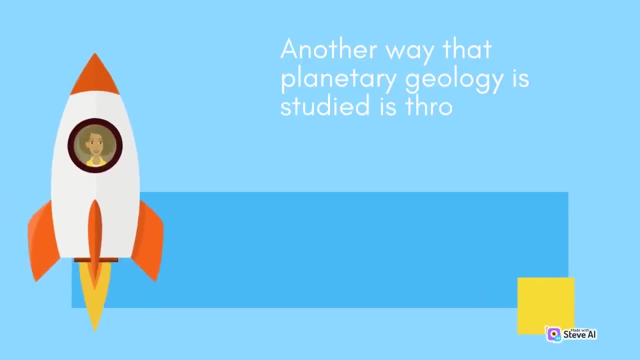 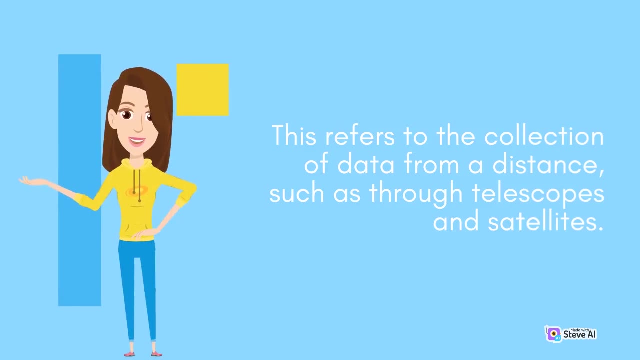 Saturn's moon, Titan. Another way that planetary scientists and scientists have been able to study the surface of the moon is by using the satellite's probe is studied is through remote sensing. This refers to the collection of data from a distance, such as through telescopes and satellites. 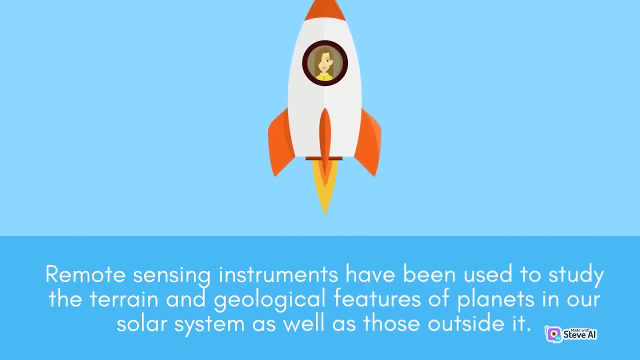 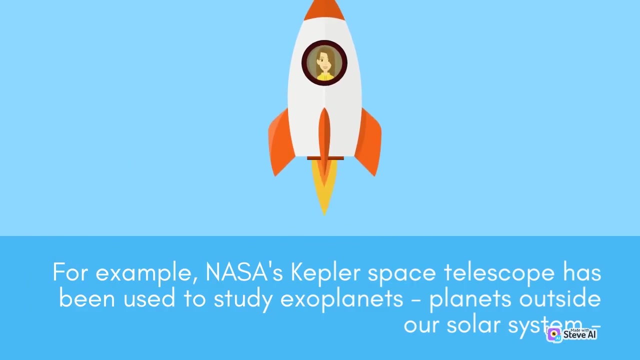 Remote sensing instruments have been used to study the terrain and geological features of planets in our solar system, as well as those outside it. For example, NASA's Kepler Space Telescope has been used to study exoplanets- planets outside our solar system- to see if they have similar geological features to those on Earth and other planets in our solar system. 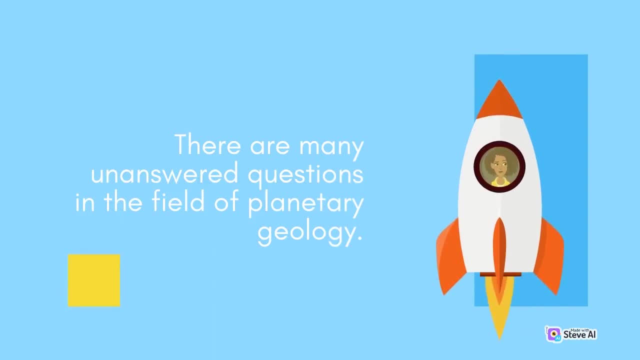 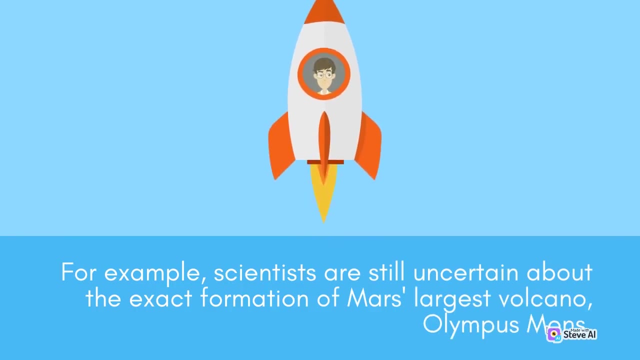 There are many unanswered questions. in the field of planetary geology, For example, scientists are still uncertain about the exact formation of planets in our solar system. For example, scientists are still uncertain about the exact formation of planets in our solar system. For example, scientists are still uncertain about the exact formation of planets in our solar system. 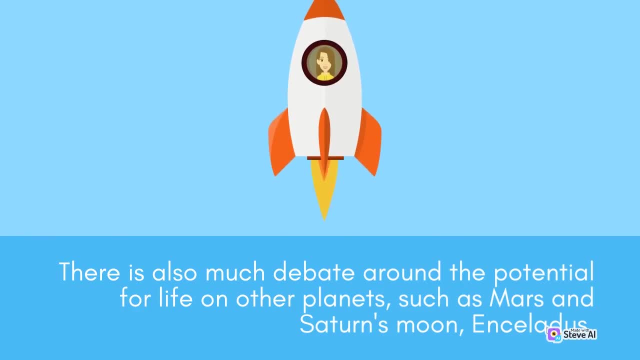 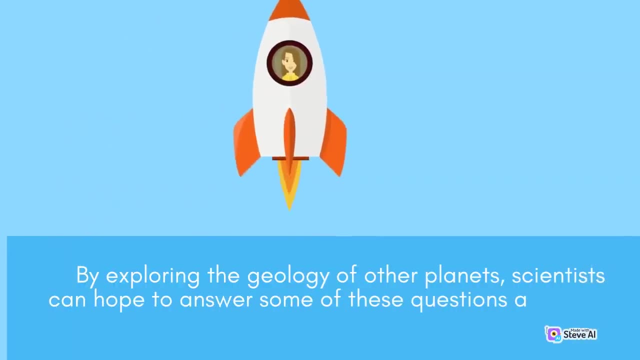 There is also much debate around the potential for life on other planets, such as Mars and Saturn's moon Enceladus. By exploring the geology of other planets, scientists can hope to answer some of these questions and gain a better understanding of the universe around us. 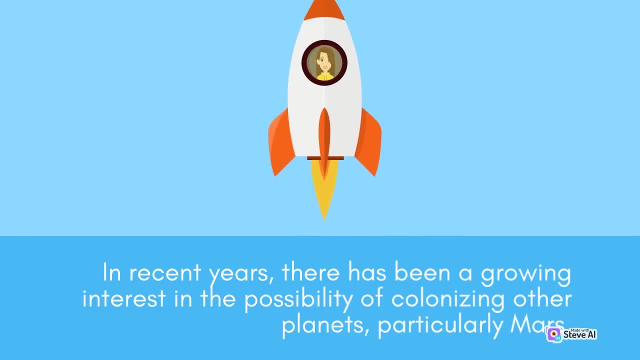 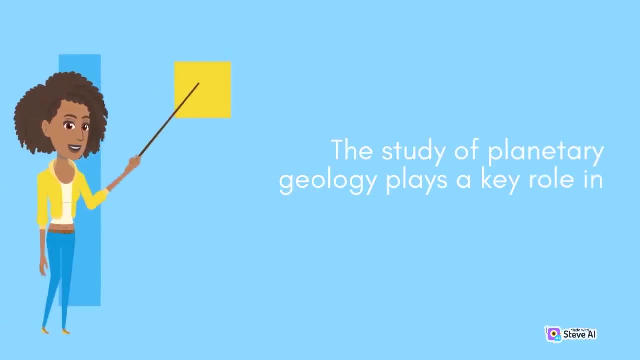 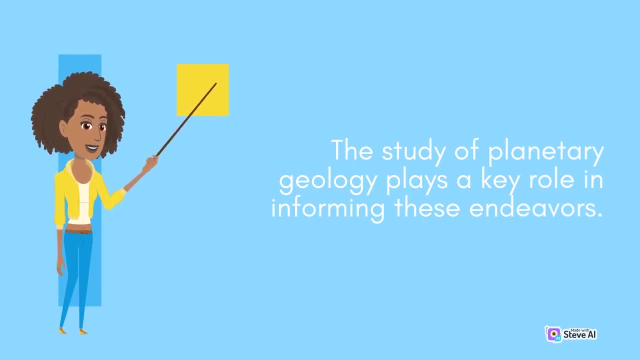 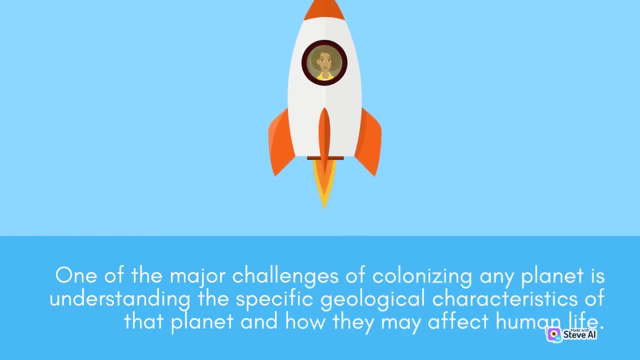 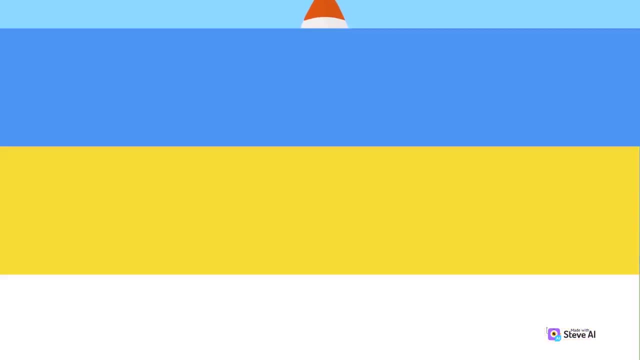 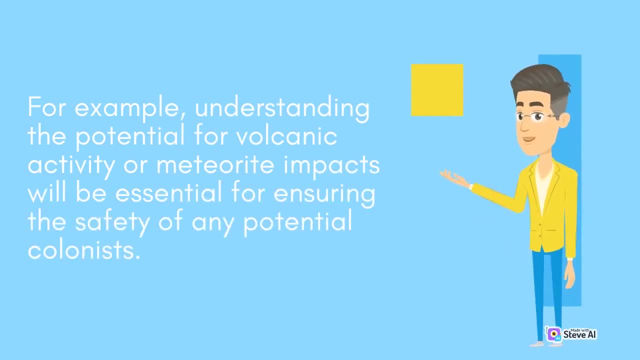 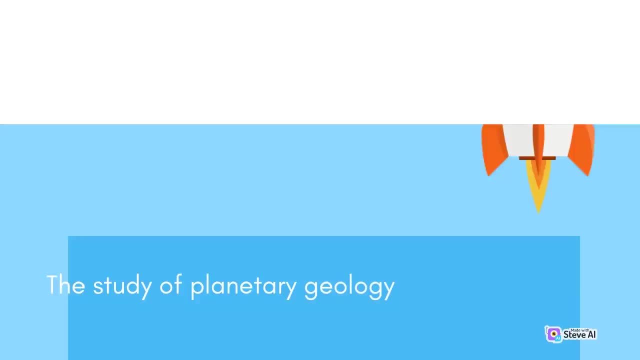 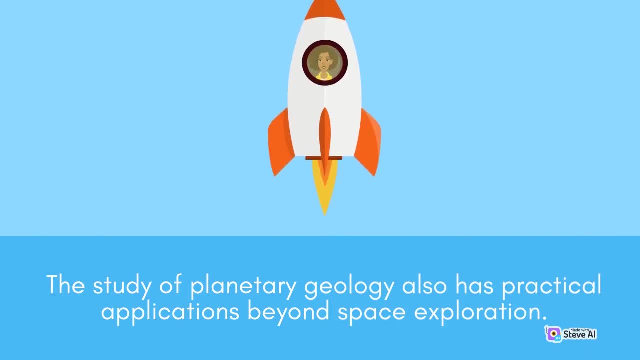 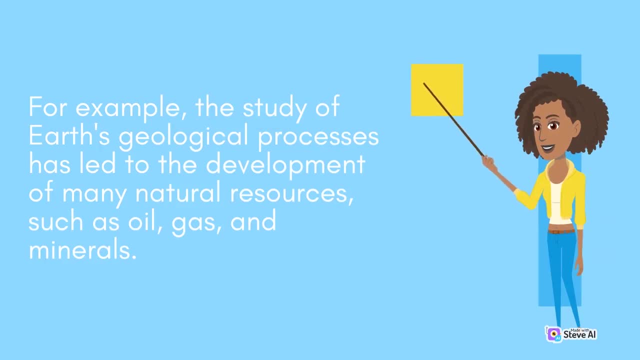 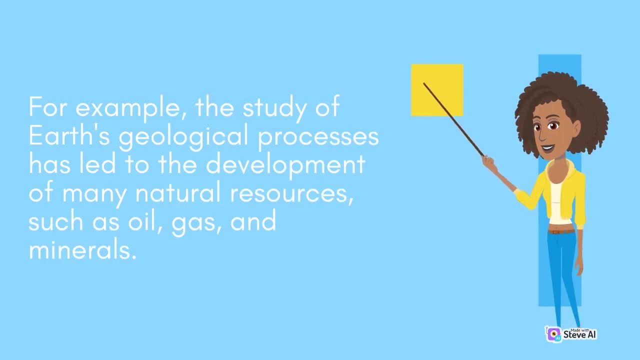 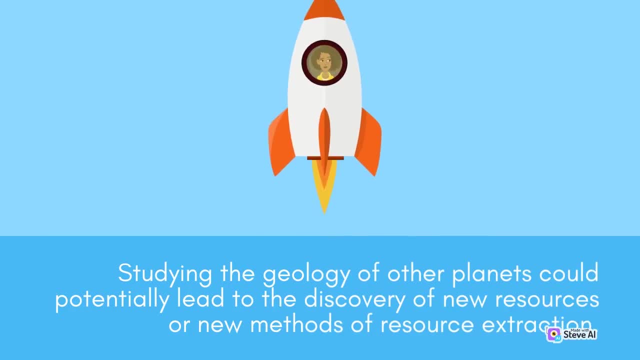 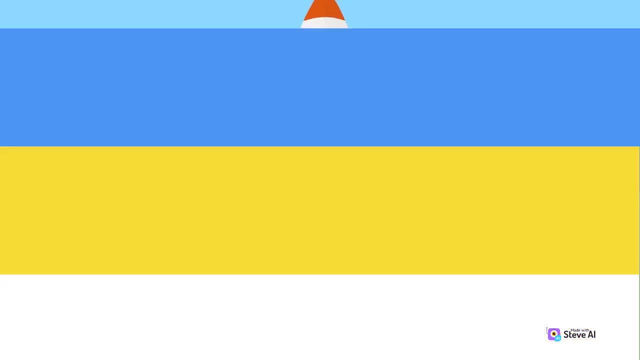 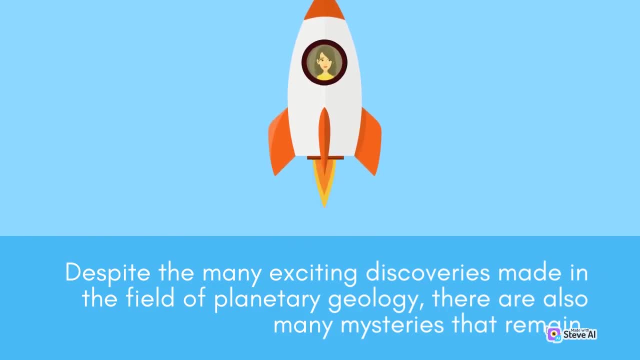 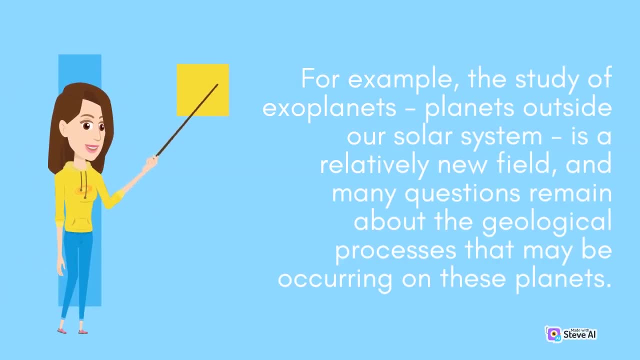 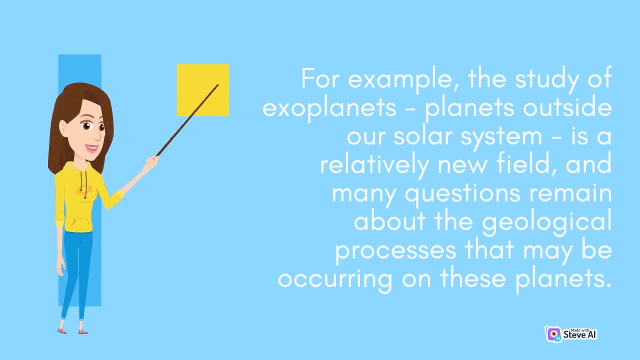 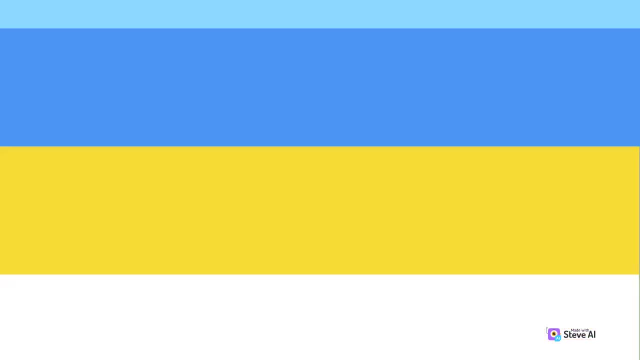 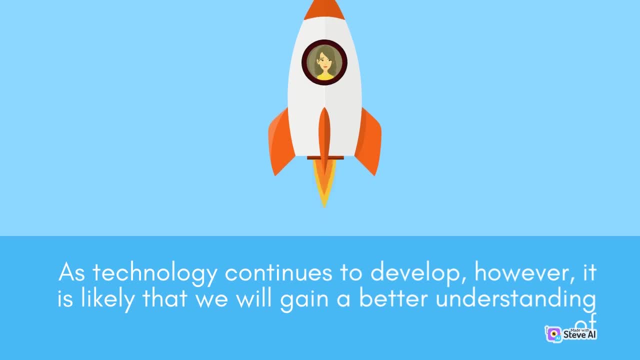 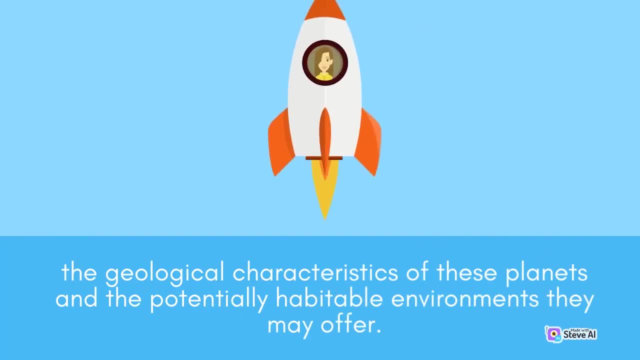 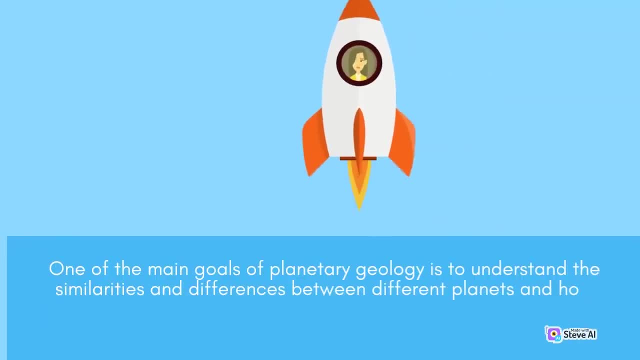 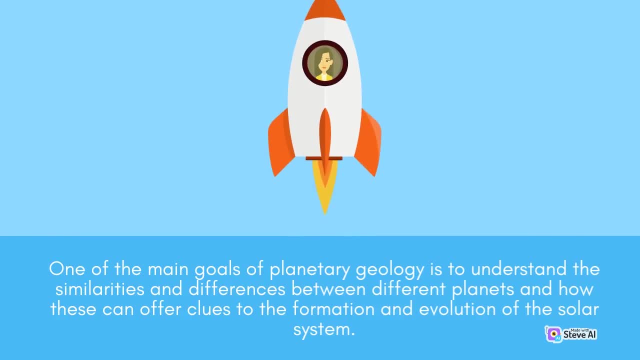 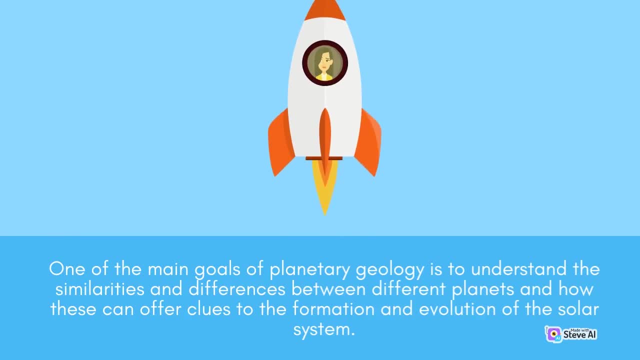 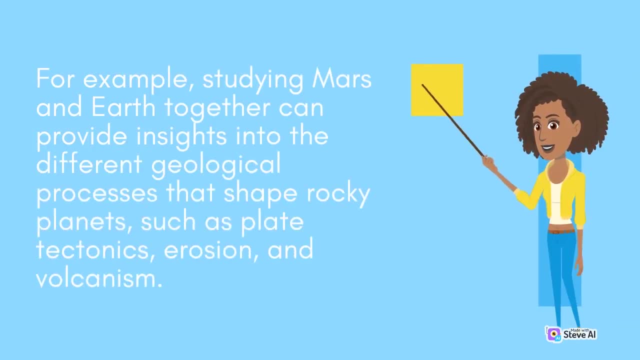 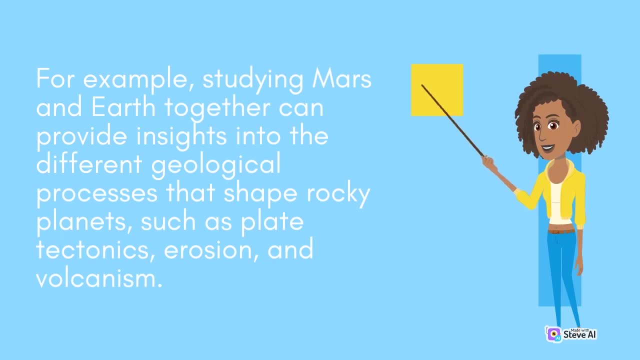 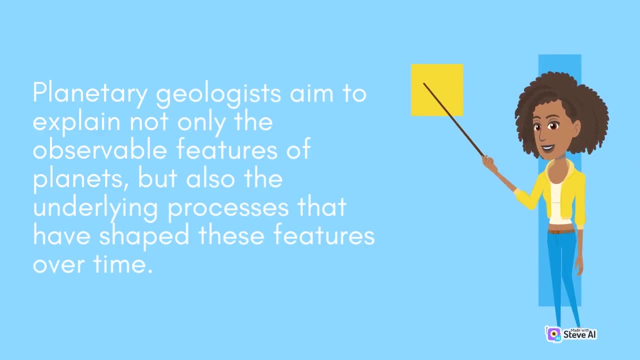 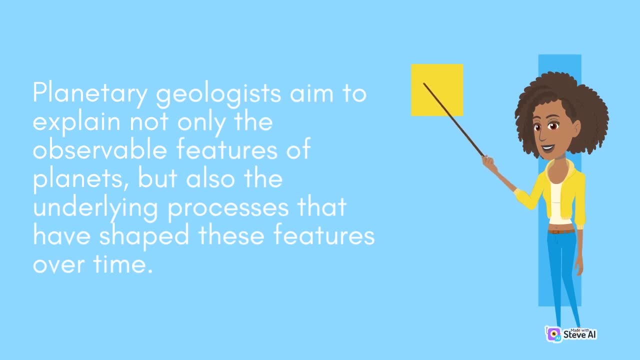 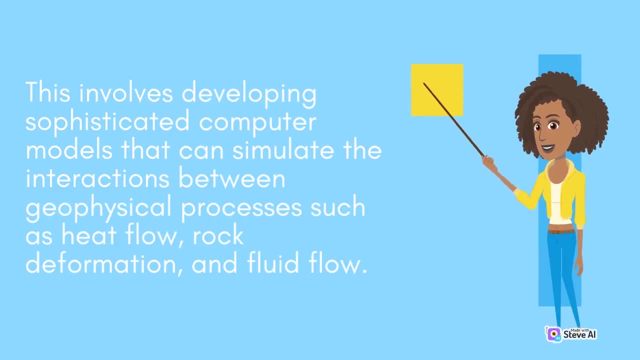 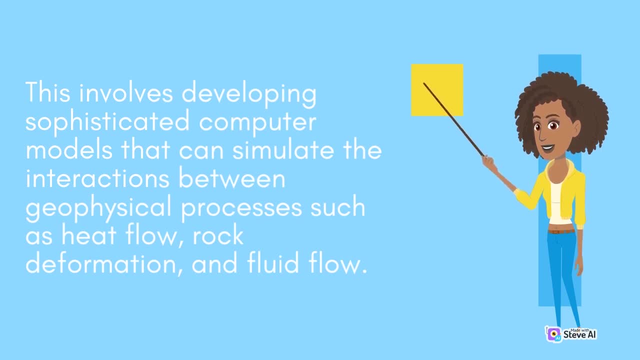 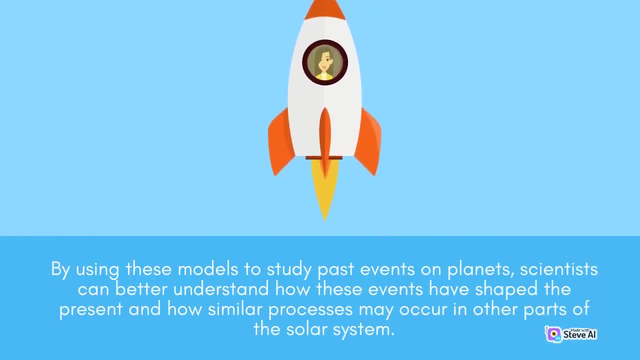 By using these models to study past events on planets, scientists can better understand how these events have shaped the present, and how similar processes may occur and their parts of the solar system. By using these models to study past events on planets, scientists can better understand how these events have shaped the present, and how similar processes may occur and their parts of the solar system. 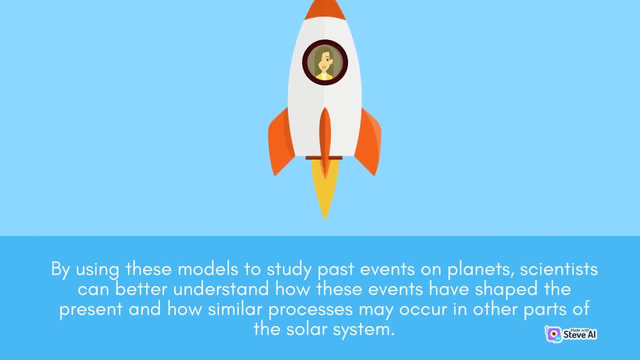 By using these models to study past events on planets, scientists can better understand how these events have shaped the present, and how similar processes may occur and their parts of the solar system. By using these models to study past events on planets, scientists can better understand how these events have shaped the present, and how similar processes may occur and their parts of the solar system. 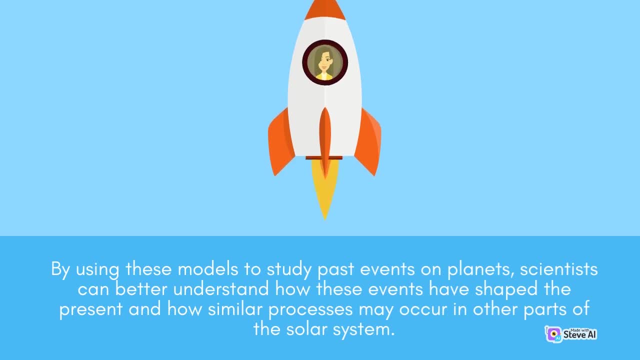 By using these models to study past events on planets, scientists can better understand how these events have shaped the present, and how similar processes may occur and their parts of the solar system. By using these models to study past events on planets, scientists can better understand how these events have shaped the present, and how similar processes may occur and their parts of the solar system. 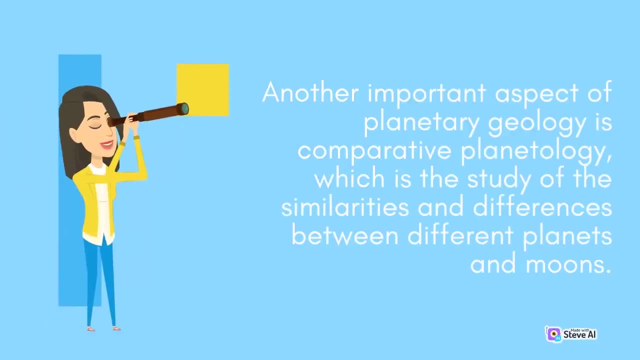 By using these models to study past events on planets, scientists can better understand how these events have shaped the present and how similar processes may occur and their parts of the solar system. Another important aspect of planetary geology is comparative planetology, which is the study of the similarities and differences between different planets and moons. 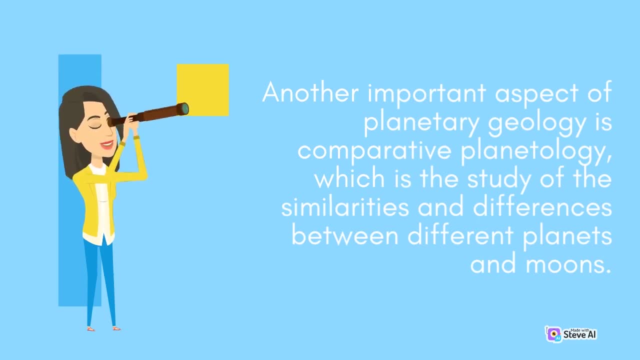 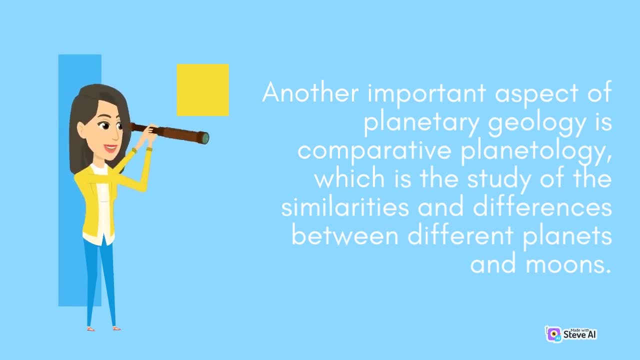 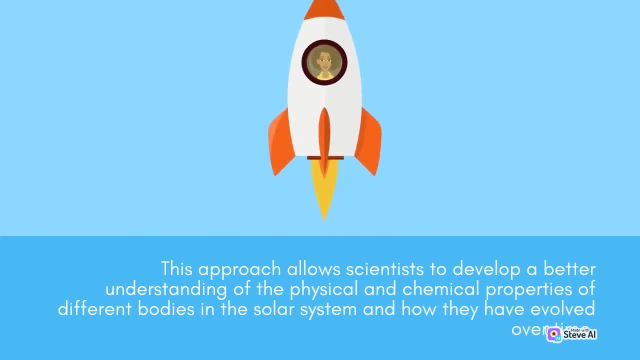 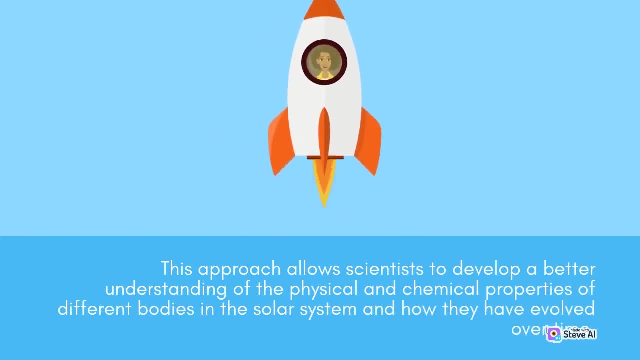 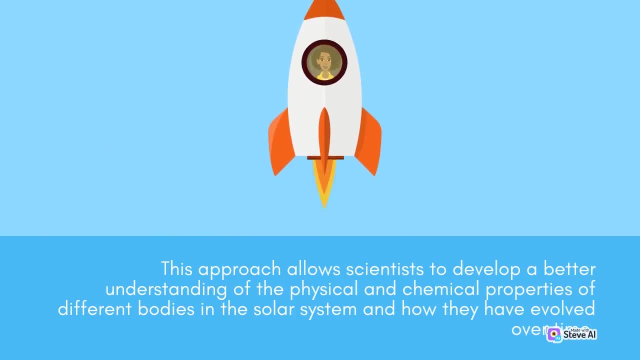 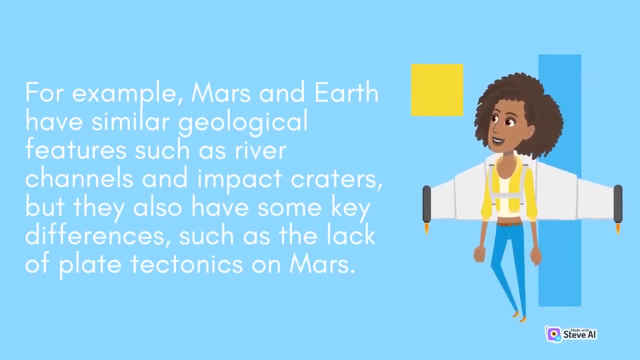 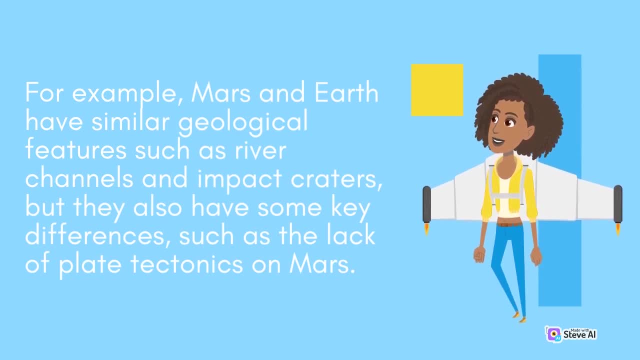 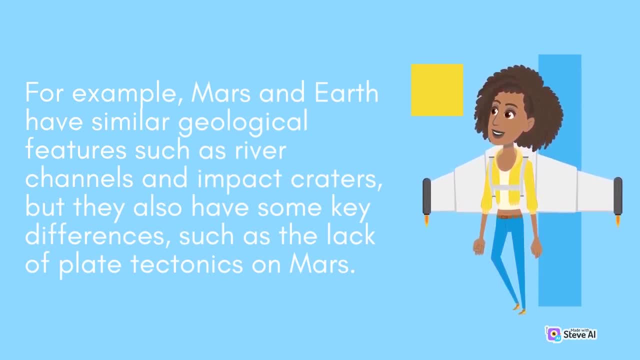 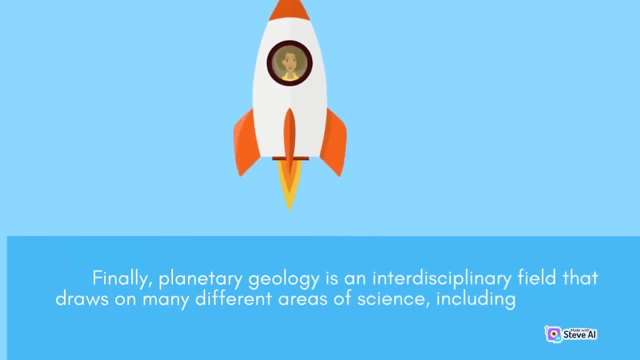 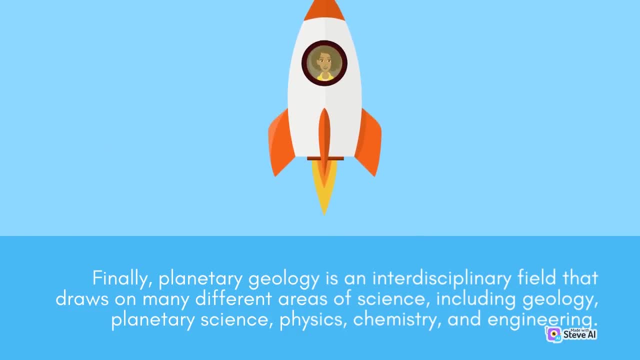 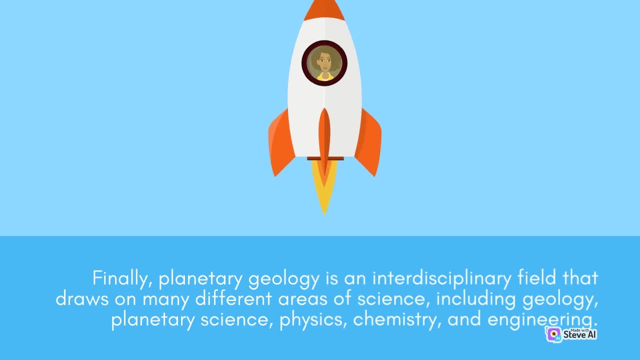 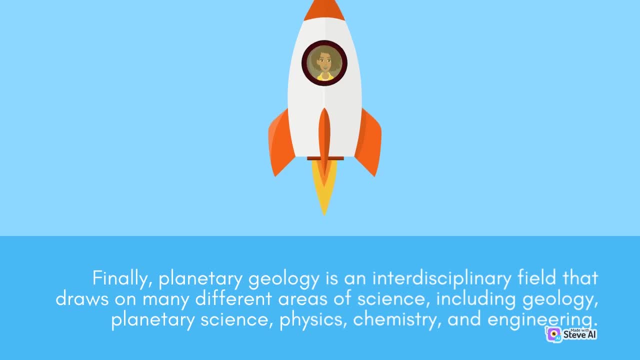 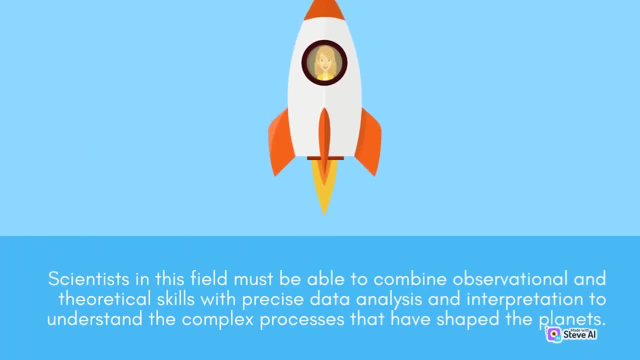 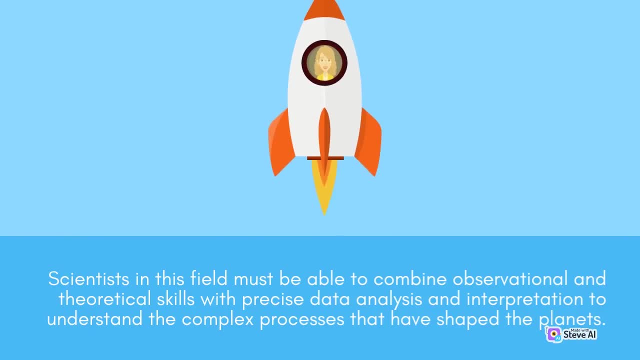 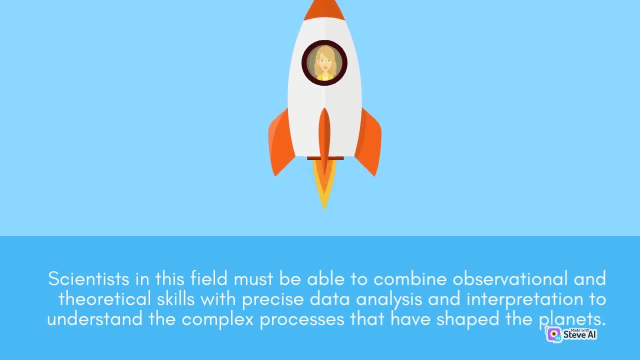 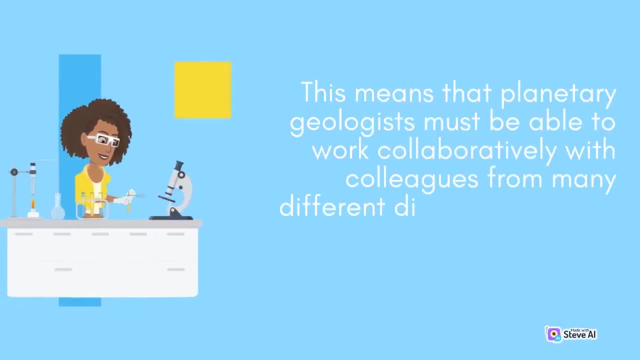 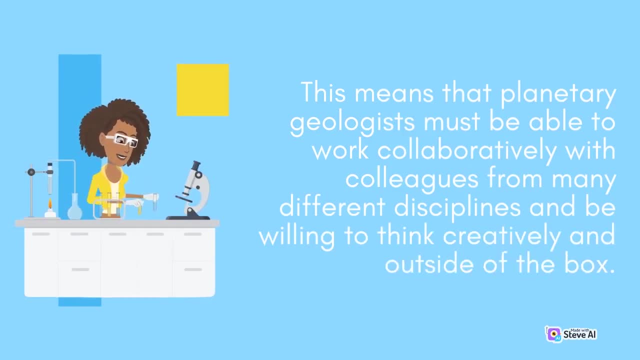 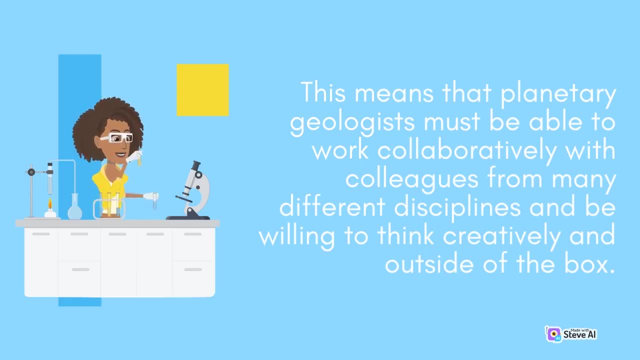 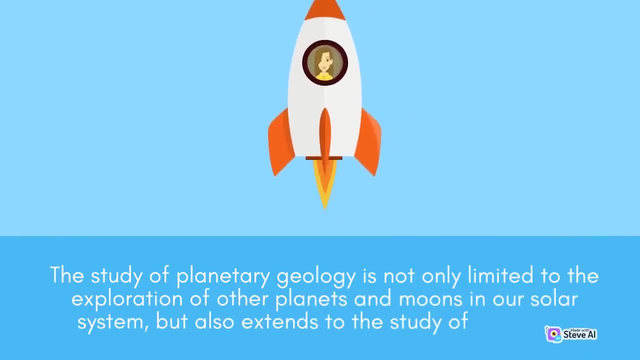 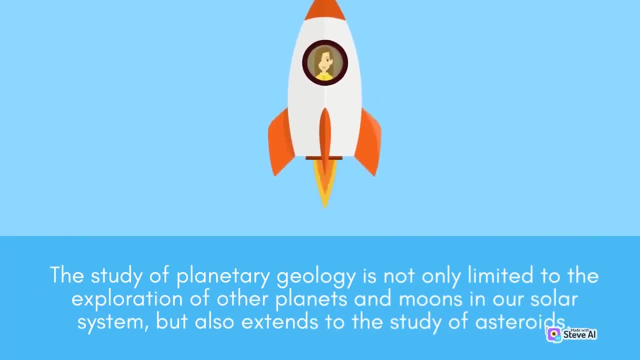 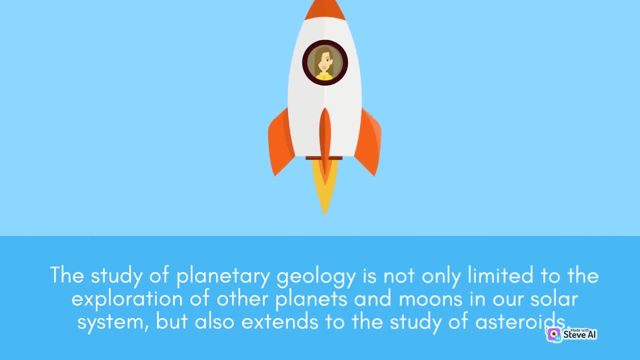 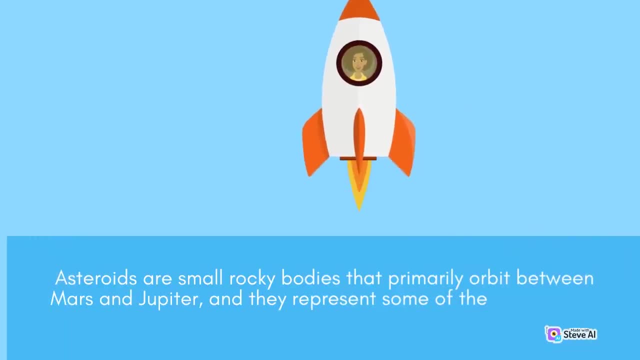 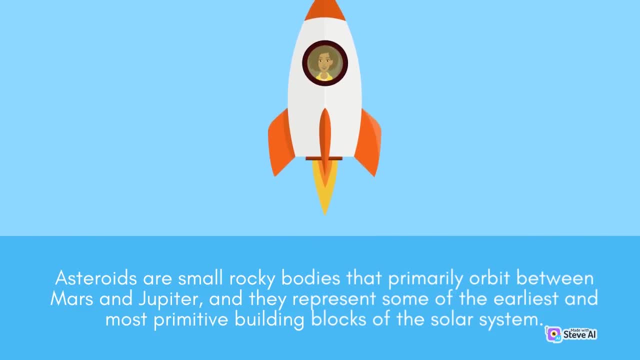 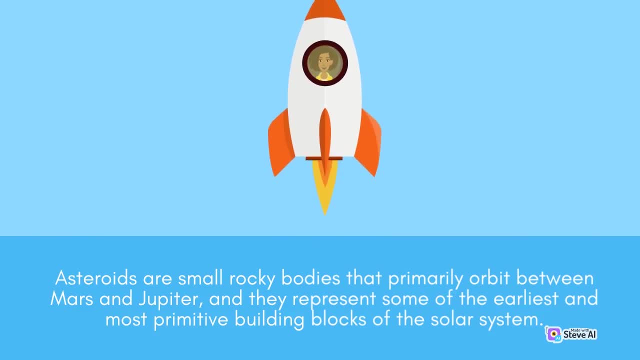 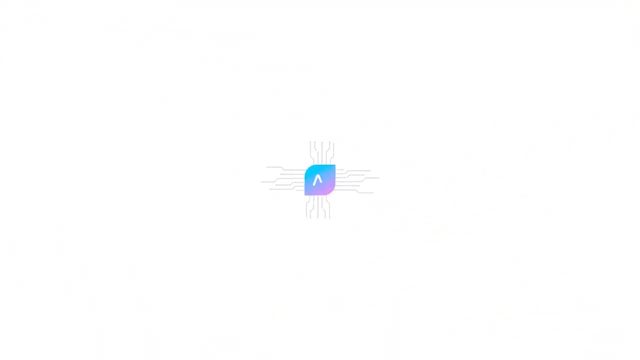 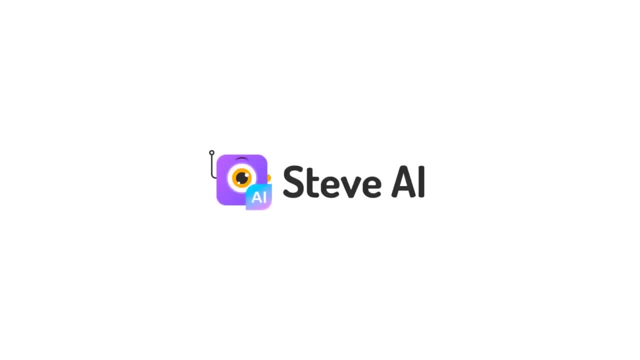 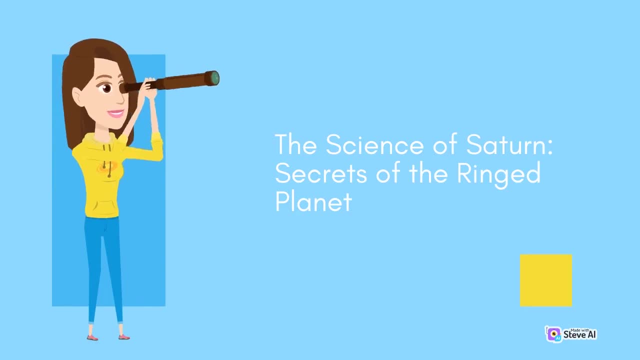 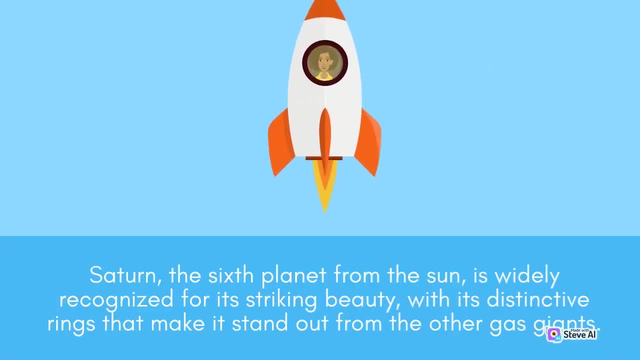 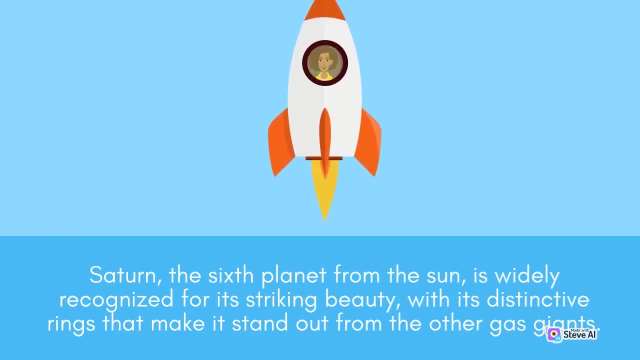 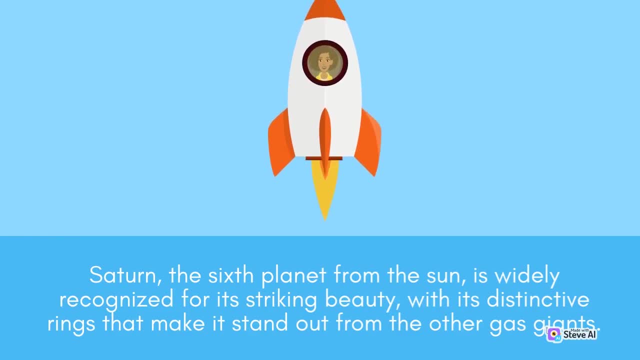 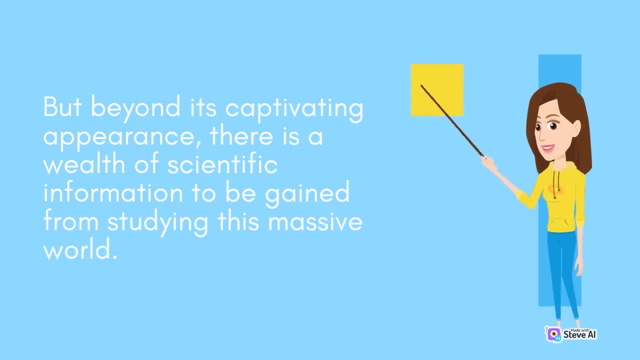 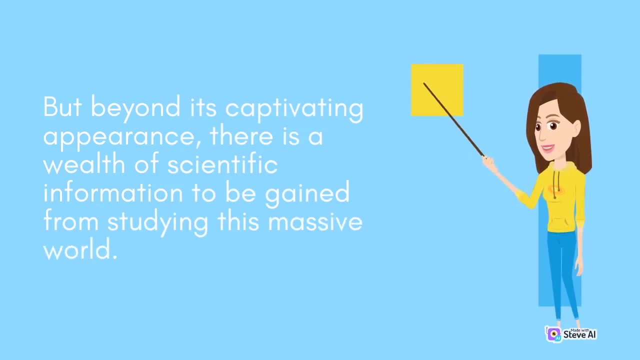 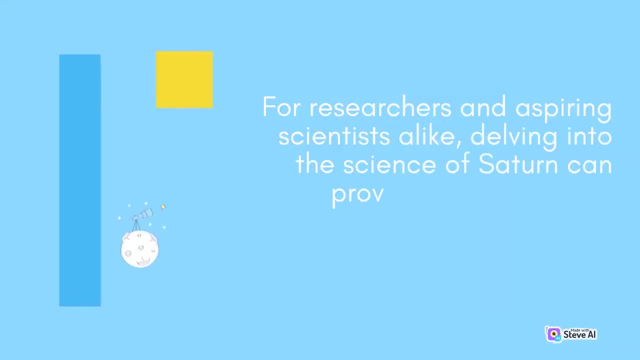 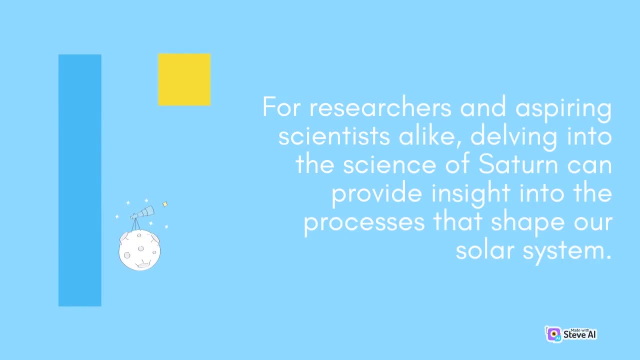 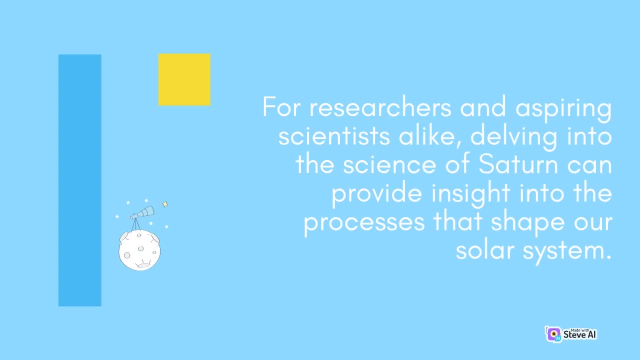 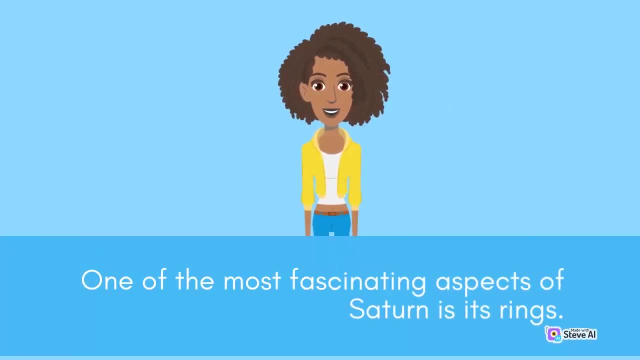 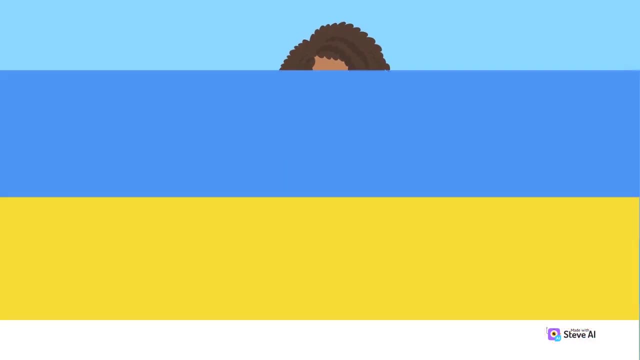 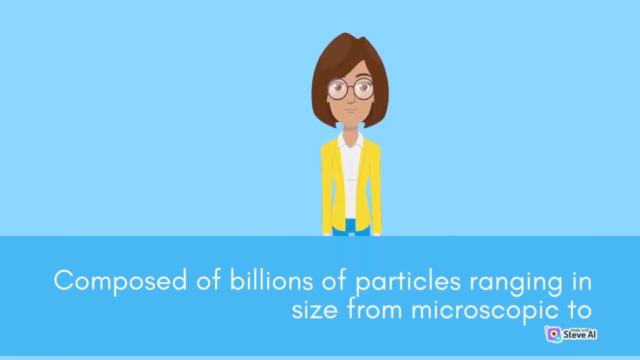 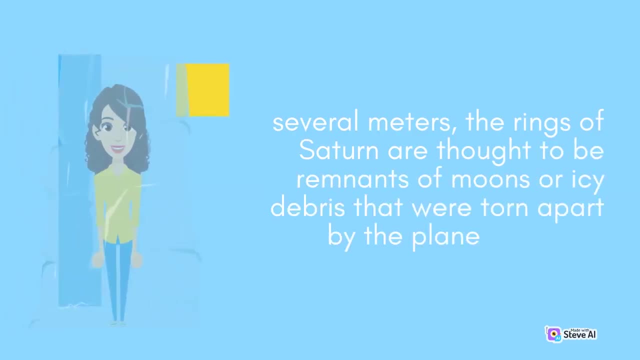 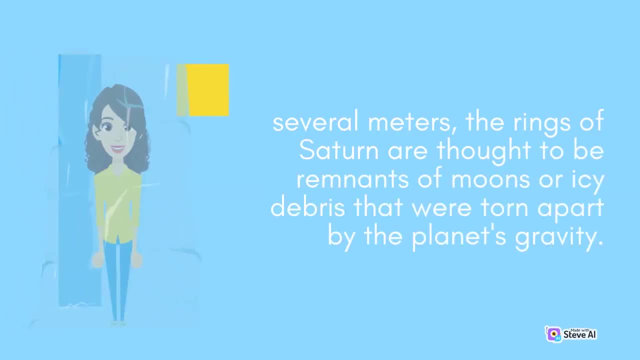 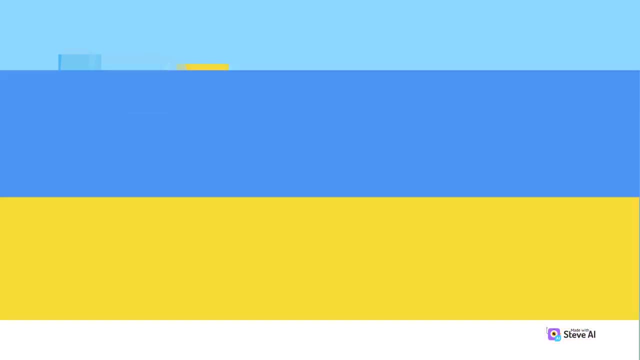 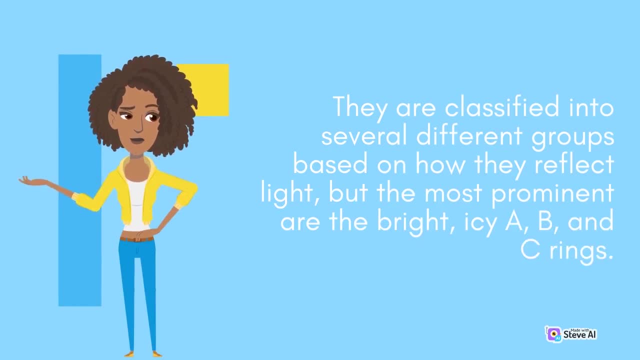 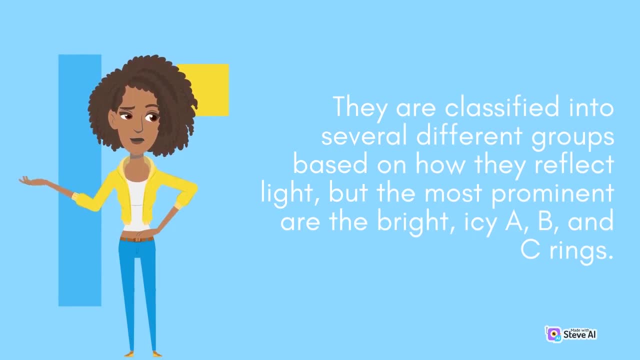 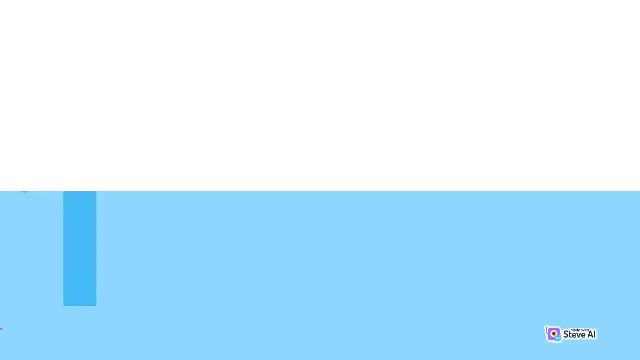 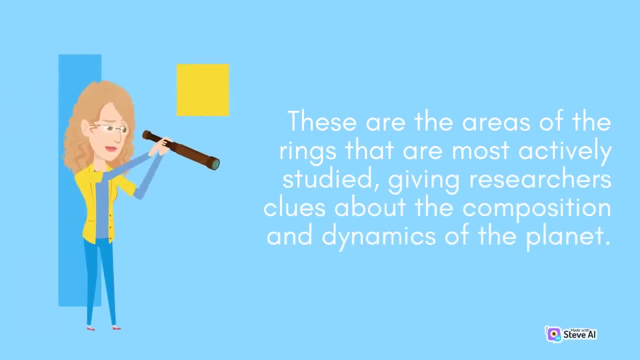 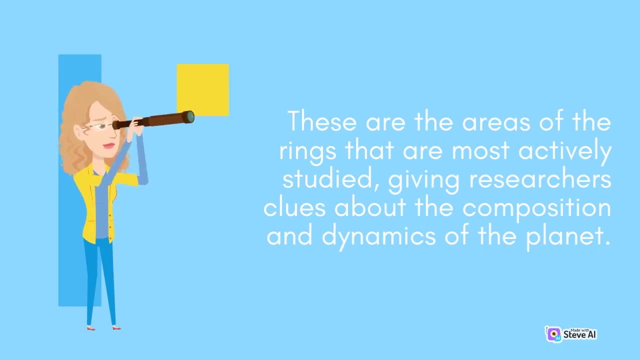 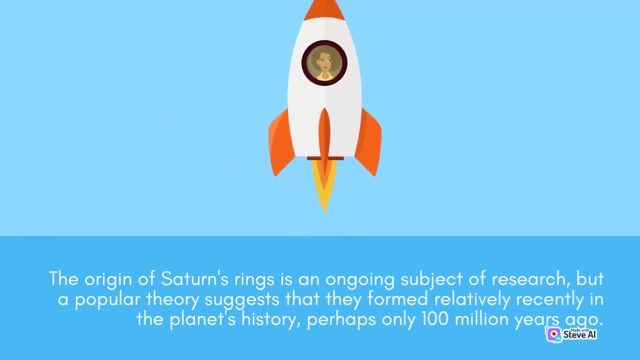 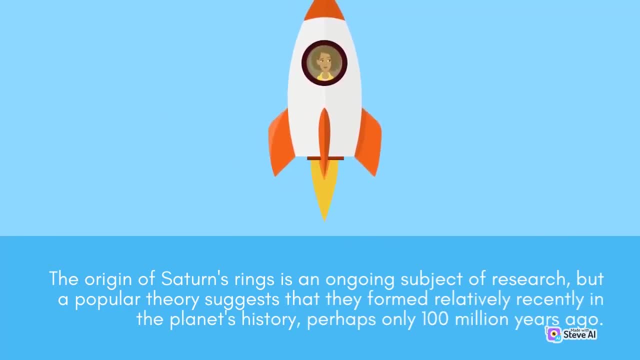 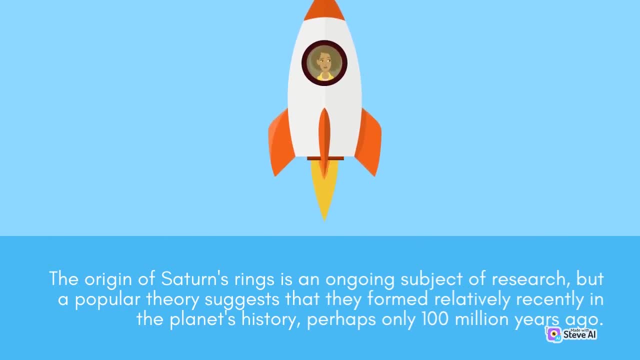 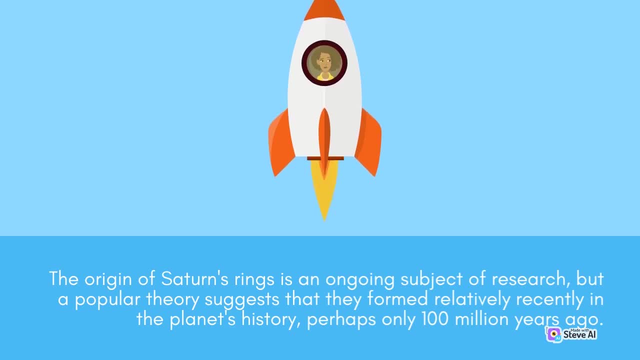 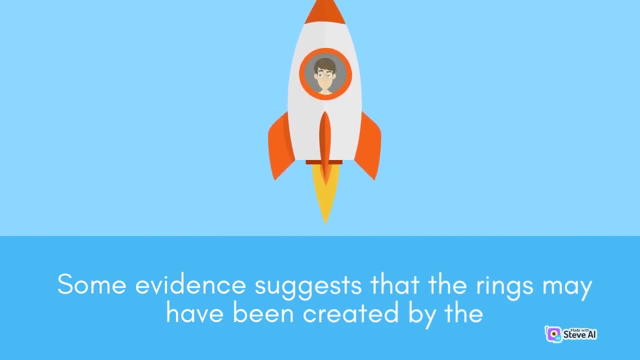 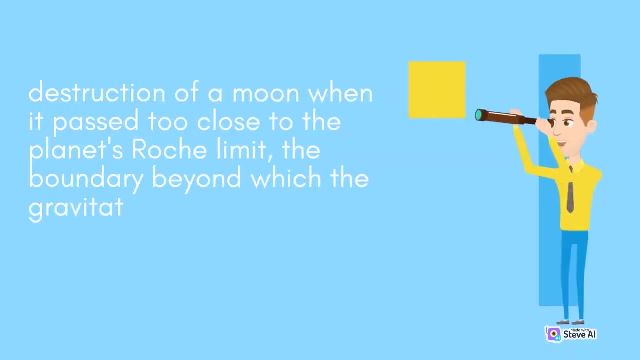 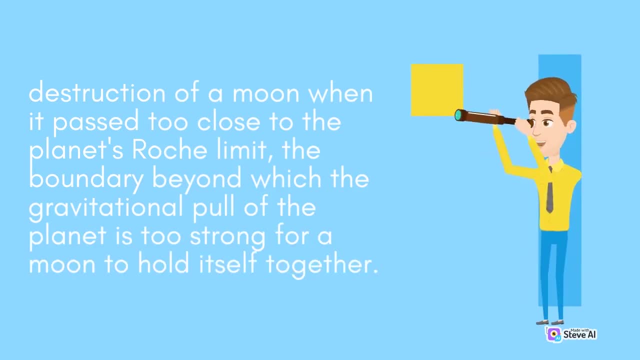 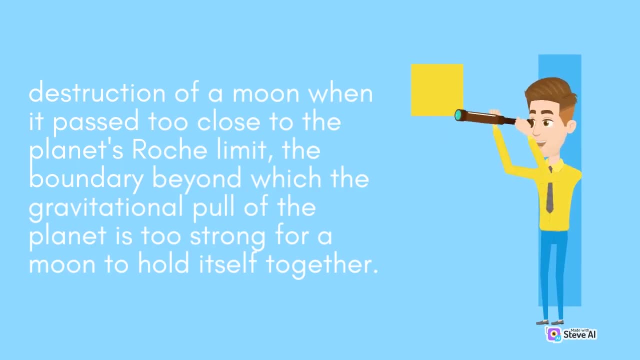 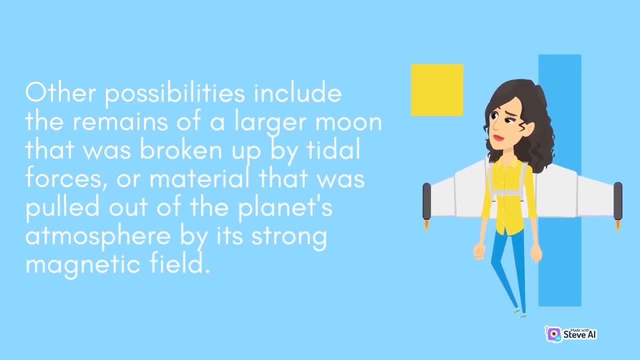 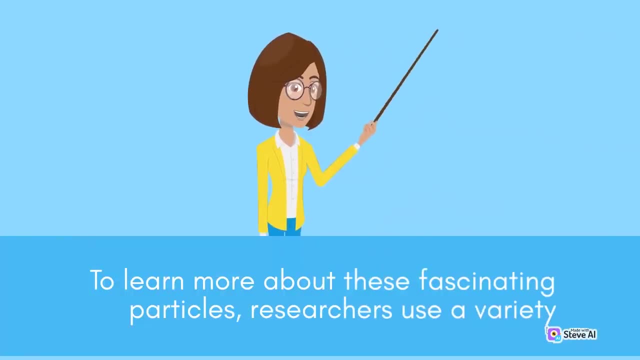 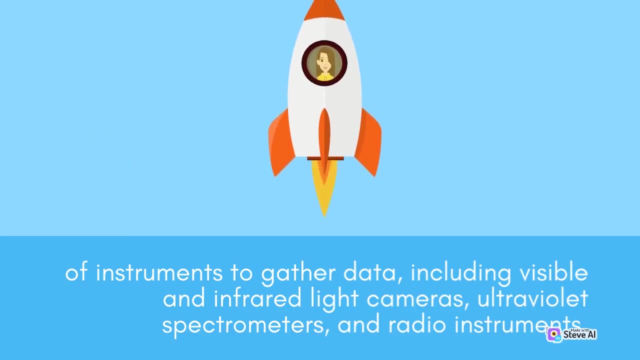 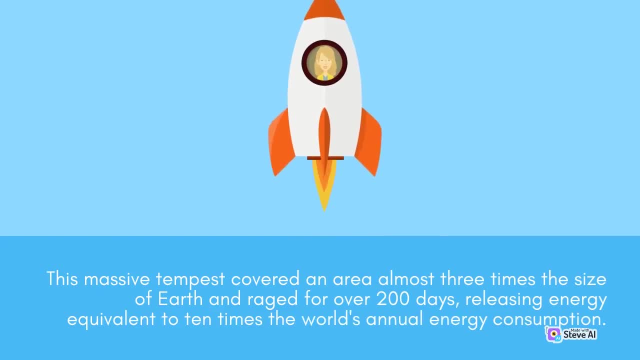 Like Jupiter, its upper atmosphere is dominated by hydrogen and helium, with trace amounts of methane, ammonia and water almost three times the size of Earth and raged for over 200 days, releasing energy equivalent to 10 times the world's annual energy consumption. 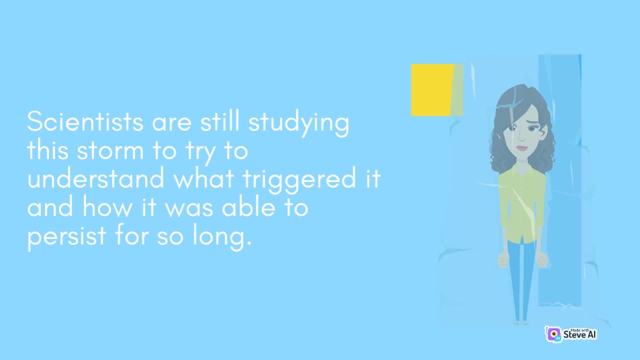 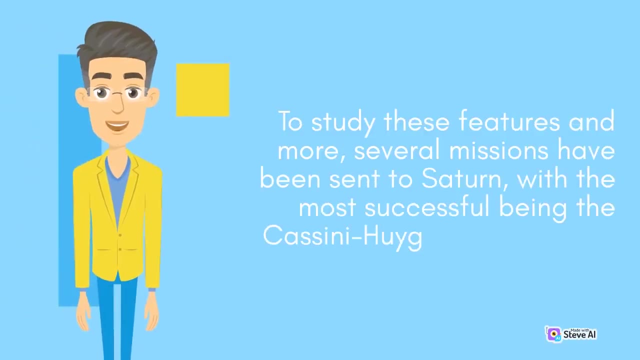 Scientists are still studying this storm to try to understand what triggered it and how it was able to persist for so long. To study these features and more, several missions have been sent to Saturn, with the most successful being the Cassini-Huygens spacecraft. 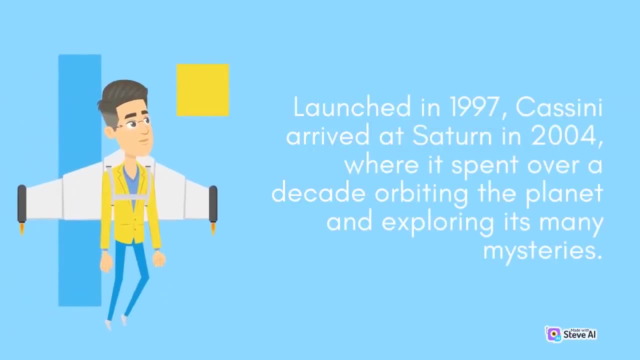 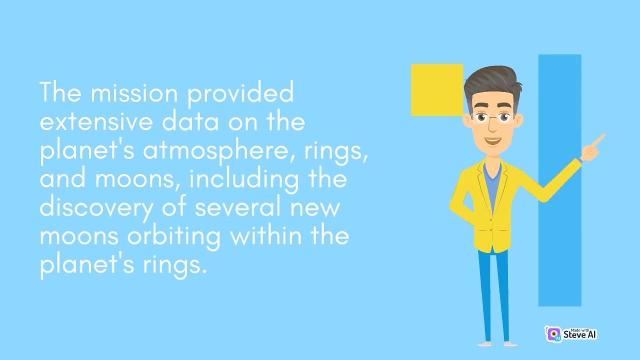 Launched in 1997, Cassini arrived at Saturn in 2004,, where it spent over a decade orbiting the planet and exploring its many mysteries. The mission provided extensive data on the planet's atmosphere, rings and moons, including the discovery of several new moons orbiting within the planet's rings. 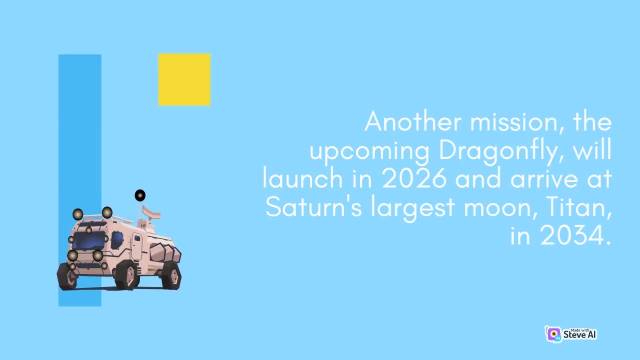 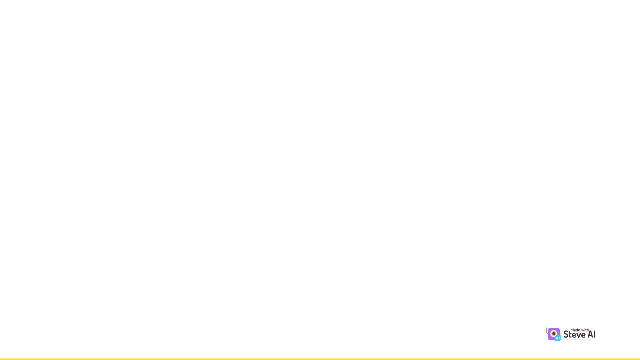 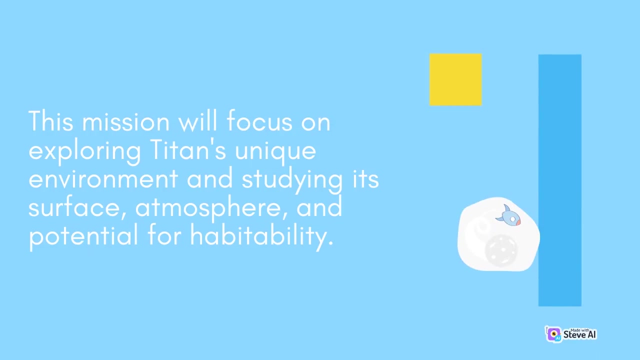 Another mission, the upcoming Dragonfly, will launch in 2026 and arrive at Saturn's largest lunar orbit, Titan, in 2034. This mission will focus on exploring Titan's unique environment and studying its surface atmosphere and potential for habitability. 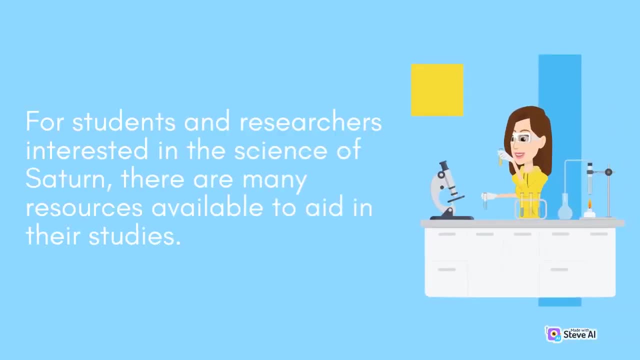 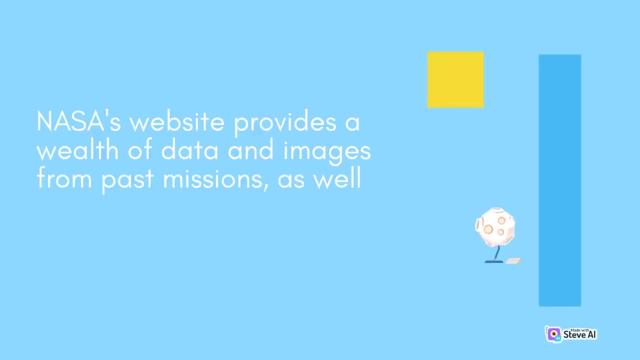 For students and researchers interested in the science of Saturn, there are many resources available to aid in their studies. NASA's website provides a wealth of data and images from past missions, as well as news on the moon. NASA's website provides a wealth of data and images from past missions. 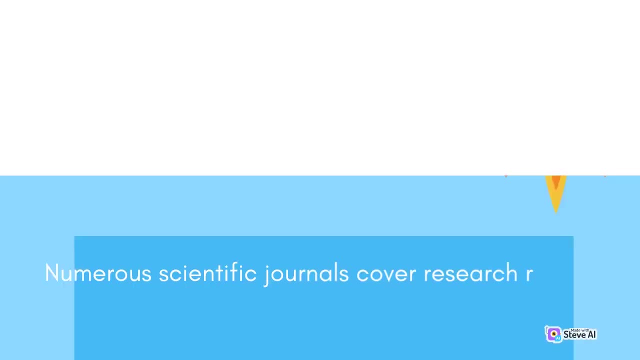 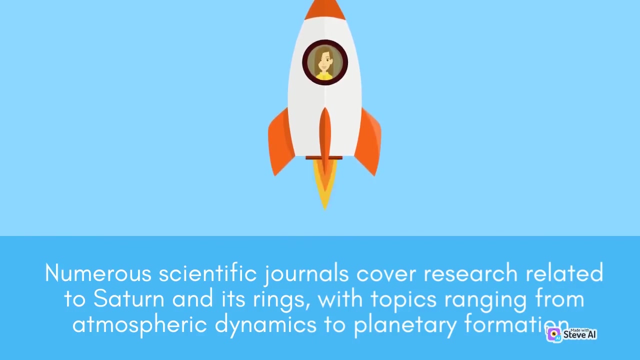 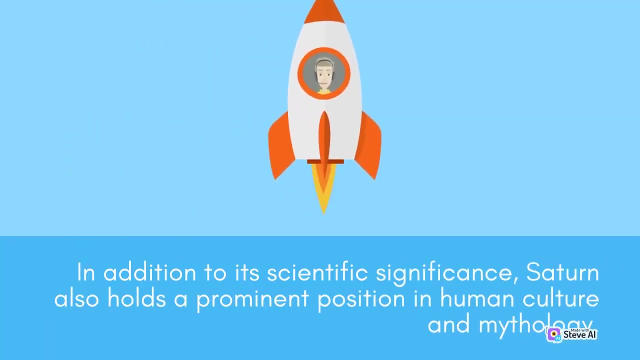 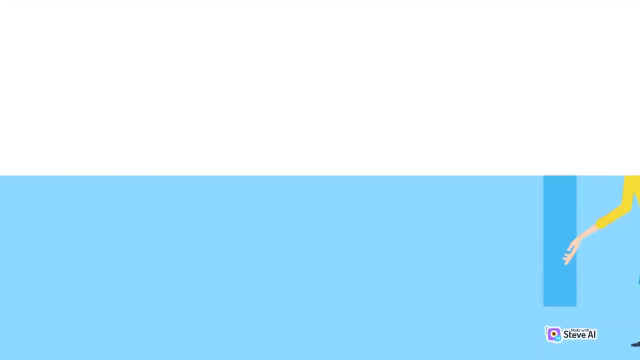 as well as news on the moon. Numerous scientific journals cover research related to Saturn and its rings, with topics ranging from atmospheric dynamics to planetary formation. In addition to its scientific significance, Saturn also holds a prominent position in human culture and mythology, Named after the Roman god of agriculture. 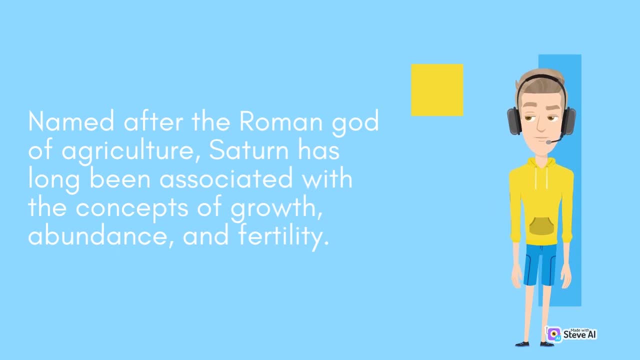 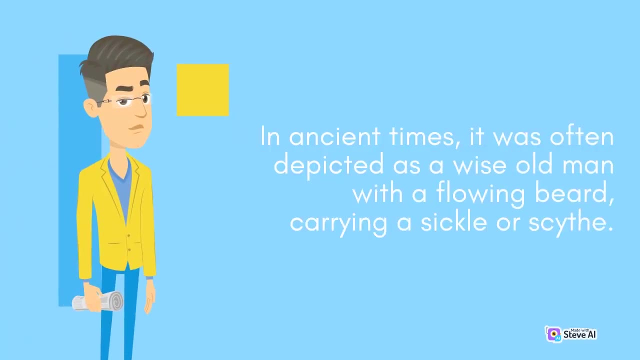 Saturn has long been a famous person for its scientific and archaeological work, associated with the concepts of growth, abundance and fertility. In ancient times, it was often depicted as a wise old man with a flowing beard, carrying a sickle or scythe. 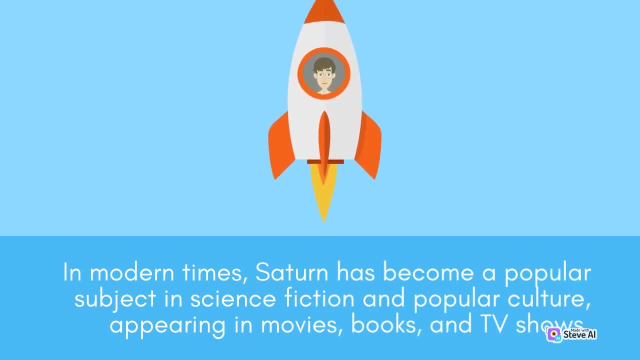 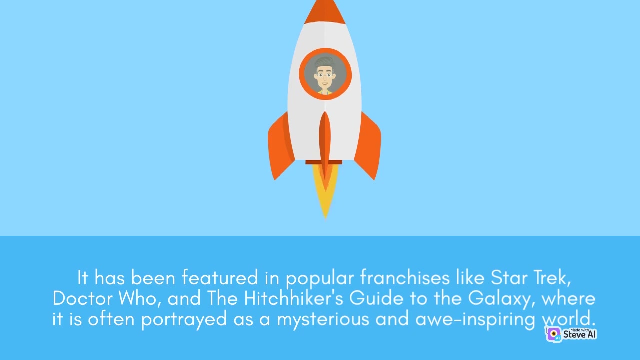 In modern times, Saturn has become a popular subject in science fiction and popular culture, appearing in movies, books and TV shows. It has been featured in popular franchises like Star Trek, Doctor Who and The Hitchhiker's Guide to the Galaxy, where it is often portrayed as a mysterious and awe-inspiring world. 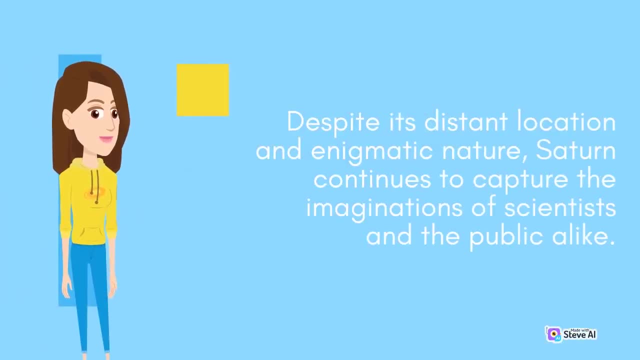 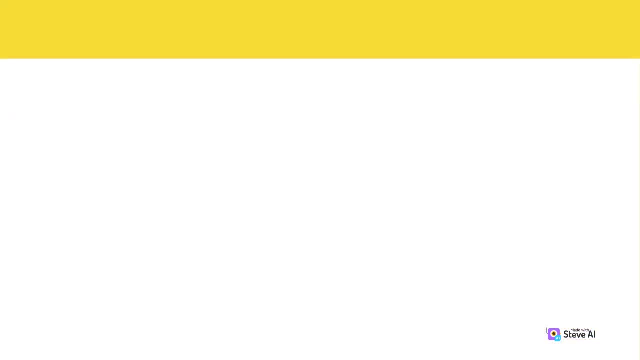 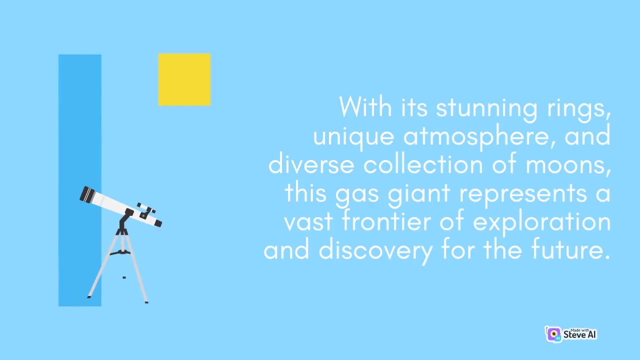 Despite its distant location and enigmatic nature, Saturn continues to capture the imaginations of scientists and the public alike. With its stunning rings, unique atmosphere and diverse collection of movies, this gas giant represents a vast frontier of exploration and discovery for the future. 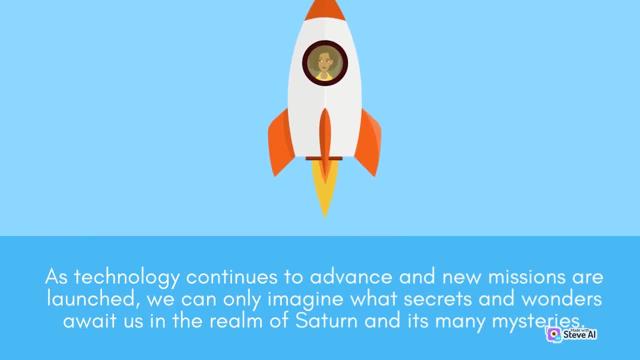 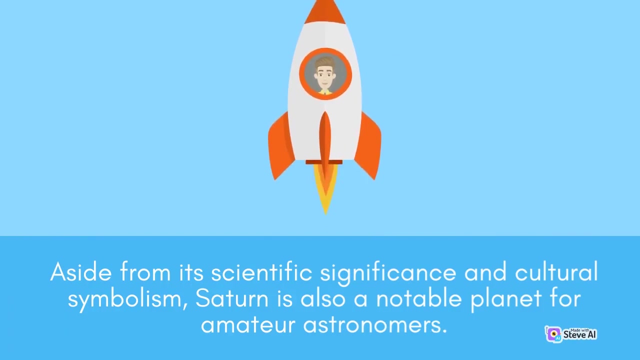 As technology continues to advance and new missions are launched, we can only imagine what secrets and wonders await us in the realm of Saturn and its many mysteries. Aside from its scientific significance and cultural symbolism, Saturn is also a notable planet for amateur astronomers- NASA. 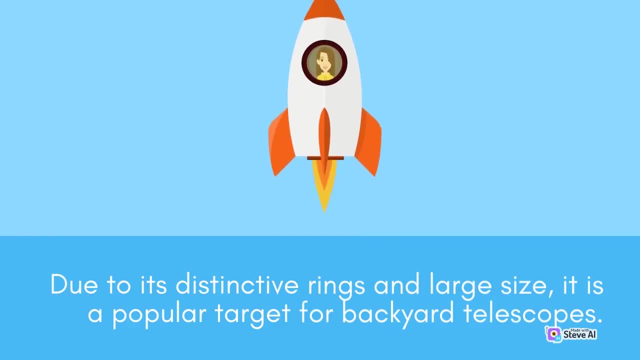 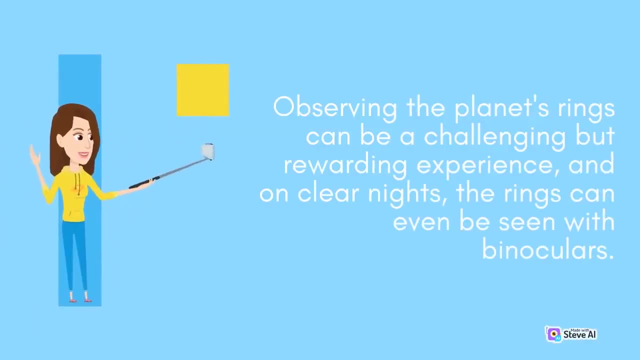 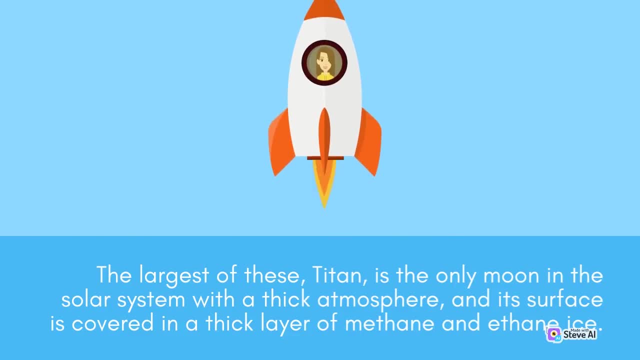 The largest of these, Titan, is the only moon in the solar system, solar system with a thick atmosphere, and its surface is covered in a thick layer of methane and ethane ice. Other notable moons include Enceladus, which has geysers of water vapor. 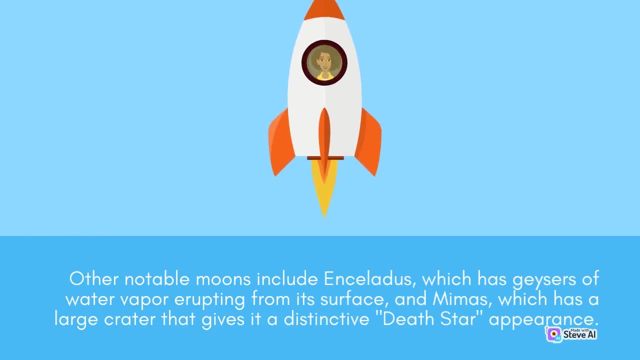 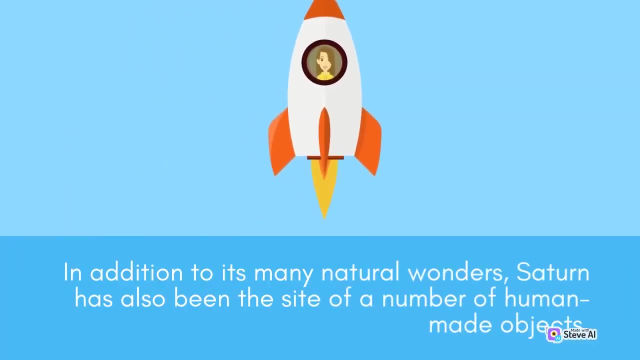 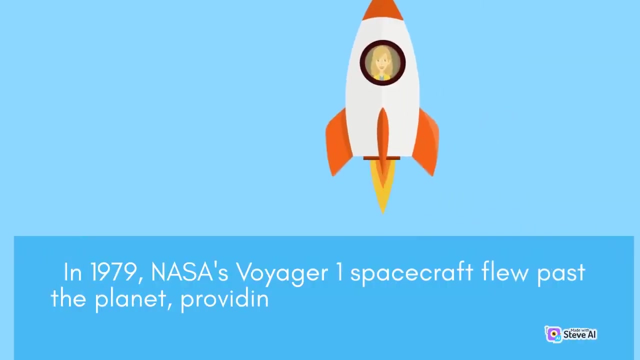 erupting from its surface, and Mimas, which has a large crater that gives it a distinctive Death Star appearance. In addition to its many natural wonders, Saturn has also been the site of a number of human-made objects. In 1979, NASA's Voyager 1 spacecraft flew past the planet. 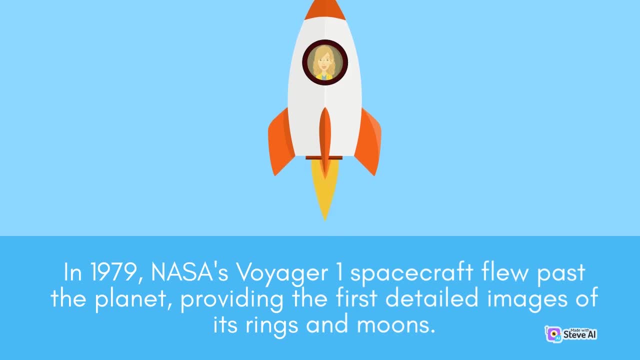 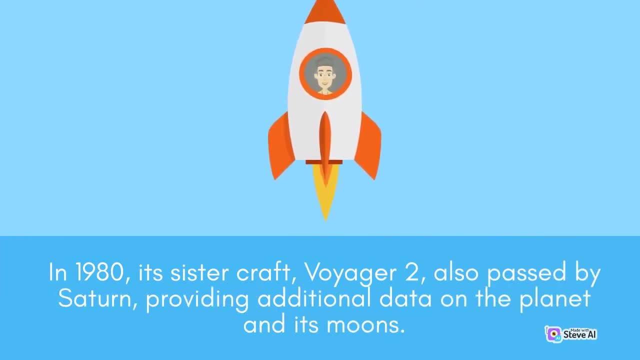 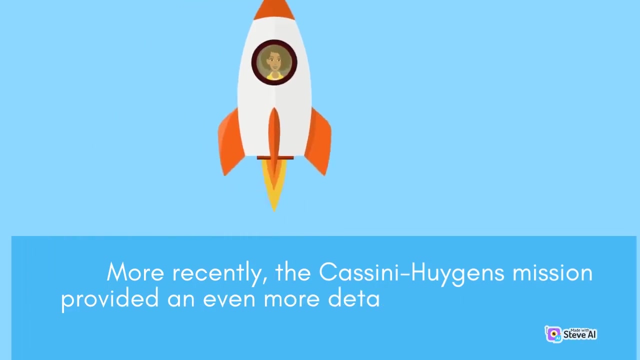 providing the first detailed images of its rings and moons. In 1980, its sister craft, Voyager 2,, also passed by Saturn, providing additional data on the planet and its moons. More recently, the Cassini-Huygens mission provided an. 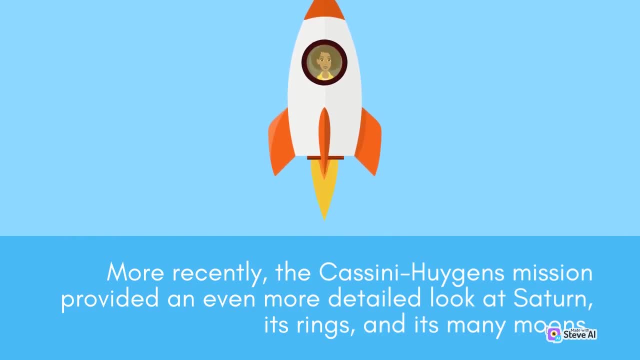 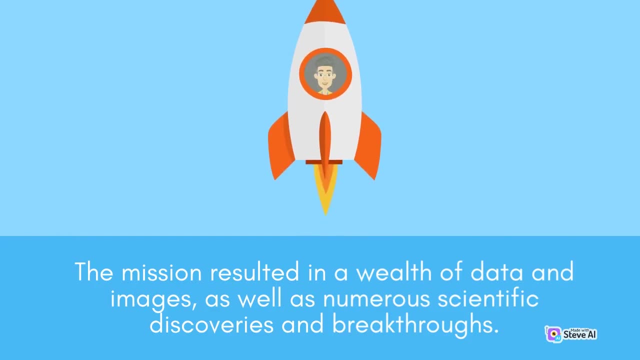 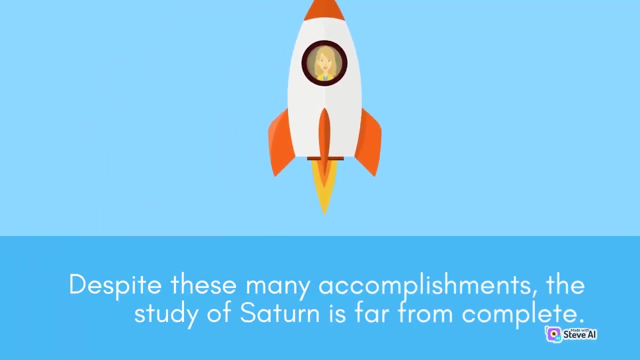 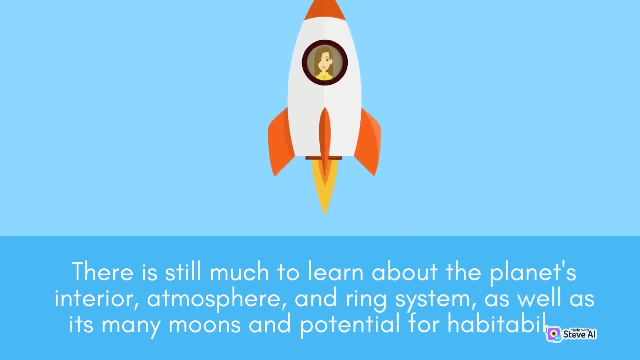 even more detailed image of the planet's rings and moons. The mission resulted in a wealth of data and images, as well as numerous scientific discoveries and breakthroughs. Despite these many accomplishments, the study of Saturn is far from complete. There is still much to learn about the planet's interior atmosphere. 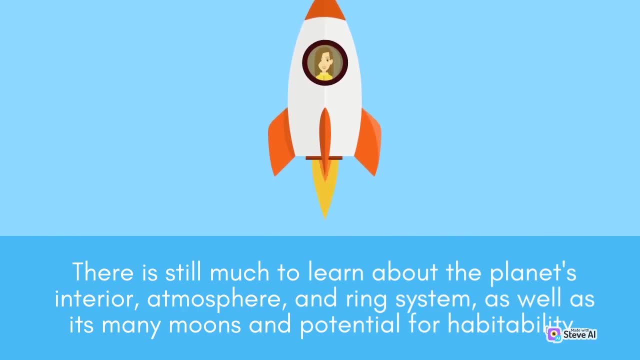 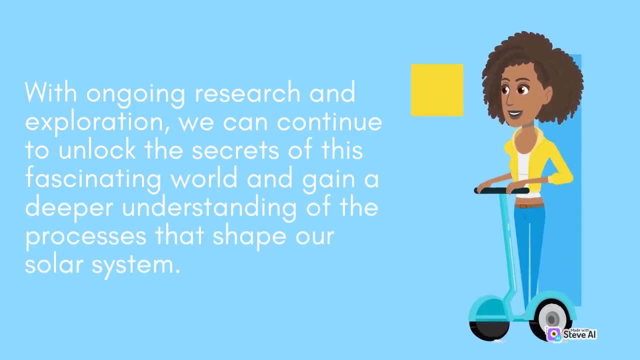 and ring system, as well as its many moons and potential for habitability. With ongoing research and exploration, we can continue to unlock the secrets of this fascinating world and gain a deeper understanding of the processes that shape our solar system. Saturn's moons are another intriguing aspect of this gas giant. 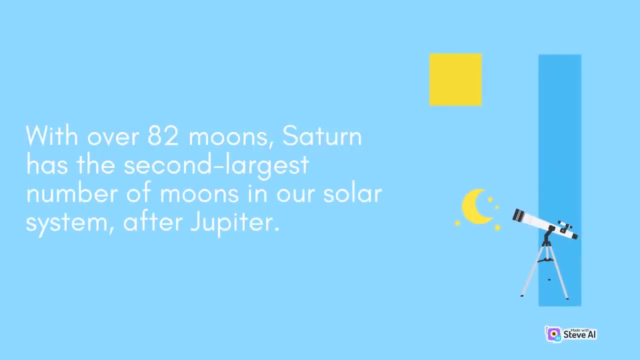 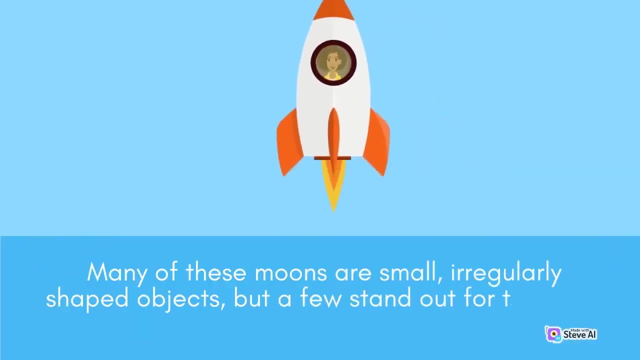 With over 82 moons, Saturn has the second largest number of moons in our solar system after Jupiter. Many of these moons are small, irregularly shaped objects, but a few stand out for their size and unique features. One of the most interesting moons of Saturn is Enceladus. 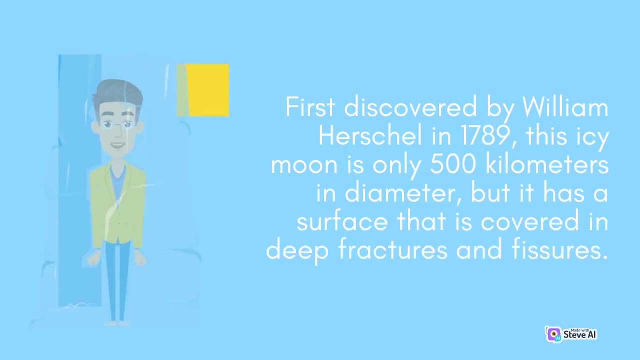 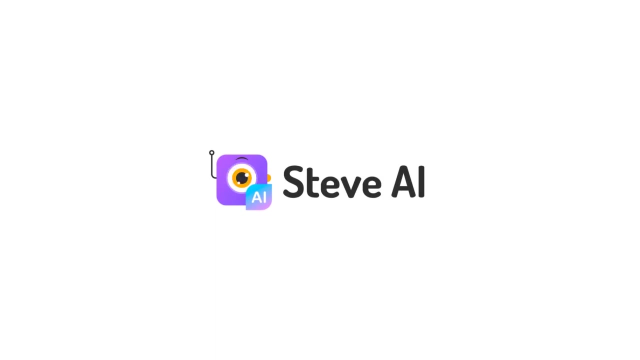 First discovered by William Herschel in 1789,. this icy moon is only 500 kilometers in diameter, but it has a surface that is covered in deep fractures and fissures. It is known to be an extreme looking star, Exploring the early universe through cosmic microwave background radiation. 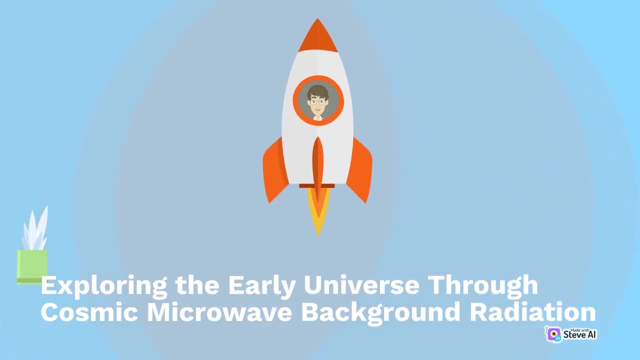 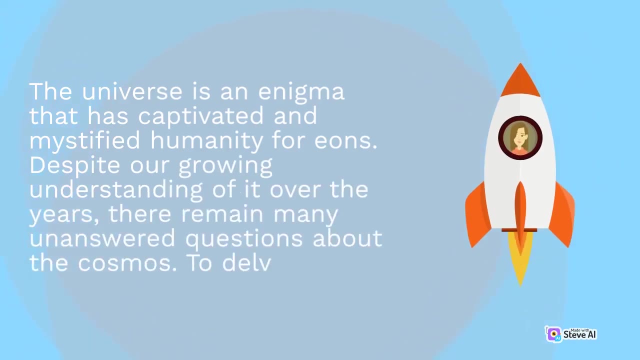 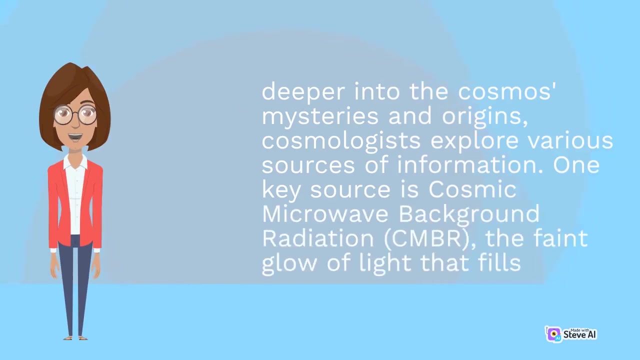 Exploring the early universe through cosmic microwave background radiation. The universe is an enigma that has captivated and mystified humanity for eons. Despite our growing understanding of it over the years, there remain many unanswered questions about the cosmos. To delve Deeper into the cosmos' mysteries and origins, cosmologists explore various sources of information. 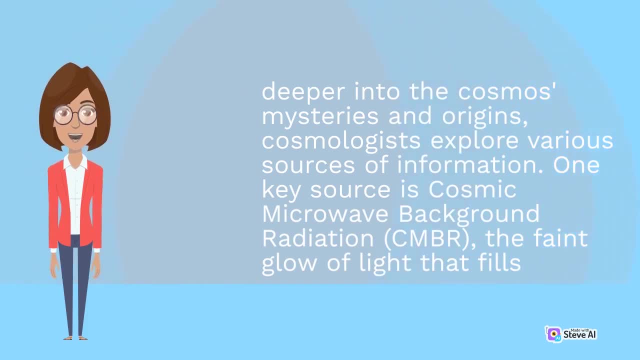 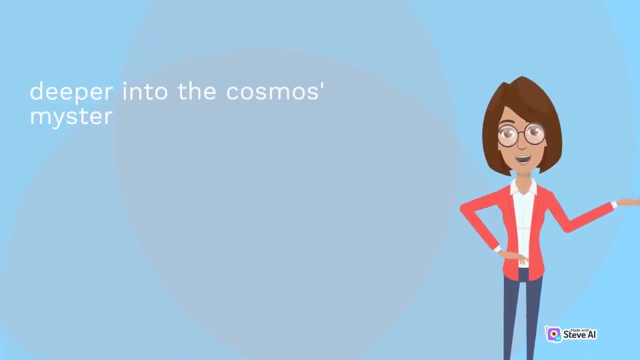 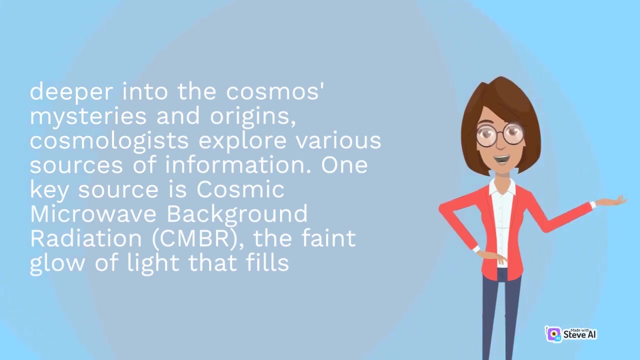 One key source is Cosmic Microwave Background Radiation- CMBR- the faint glow of light that fills Deeper into the cosmos' mysteries and origins. cosmologists explore various sources of information. One key source is Cosmic Microwave Background Radiation- CMBR- the faint glow of light that fills 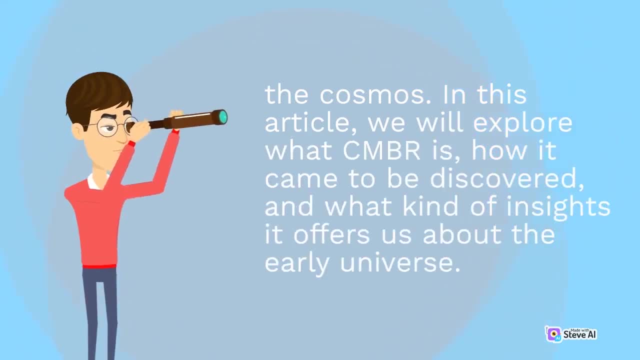 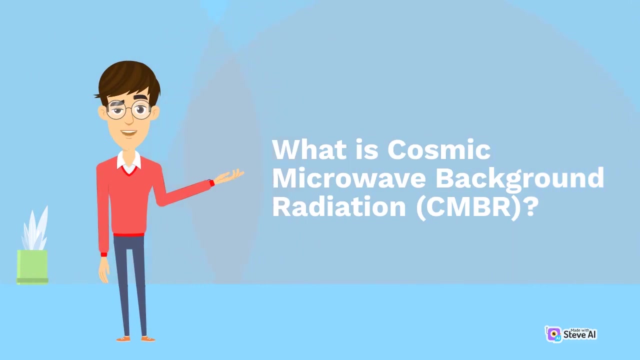 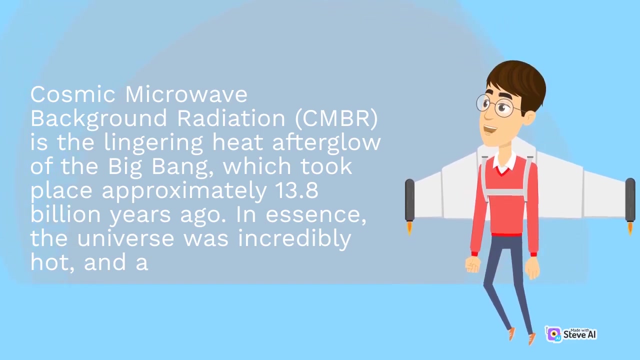 The Cosmos. In this article, we will explore what CMBR is, how it came to be discovered and what kind of insights it offers us about the early universe. What is Cosmic Microwave Background Radiation- CMBR? Cosmic Microwave Background Radiation. Cosmic Microwave Background Radiation- CMBR is the lingering heat afterglow of the Big Bang, which took place approximately 13.8 billion years ago. 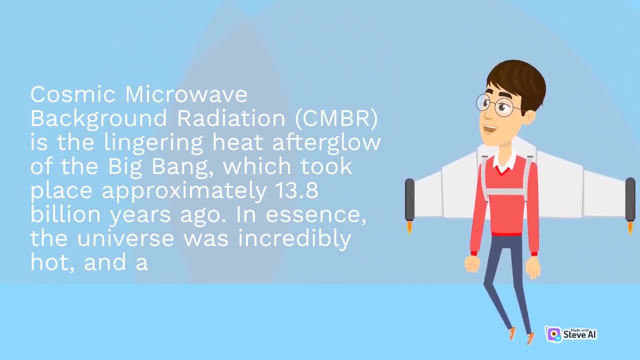 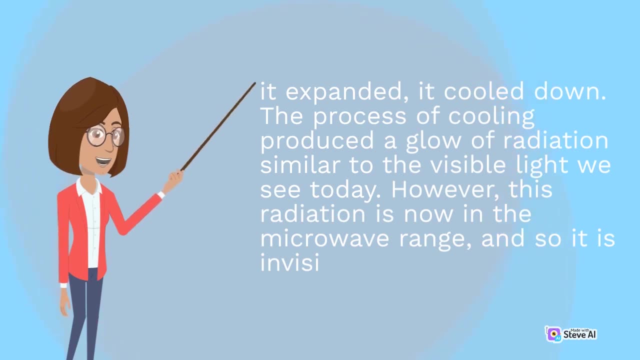 In essence, the universe was incredibly hot, and a It expanded, it cooled down. The process of cooling produced a glow of radiation similar to the visible light we see today. However, this radiation is now in the microwave range, and so it isn't busy. 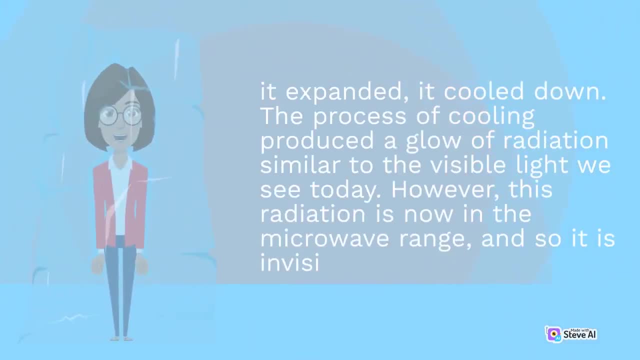 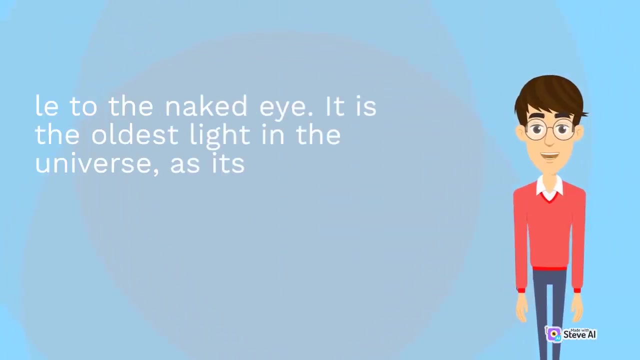 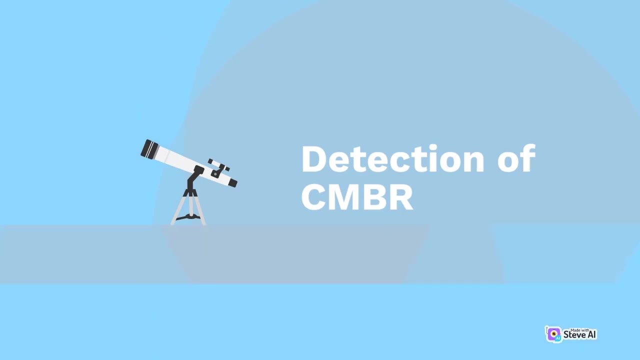 Led to the naked eye. It is the oldest light in the universe, as its origin traces back to about 380,000 after the Big Bang. Detection of CMBR. Detection of CMBR. The detection of CMBR is considered one of the most significant accomplishments in 20th-century. 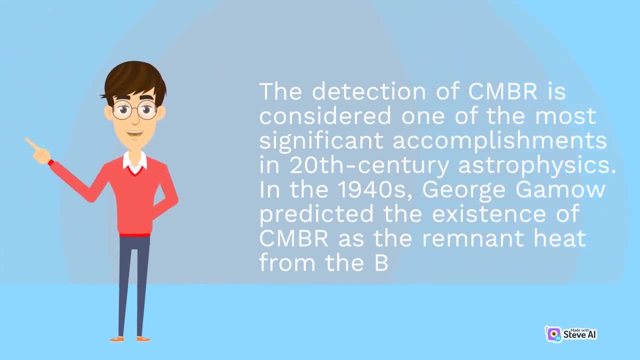 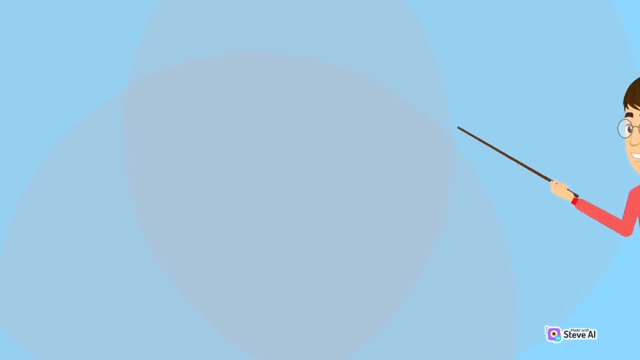 astrophysics. In the 1940s, George Gamow predicted the existence of CMBR as the remnant heat from the B? Gee-bang. In the early 1960s, Robert Wilson and Arno Penzias discovered CMBR through their use. 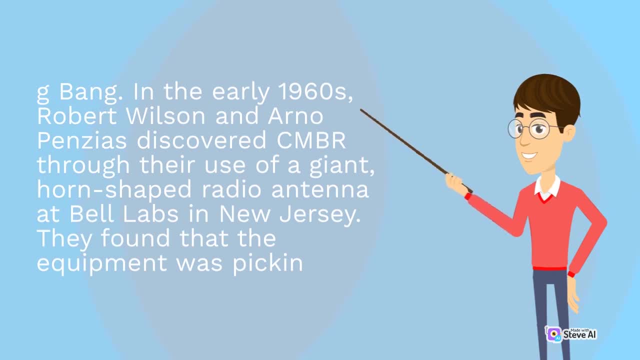 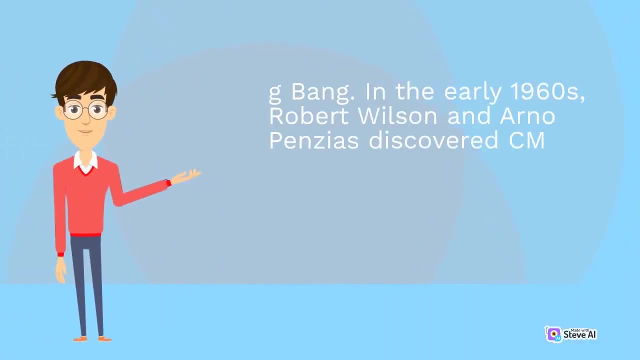 of a giant horn-shaped radio antenna at Bell Labs in New Jersey. They found that the equipment was picking Gee-bang. In the early 1960s, Robert Wilson and Arno Penzias discovered CMBR through their use of a. 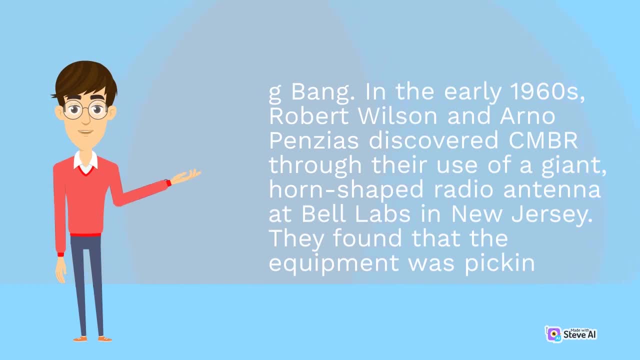 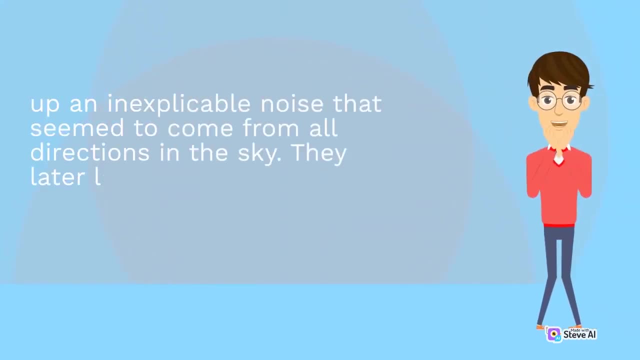 giant horn-shaped radio antenna at Bell Labs in New Jersey. They found that the equipment was picking Up an inexplicable noise that seemed to come from all directions in the sky. they later learned that this noise was in fact CMBR, which had remained incredibly uniform over. 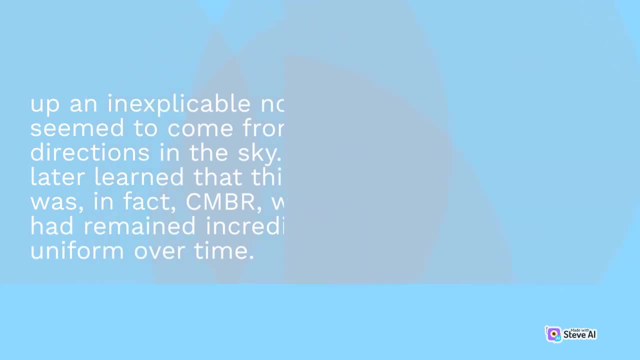 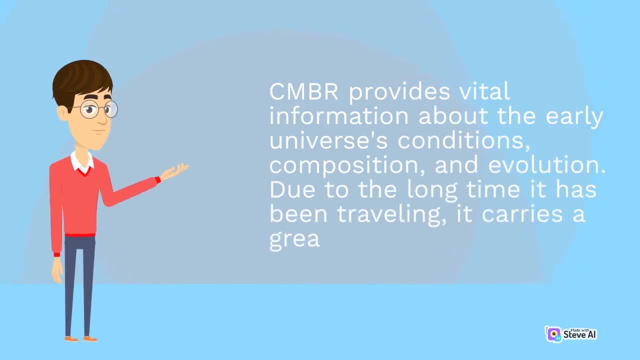 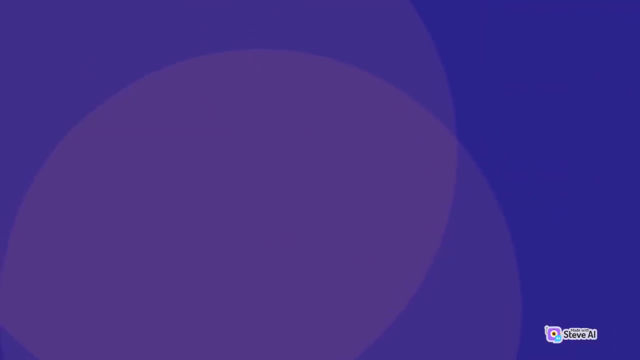 When it was first discovered, it was a very important piece of information. It was a very important piece of information. When it was first discovered, it was a very important piece of information. It was a very important piece of information S Observations and experiments contributing to our current understanding of these elusive objects. 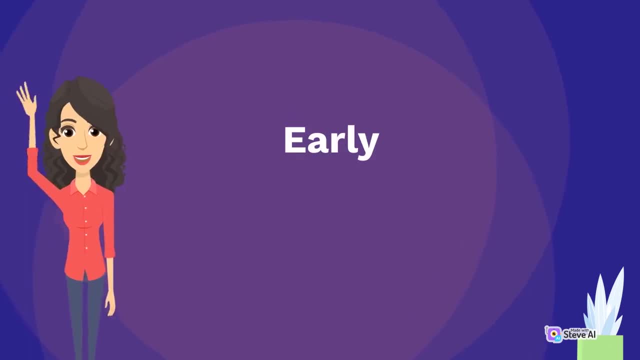 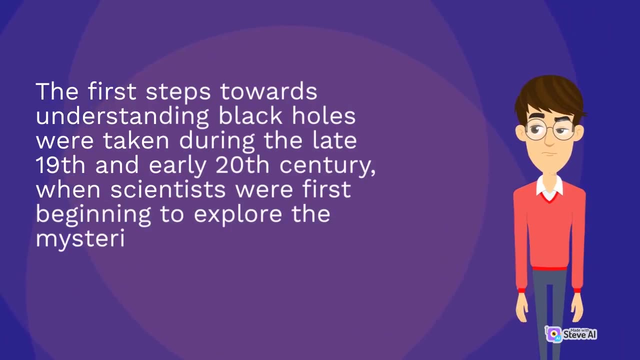 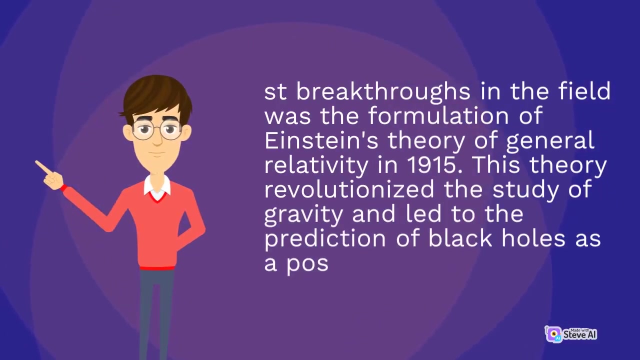 Early Theories and Observations. The first steps towards understanding black holes were taken during the late 19th and early 20th century, when scientists were first beginning to explore the mysteries of the cosmos. One of the early SD breakthroughs in the field was the formulation of Einstein's theory of general relativity in 1915. This theory revolutionized the study of gravity and led to the prediction of black holes as a POS. 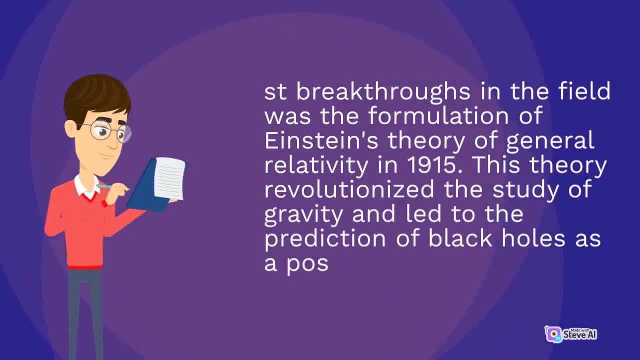 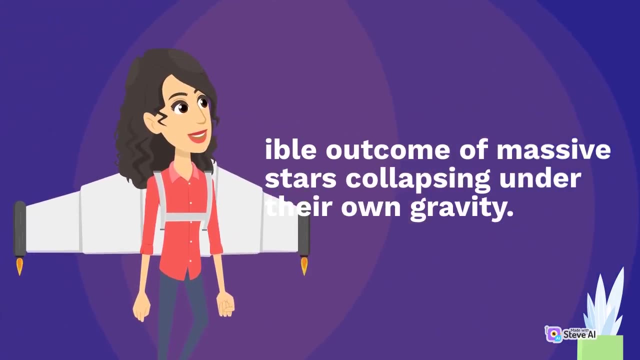 SD breakthroughs in the field was the formulation of Einstein's theory of general relativity in 1915. This theory revolutionized the study of gravity and led to the prediction of black holes as a POS Eyeball Outcome of Massive Stars Collapsing Under Their Own Gravity. 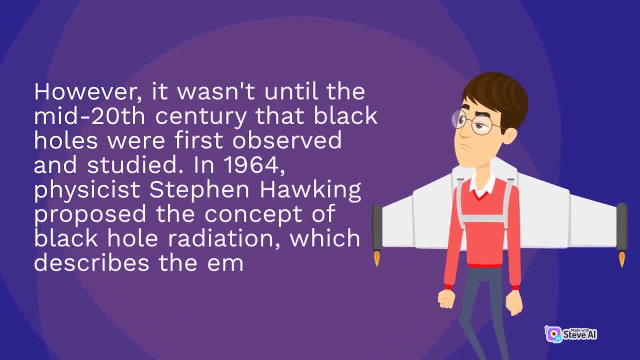 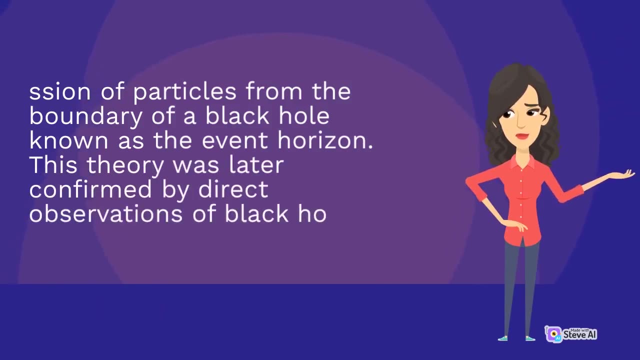 However, it wasn't until the mid-20th century that black holes were first observed and studied. In 1964, physicist Stephen Hawking proposed the concept of black hole radiation, which describes the M Shunt of Particles from the Boundary of a Black Hole Known as the Event Horizon. 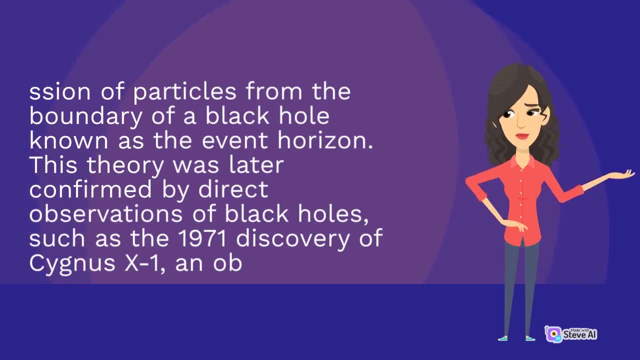 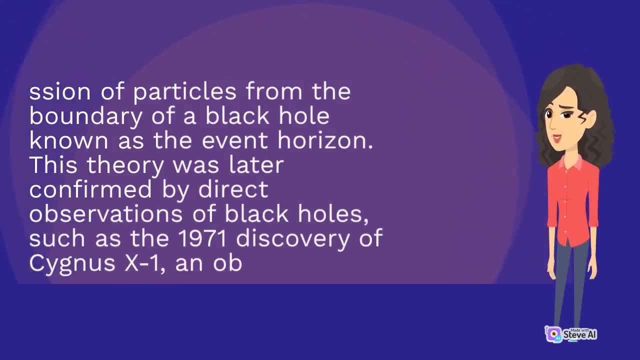 Shunt of Particles from the Boundary of a Black Hole Known as the Event Horizon black hole known as the event horizon. This theory was later confirmed by direct observations of black holes, such as the 1971 discovery of Cygnus X-1 and OB. 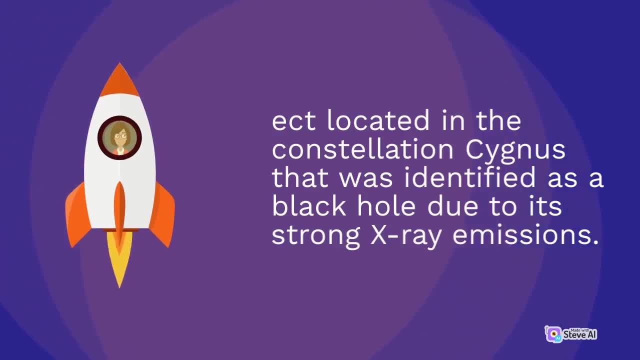 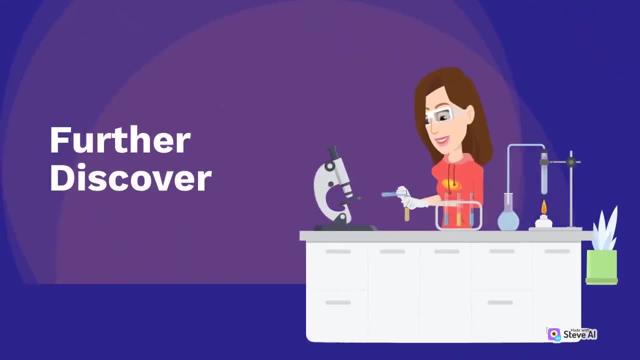 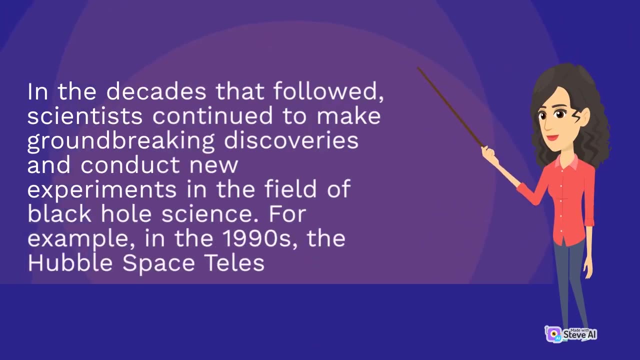 X, located in the constellation Cygnus. that was identified as a black hole due to its strong X-ray emissions. Further Discoveries and Experiments. In the decades that followed, scientists continued to make groundbreaking discoveries and conduct new experiments in the field of black hole science. For example, in the 1990s, the Hubble. 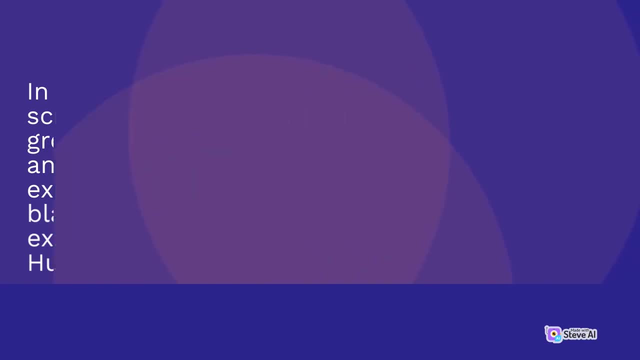 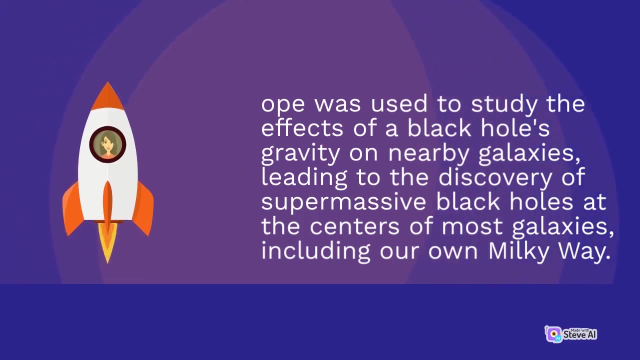 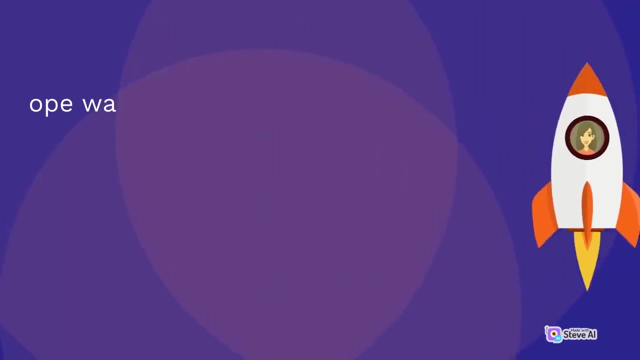 Space Telescope was used to study the effects of a black hole's gravity on nearby galaxies, leading to the discovery of supermassive black holes at the centers of most galaxies, including our own Milky Way. Another major breakthrough in black hole research came in 2015,, when the Laser Interferometer 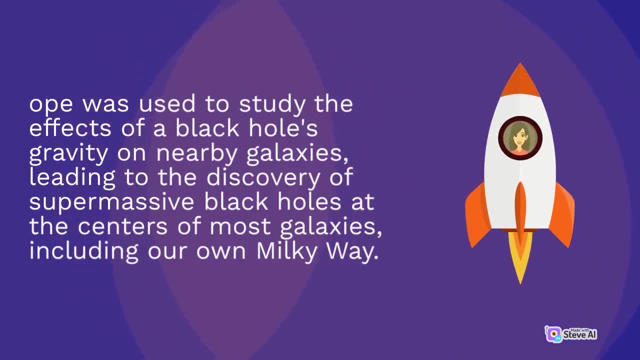 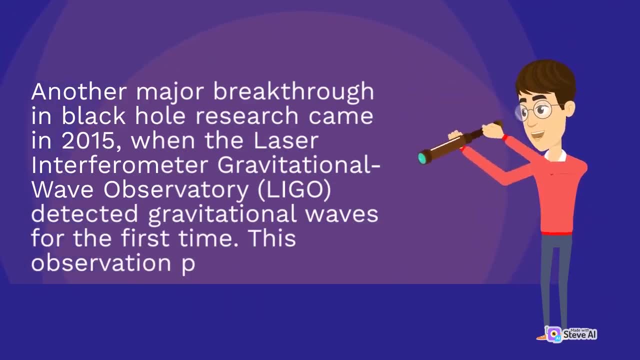 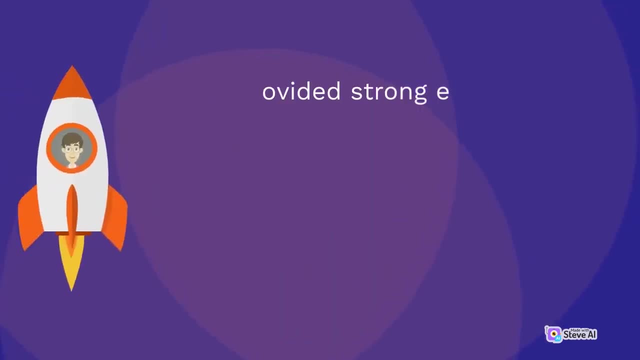 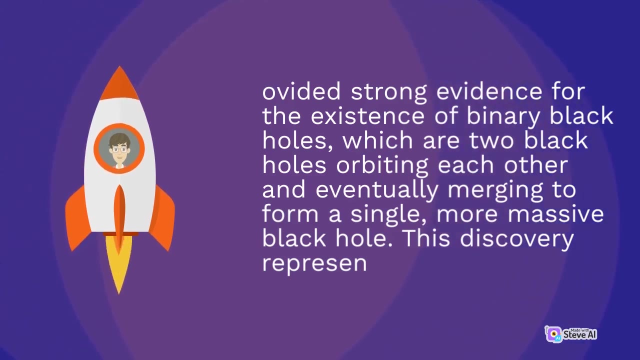 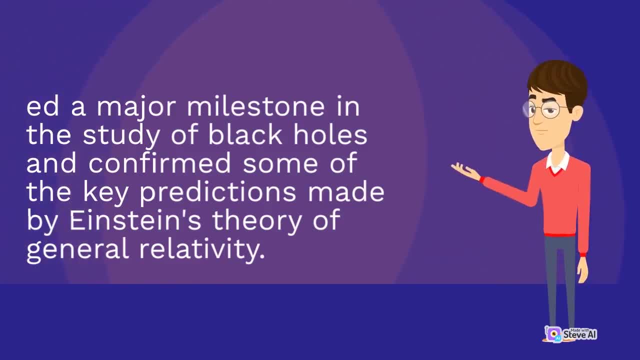 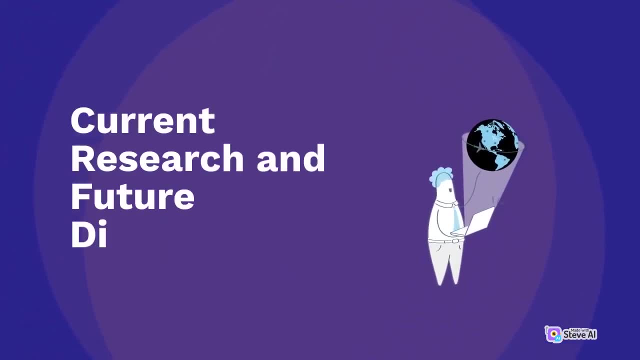 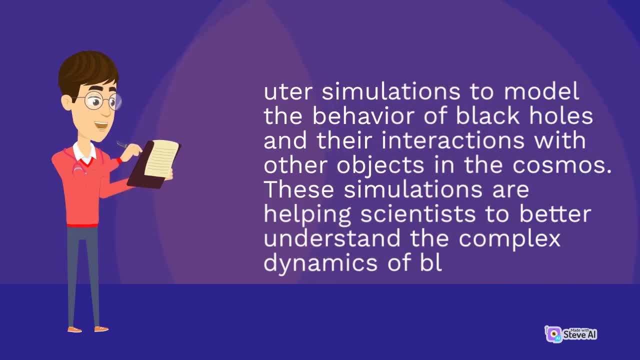 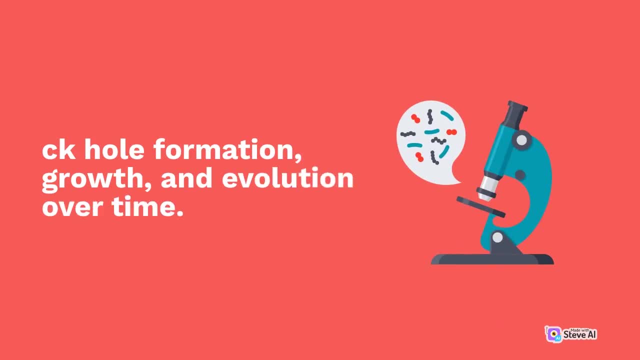 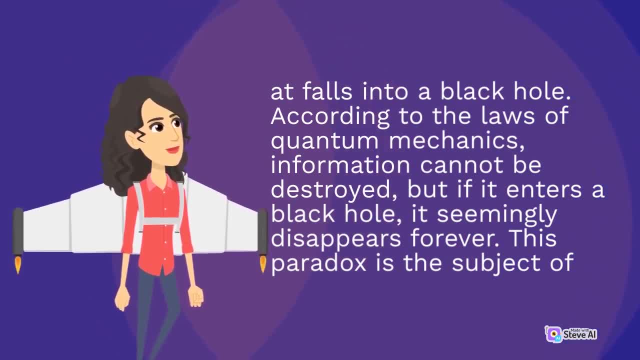 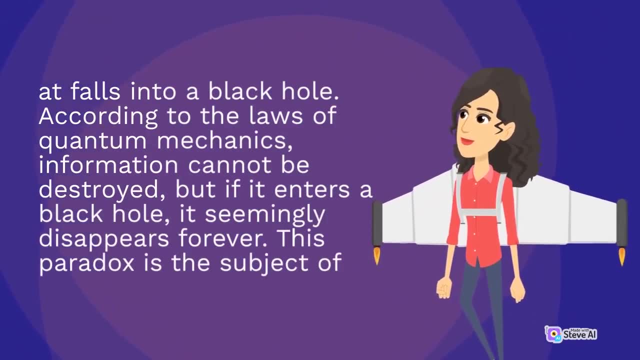 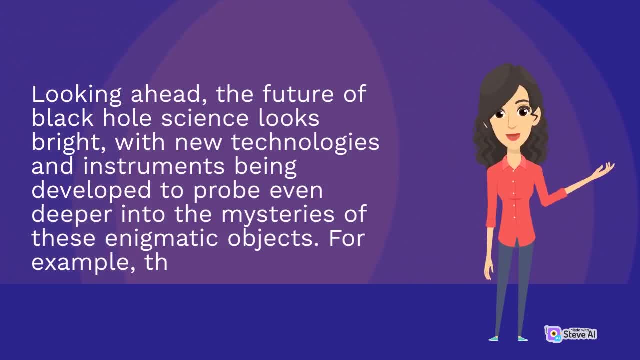 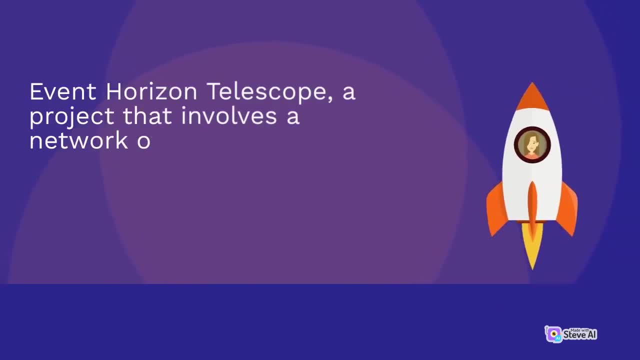 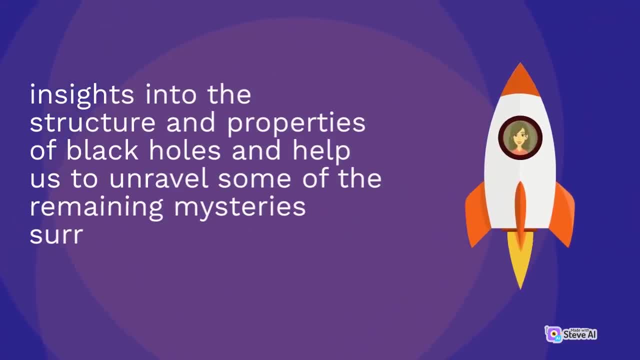 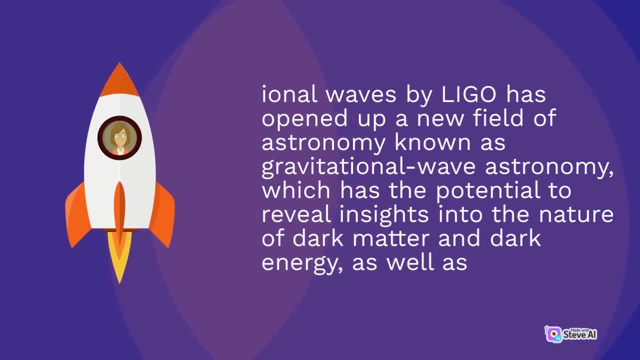 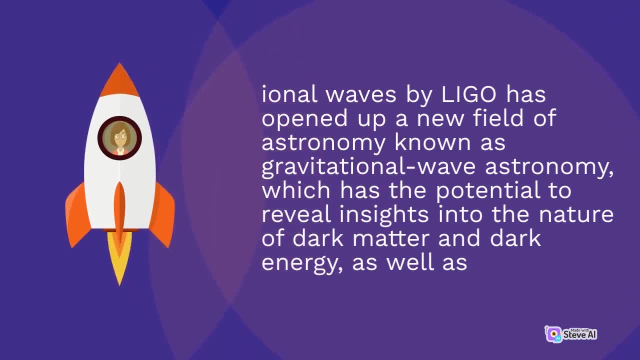 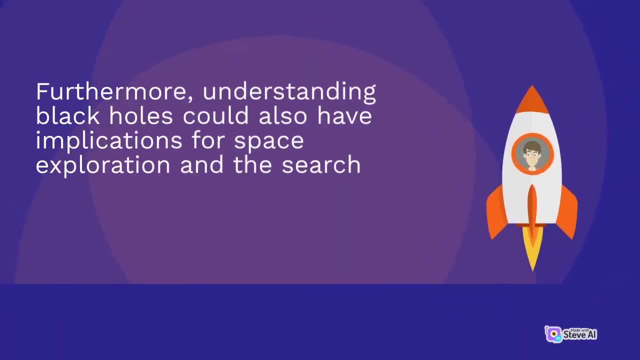 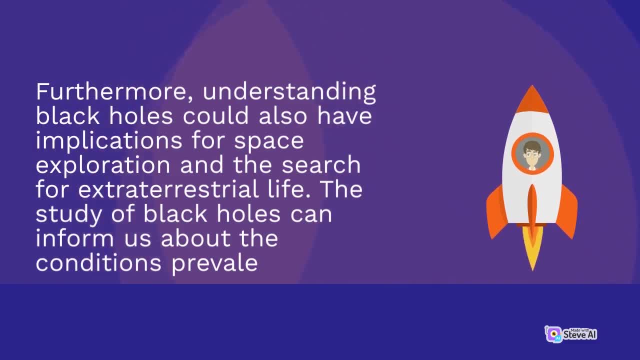 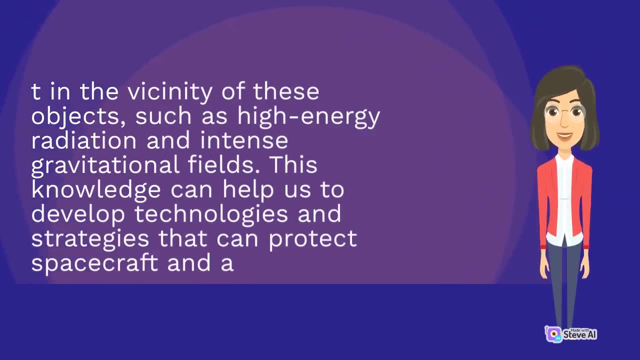 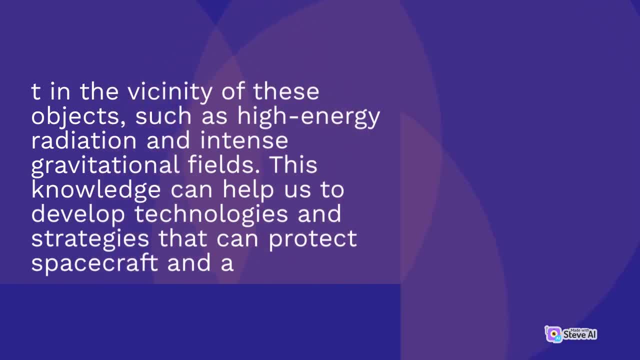 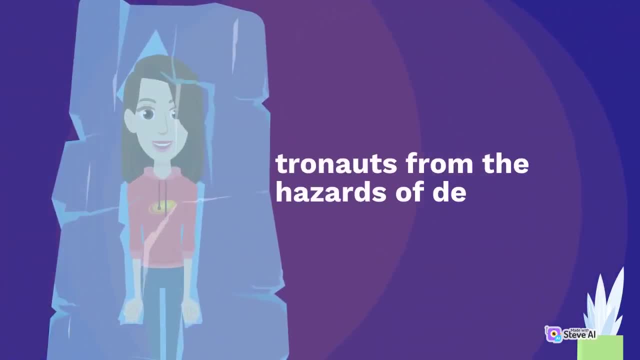 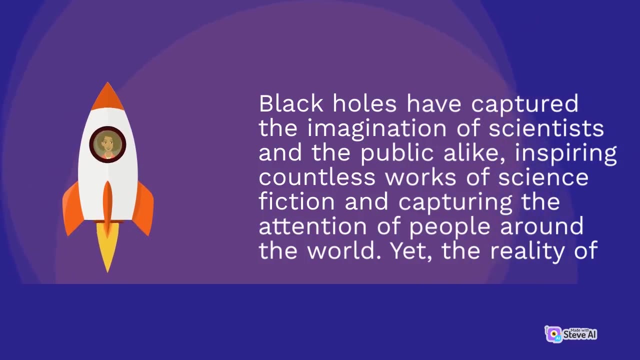 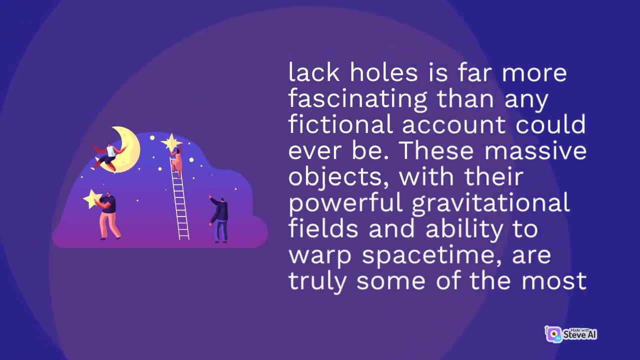 0. Trenauts from the Hazards of Deep Space. Black holes have captured the imagination of scientists and the public alike, inspiring countless works of science fiction and capturing the attention of people around the world. Yet the reality of Black holes is far more fascinating than any fictional account could ever be. These massive objects, with their powerful gravitational fields and ability to warp spacetime, are truly some of the most 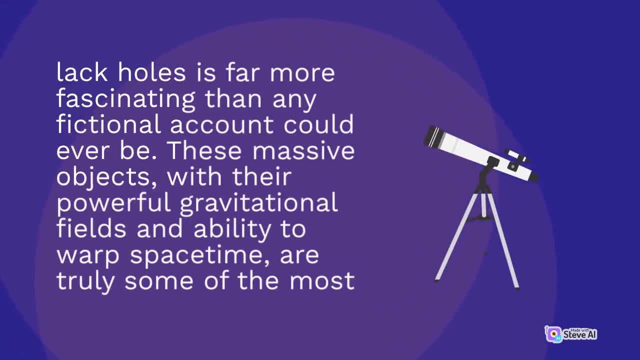 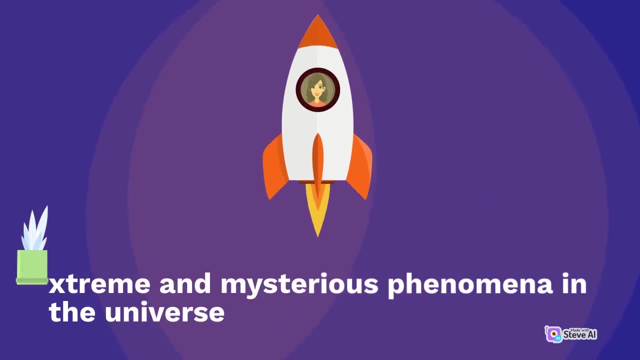 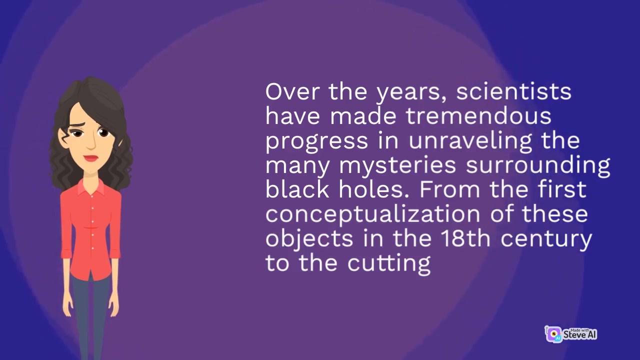 Black holes is far more fascinating than any fictional account could ever be. These massive objects, with their powerful gravitational fields and ability to warp spacetime, are truly some of the most X-ray, Extreme and Mysterious Phenomena in the Universe. Over the years, scientists have made tremendous progress in unraveling the many mysteries surrounding black holes. From the first conceptualization of these objects in the 18th century to the cutting 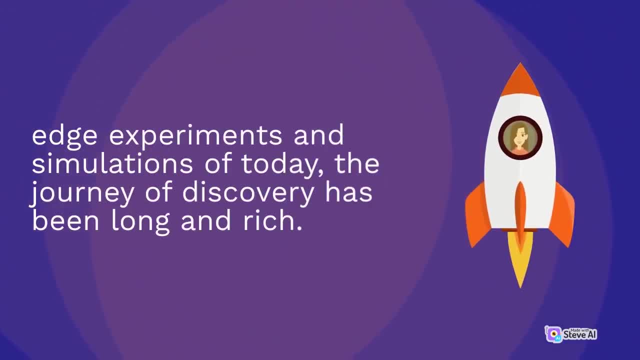 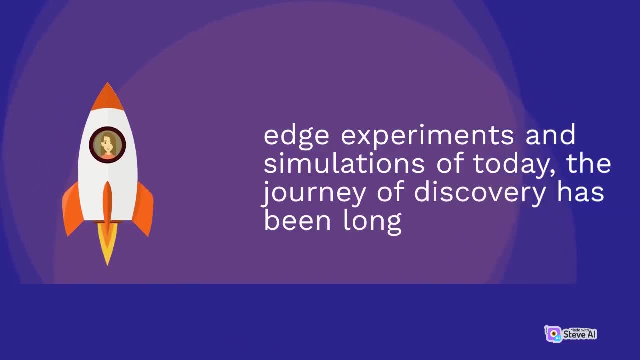 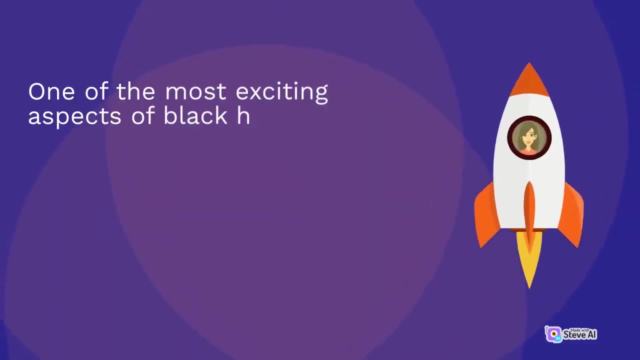 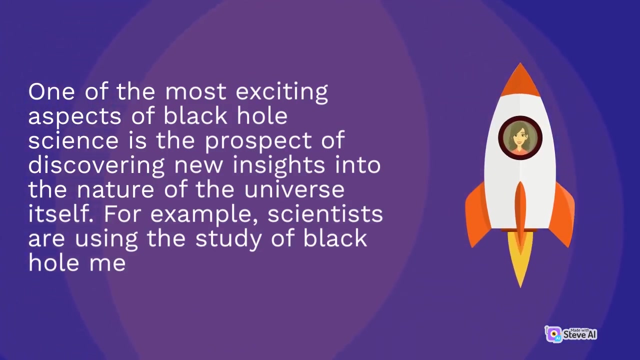 edge experiments and simulations of today. the journey of discovery has been long and rich. Edge Experiments and Simulations of Today. Edge Experiments and Simulations of Today. The journey of discovery has been long and rich. One of the most exciting aspects of black hole science is the prospect of discovering new insights into the nature of the universe itself. For example, scientists are using the study of Black Hole Me. 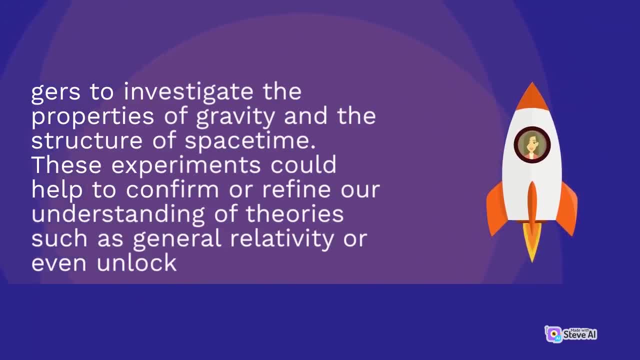 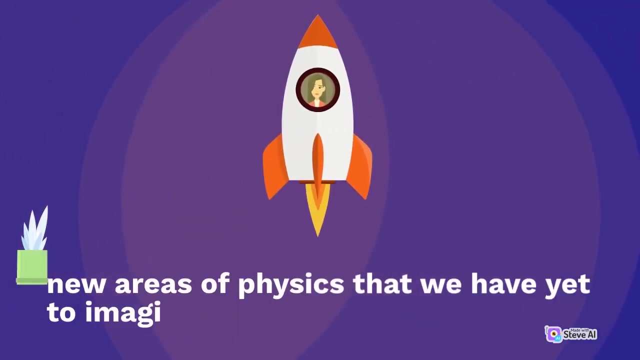 to investigate the properties of gravity and the structure of spacetime. These experiments could help to confirm or refine our understanding of theories such as general relativity or conclusion andamente, the zero. At the same time, the study of black holes is also revealing new information about the formation and evolution of galaxies and chimneys. 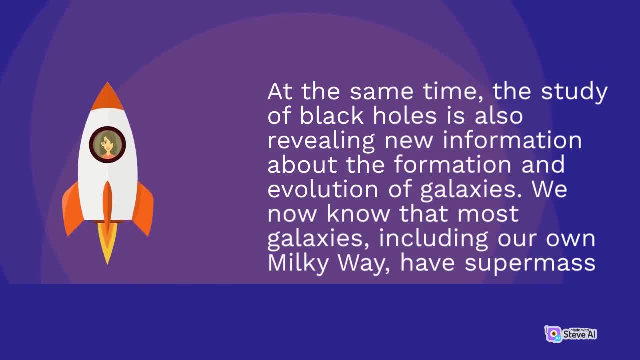 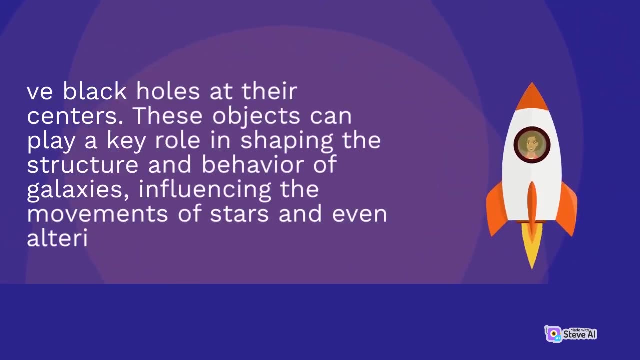 History, History également. Philosophy, Technology, Data, galaxies. We now know that most galaxies, including our own, Milky Way, have supermass. They black holes at their centers. These objects can play a key role in shaping the structure and behavior of galaxies, influencing the movements of stars, even altering the surrounding interstellar. 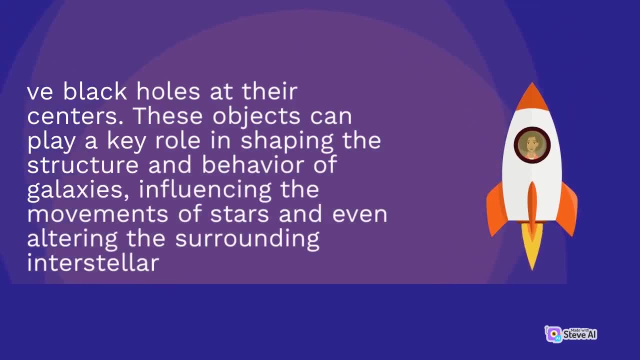 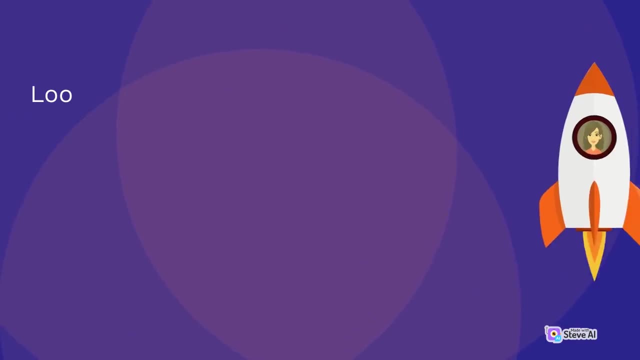 They black holes at their centers. These objects can play a key role in shaping the structure and behavior of galaxies, influencing the movements of stars, even altering the surrounding interstellar Medium. Looking ahead, there will undoubtedly be many more exciting discoveries and breakthroughs to 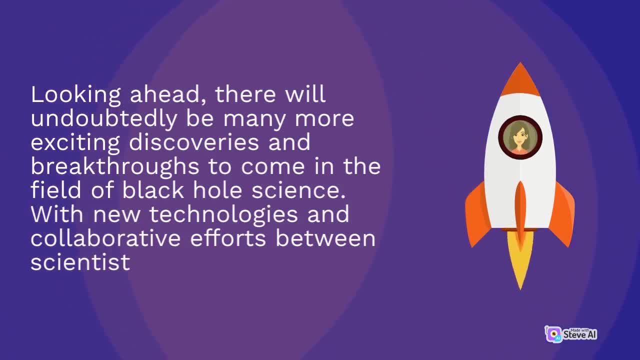 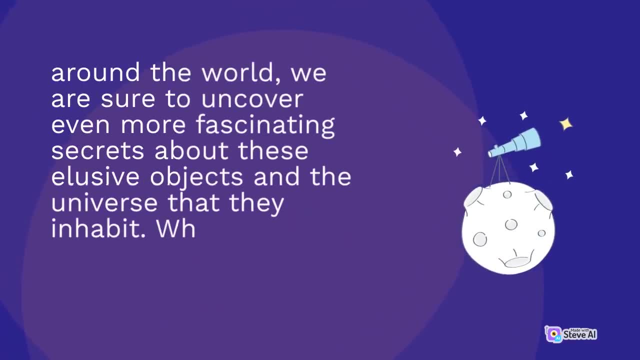 come in the field of black hole science. With new technologies and collaborative efforts between scientists around the world, we are sure to uncover even more fascinating secrets about these elusive galaxies, objects and the universe that they inhabit. Whether we are seeking to unravel the mysteries, 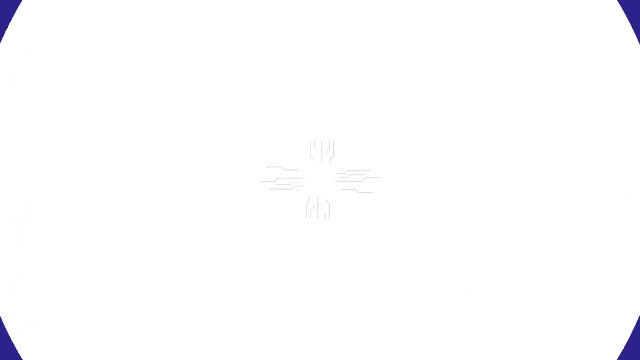 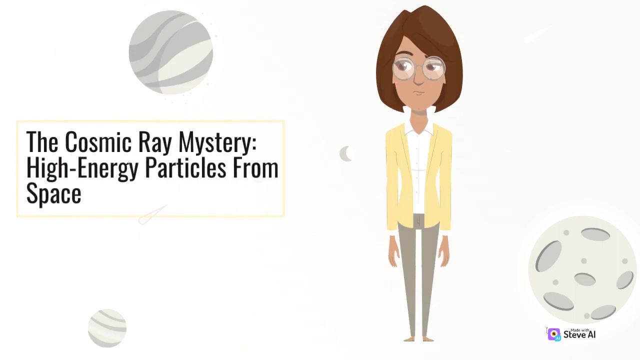 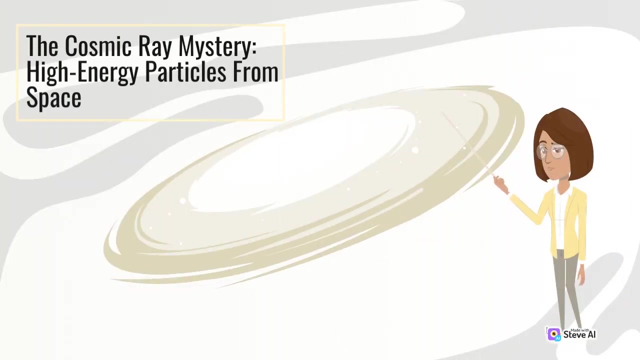 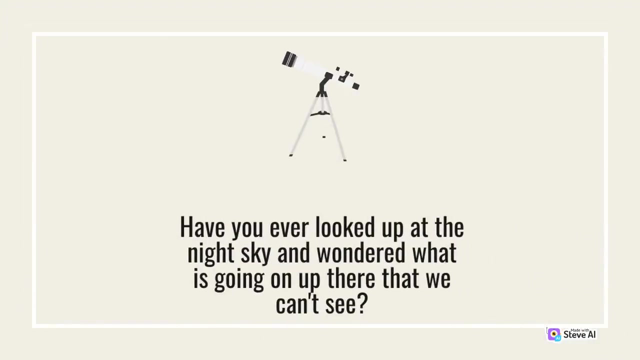 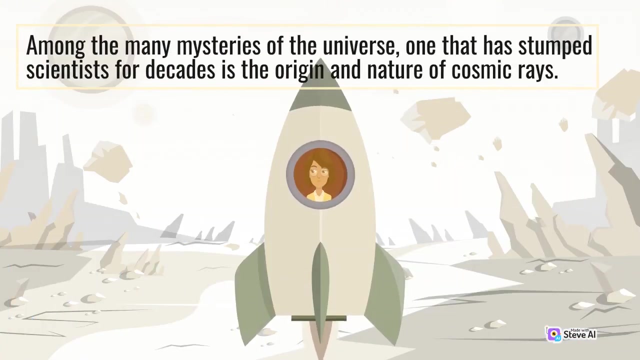 of gravity and the cosmic ray mystery- high energy particles from space. The cosmic ray mystery- high energy particles from space. Have you ever looked up at the night sky and wondered what is going on up there that we can't see? Among the many mysteries of the universe, one that has stumped scientists for decades is the origin. 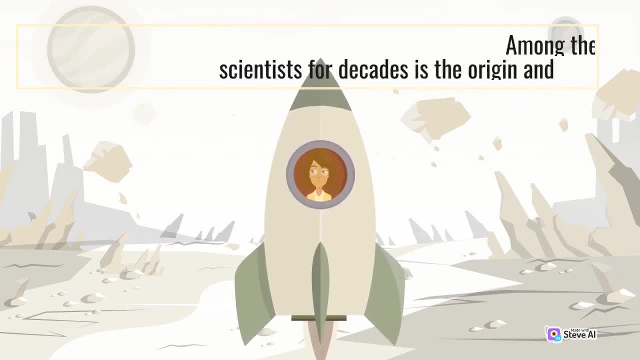 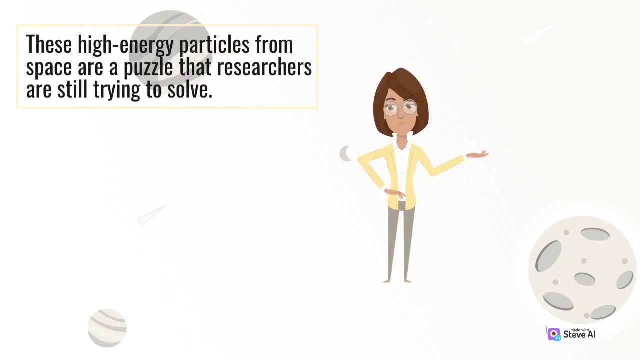 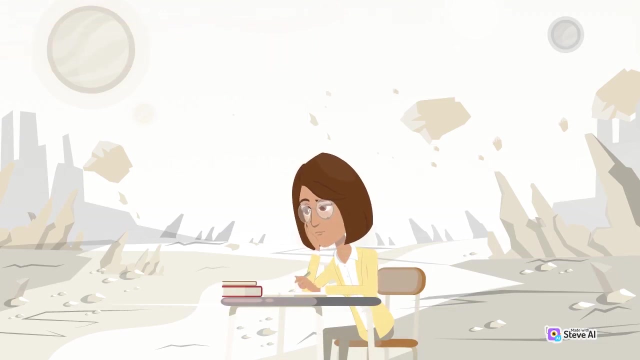 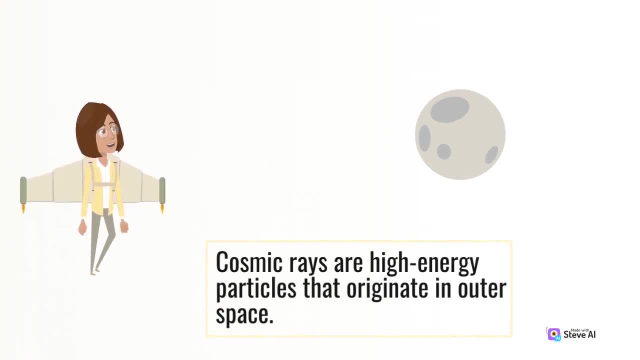 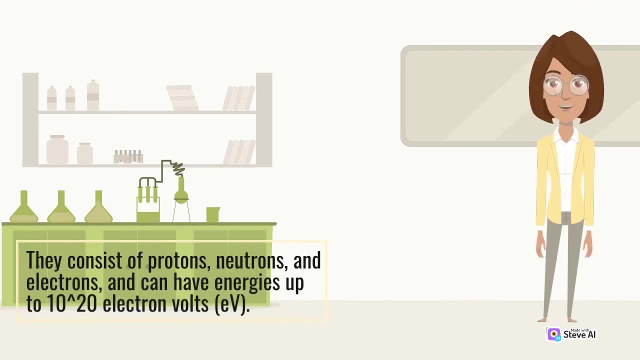 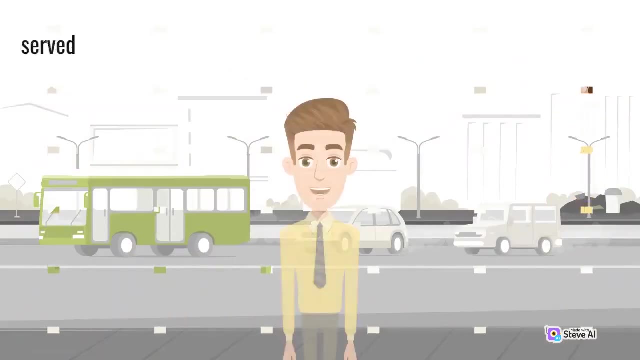 Cosmic rays are high-energy particles that originate in outer space. They consist of protons, neutrons and electrons and can have energies up to 10 to the power of 20 electron volts. To put that into perspective, the highest energy particle ever observed from a man-made 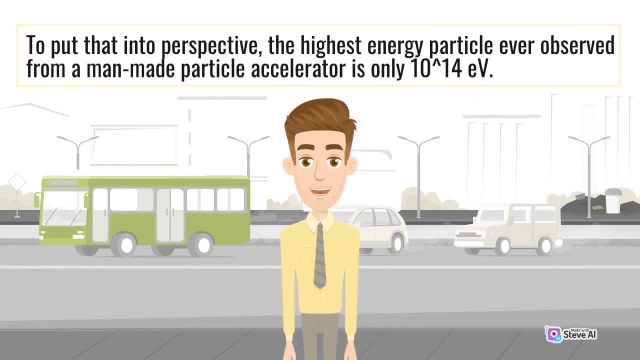 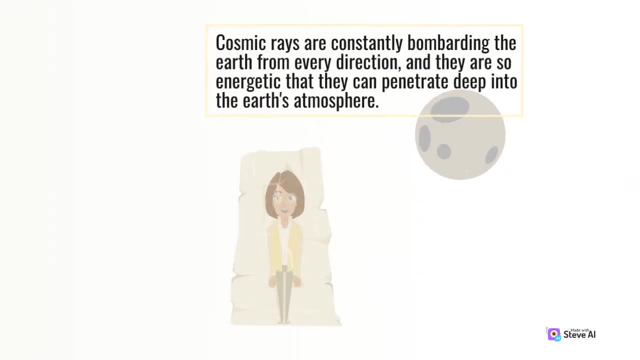 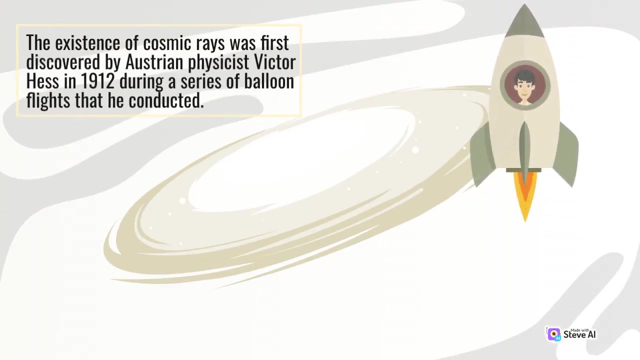 particle accelerator is only 10 to the power of 14 F. Cosmic rays are constantly bombarding the Earth from every direction, and they are so energetic that they can penetrate deep into the Earth's atmosphere. The Discovery of Cosmic Rays. The existence of cosmic rays was first discovered by Austrian physicist Victor Hess in 1912. 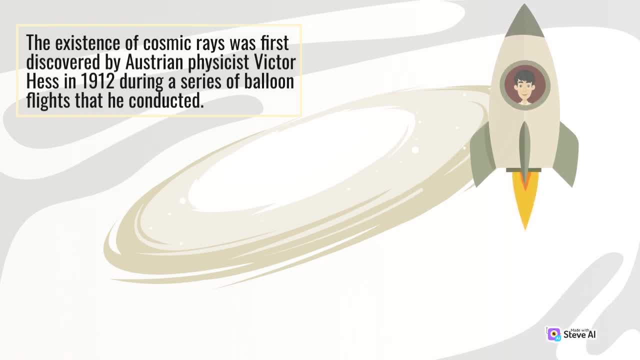 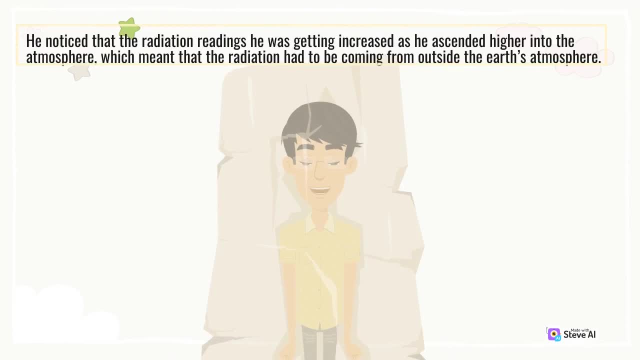 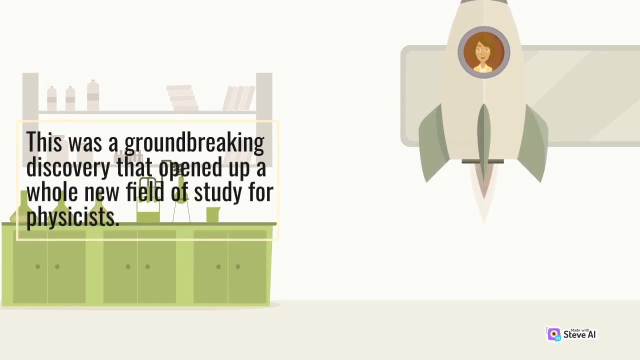 during a series of experiments, He noticed that the radiation readings he was getting increased as he ascended higher into the atmosphere, which meant that the radiation had to be coming from outside the Earth's atmosphere. This was a groundbreaking discovery that opened up a whole new field of study for physicists. 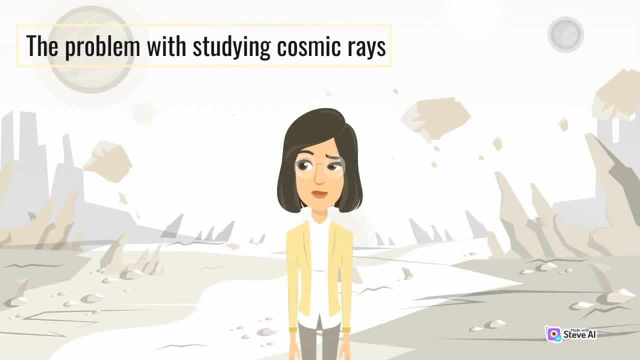 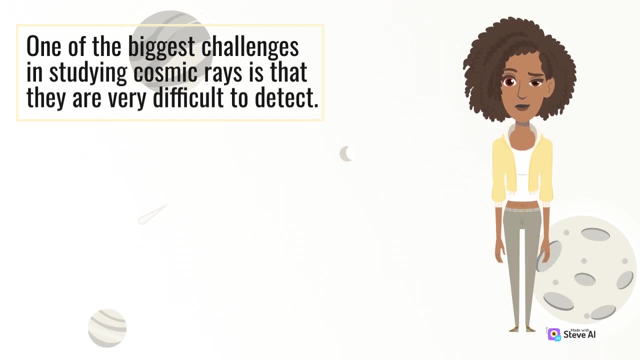 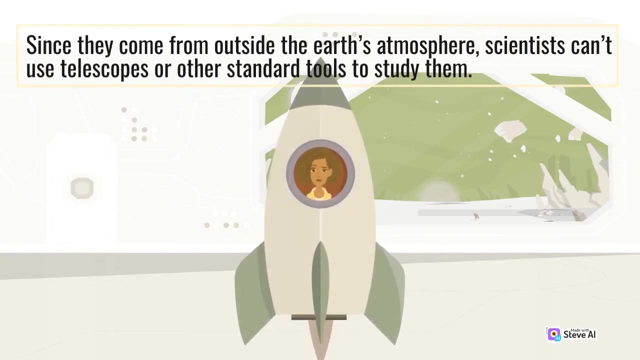 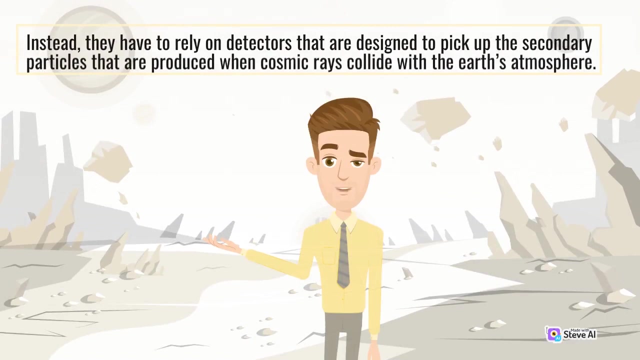 The Problem with Studying Cosmic Rays. One of the biggest challenges in studying cosmic rays is that they are very difficult to detect, Since they come from outside the Earth's atmosphere. scientists can't use telescopes or other standard tools to study them. Instead, they have to rely on detectors that are designed to pick up the secondary particles. 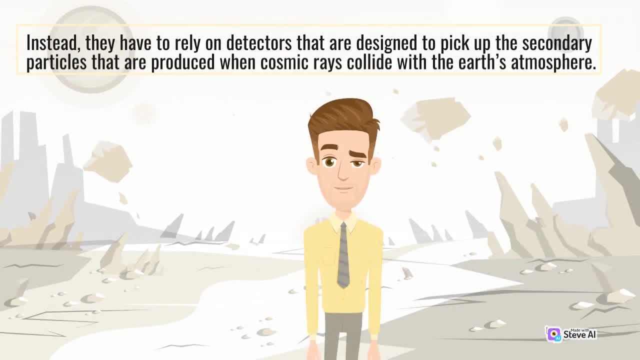 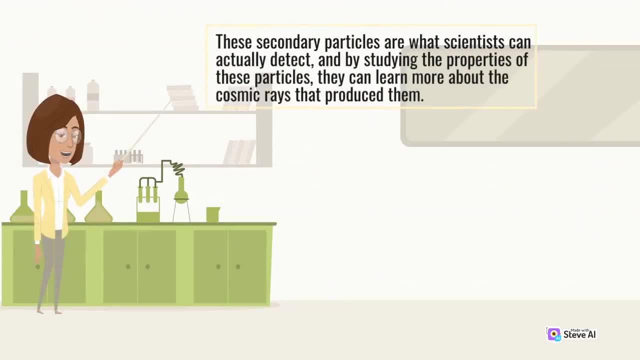 that are produced when cosmic rays collide with the Earth's atmosphere. The problem with studying cosmic rays is that they are very difficult to detect. They are not easily detected And by studying the properties of these particles they can learn more about the cosmic rays. 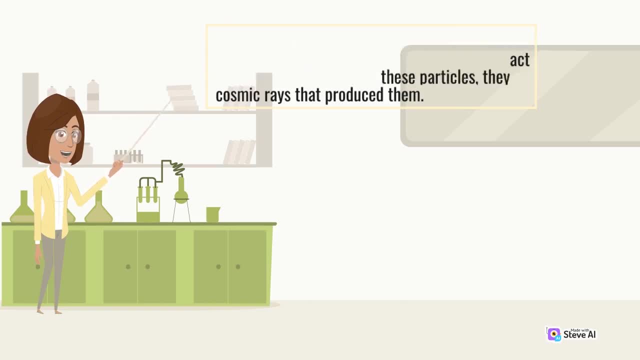 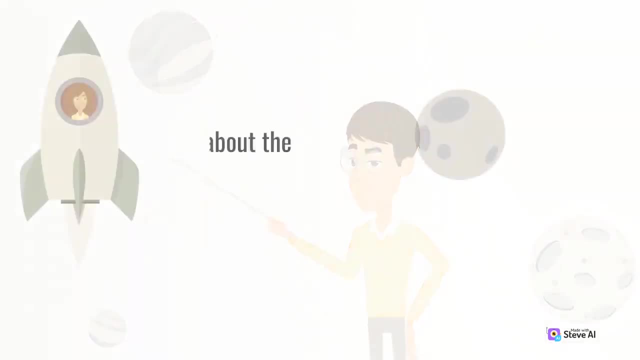 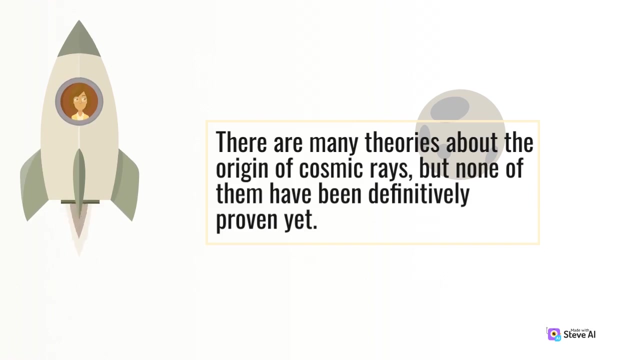 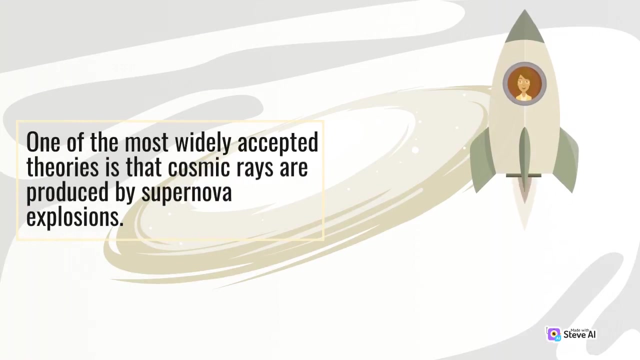 that produce them. Theories About The Origin Of Cosmic Rays. There are many theories about the origin of cosmic rays, but none of them have been definitively proven yet. One of the most widely accepted theories is that cosmic rays are produced by supernova explosions. 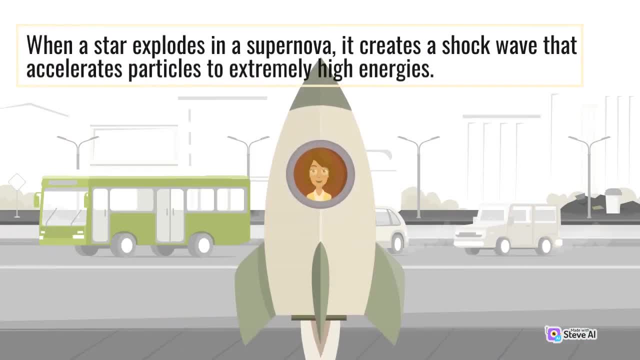 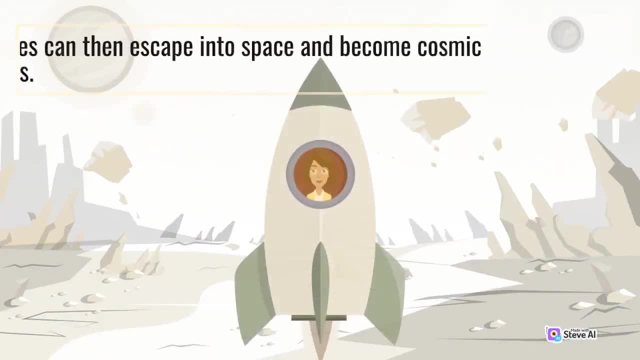 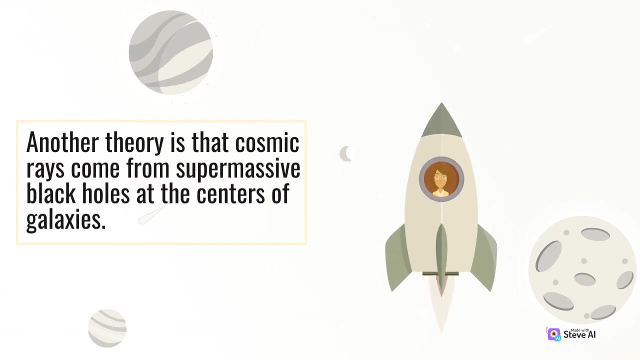 When a star explodes in a supernova, it creates a shock wave that accelerates particles to extremely high energies. These particles can then escape into space and become cosmic rays. Another theory is that cosmic rays come from supermassive black holes at the centers of galaxies. 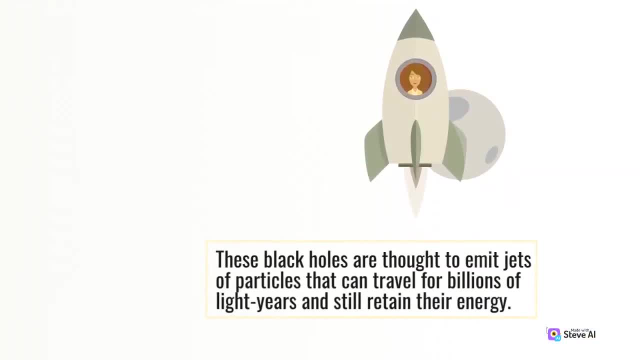 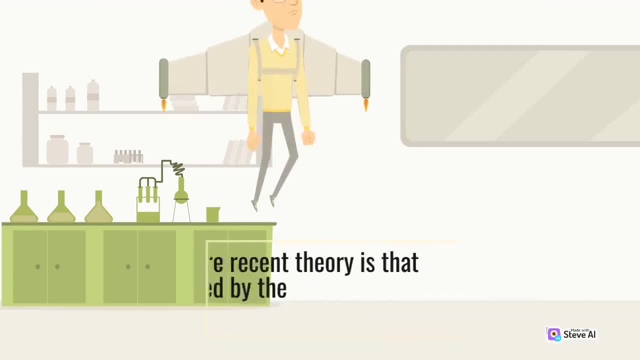 These black holes are thought to emit jets of particles that can travel for billions of light-years and still retain their energy. A more recent theory is that cosmic rays are produced by the collision of dark matter particles. Dark matter is a mysterious substance that makes it possible for a star to explode. 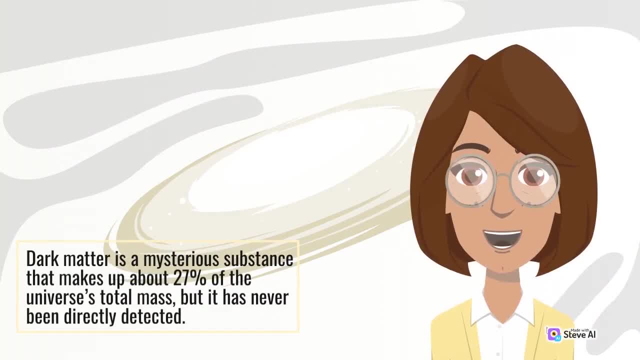 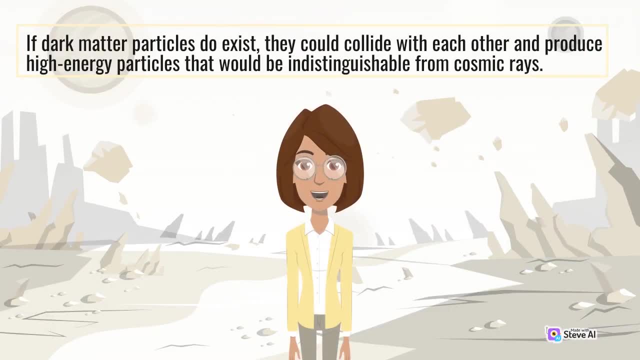 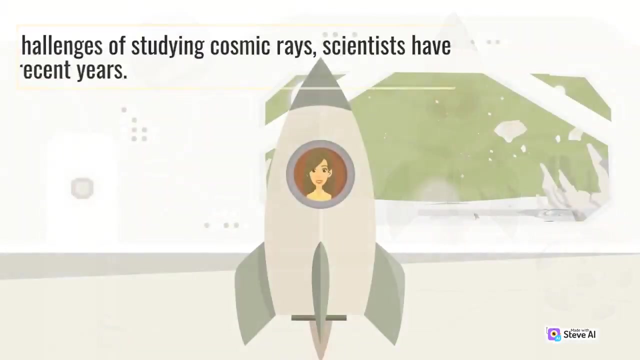 It makes up about 27% of the universe's total mass, but it has never been directly detected. If dark matter particles do exist, they could collide with each other and produce high-energy particles that would be indistinguishable from cosmic rays. The Study of Cosmic Rays. 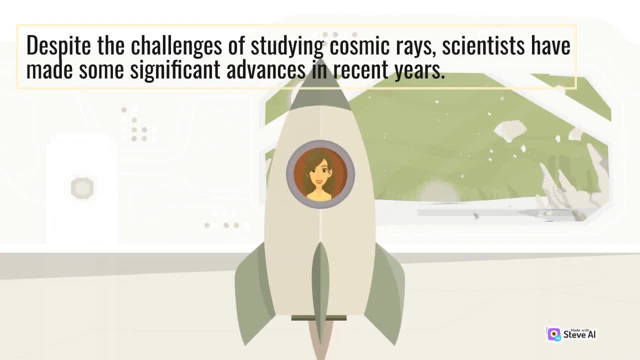 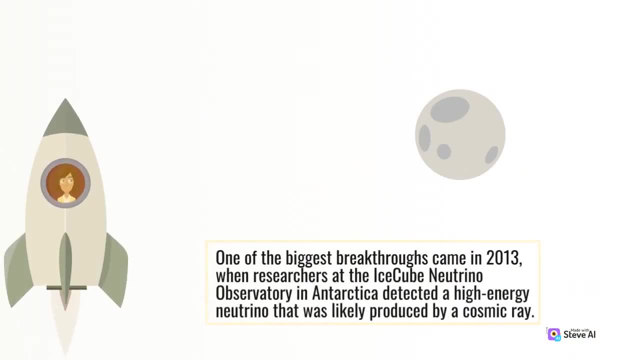 Despite the challenges of studying cosmic rays, scientists have made some significant advances in research The study of cosmic rays. One of the biggest breakthroughs came in 2013,, when researchers at the IceCube Neutrino Observatory in Antarctica detected a high-energy neutrino that was likely produced by a cosmic ray. 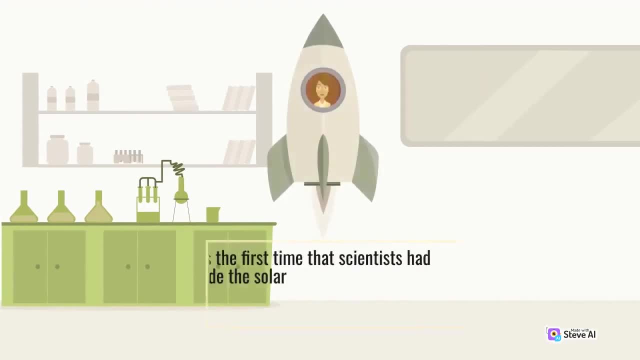 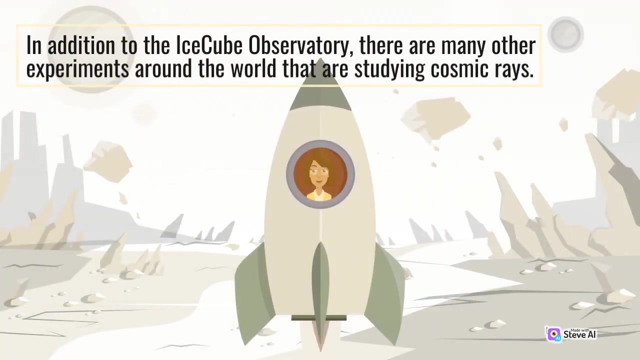 This was the first time that scientists had detected a cosmic ray from outside the solar system, and it provided valuable information about the nature of these mysterious particles. In addition to the IceCube Observatory, there are many other experiments around the world that are studying cosmic rays. 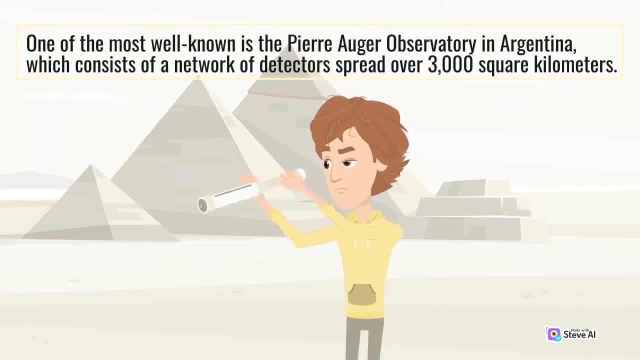 One of the most well-known is the Pierre Auger Observatory in Argentina, which consists of a network of detectors spread over 3,000 square kilometers. The observatory is designed to study the highest-energy cosmic rays and it has made some significant discoveries in recent years. 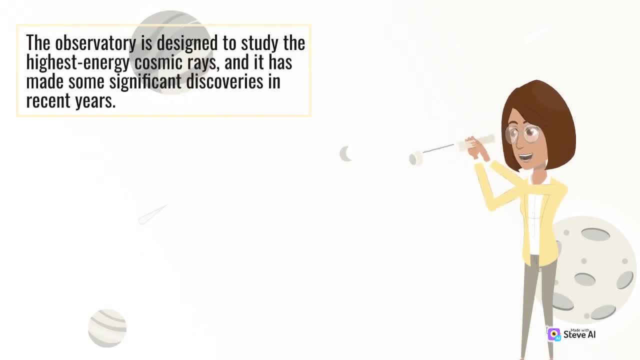 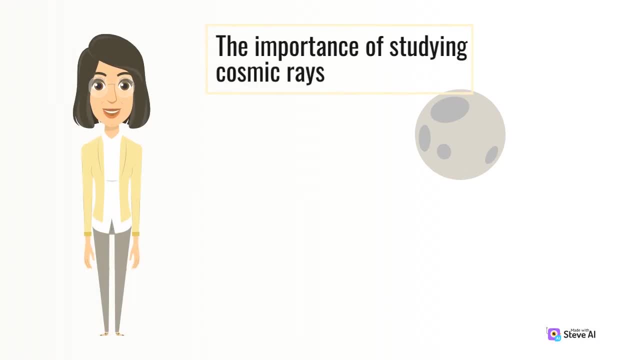 The observatory is designed to study the highest-energy cosmic rays and it has made some significant discoveries in recent years. The observatory is designed to study the highest-energy cosmic rays and it has made some significant discoveries in recent years. The importance of studying cosmic rays. 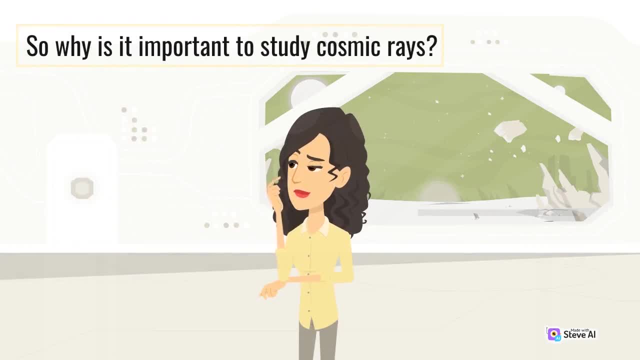 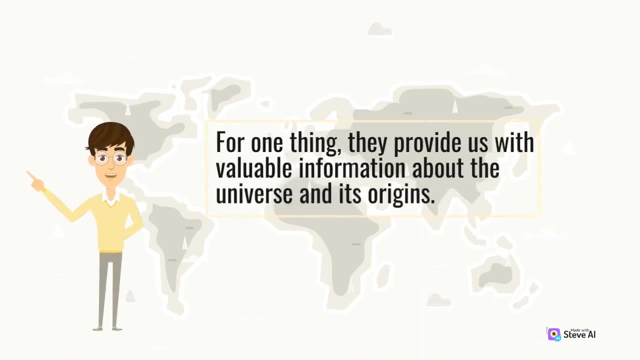 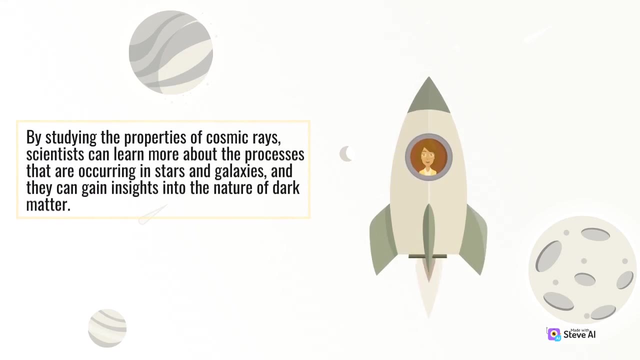 So why is it important to study cosmic rays? For one thing, they provide us with valuable information about the universe and its origins. By studying the properties of cosmic rays, scientists can learn more about the process of studying cosmic rays. By studying the properties of cosmic rays, scientists can learn more about the process of studying cosmic rays. By studying the properties of cosmic rays, scientists can learn more about the processes that are occurring in stars and galaxies, and they can gain insights into the nature of dark matter. By studying the properties of cosmic rays, scientists can learn more about the processes that are occurring in stars and galaxies, and they can gain insights into the nature of dark matter. By studying the properties of cosmic rays, scientists can learn more about the processes that are occurring in stars and galaxies, and they can gain insights into the nature of dark matter. By studying the properties of cosmic rays, scientists can learn more about the processes that are occurring in stars and galaxies, and they can gain insights into the nature of dark matter. 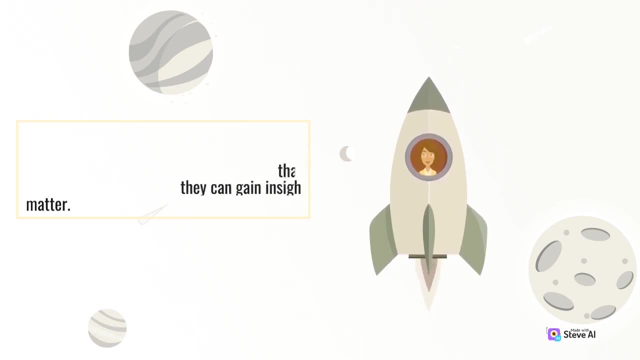 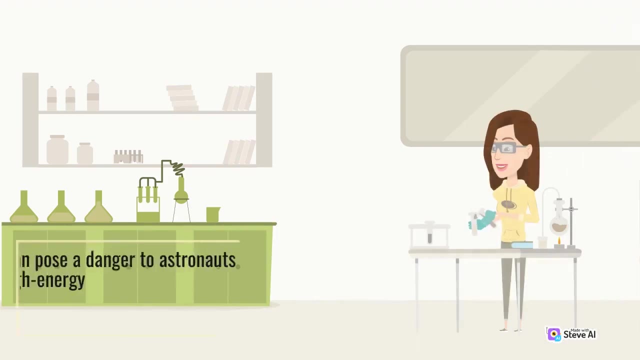 By studying the properties of cosmic rays, scientists can learn more about the processes that are occurring in stars and galaxies, and they can gain insights into the nature of dark matter matter. Cosmic rays also have practical applications. They can pose a danger to astronauts and spacecraft, as the high-energy particles can cause damage. 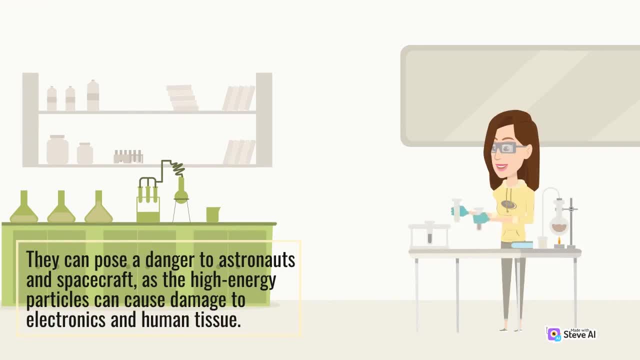 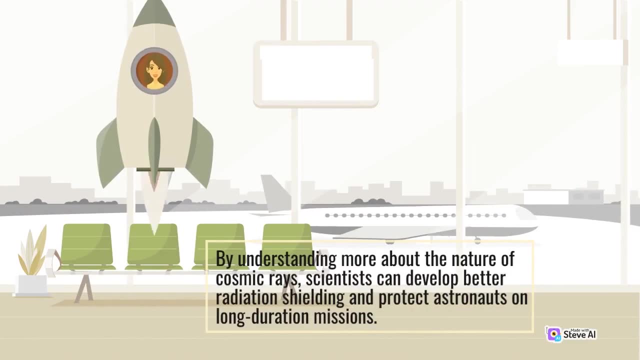 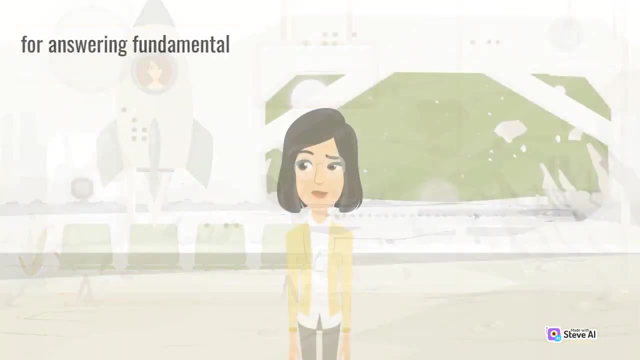 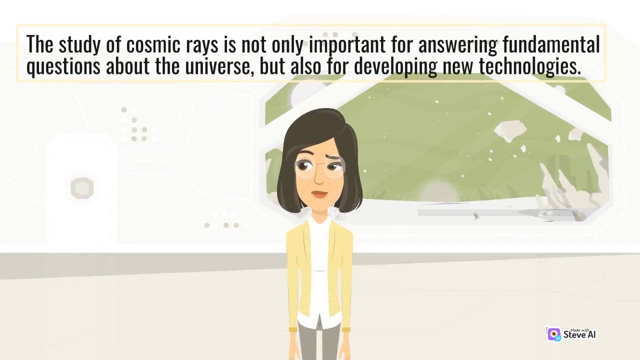 to electronics and human tissue. By understanding more about the nature of cosmic rays, scientists can develop better radiation shielding and protect astronauts on long-duration missions. The study of cosmic rays is not only important for answering fundamental questions about the universe, but also for developing new technologies. 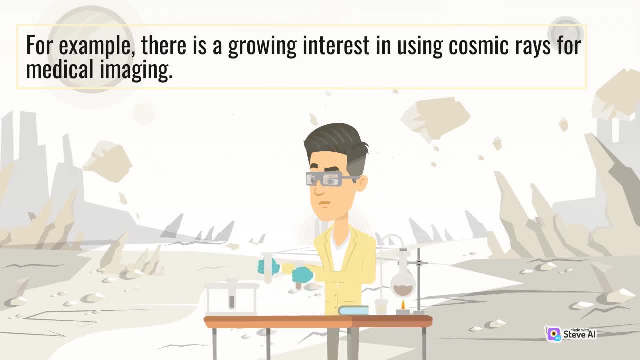 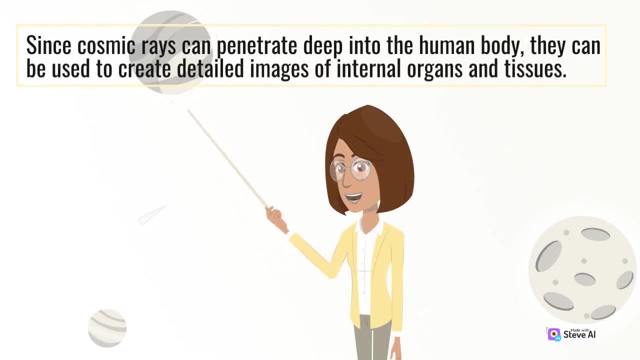 For example, there is a growing interest in using cosmic rays for medical imaging. Since cosmic rays can penetrate deep into the human body, they can be used to create detailed images of internal organs and tissues. This technique, known as muon tomography, has the potential to be a safer and more cost-effective. 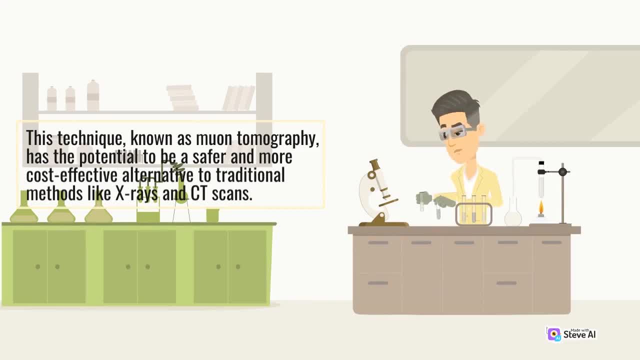 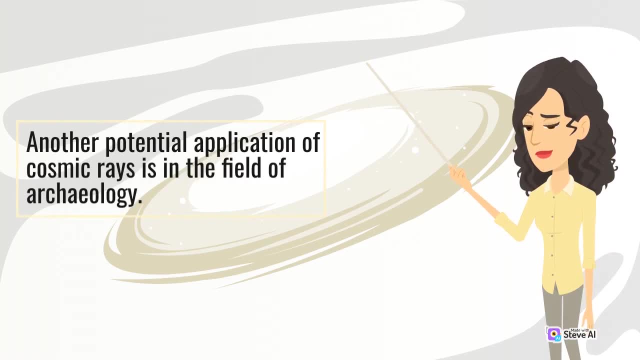 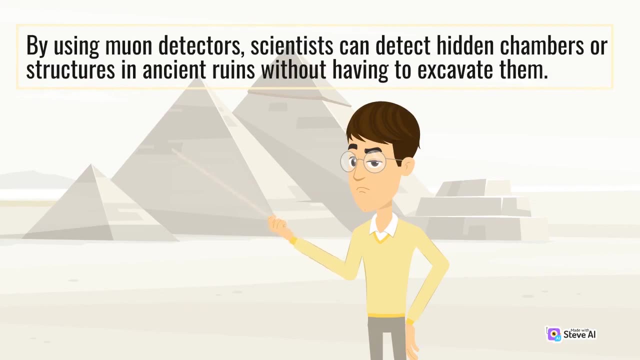 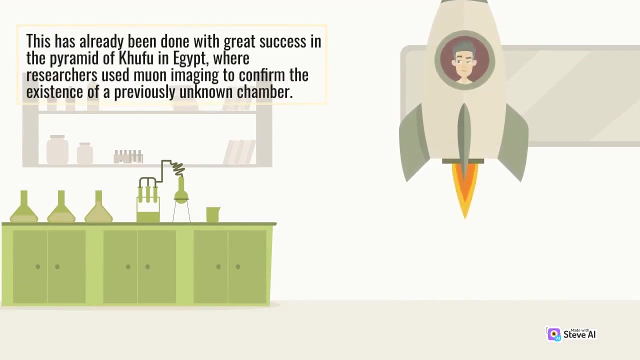 alternative to traditional methods like X-rays and CT scans. Another potential application of cosmic rays is in the field of archaeology. By using muon detectors, scientists can detect hidden chambers or structures in ancient ruins without having to excavate them. This has already been done with great success in the Pyramid of Khufu in Egypt, where researchers 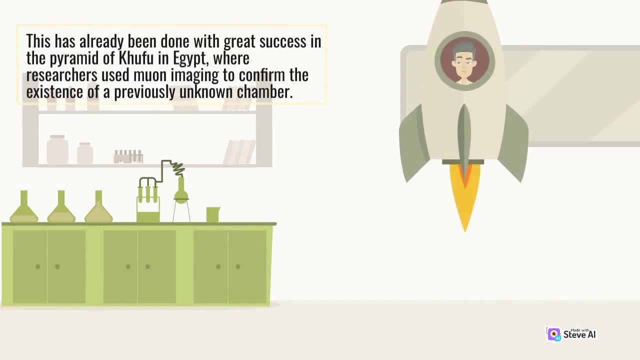 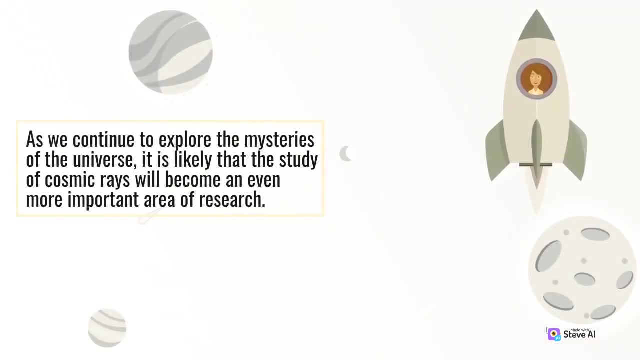 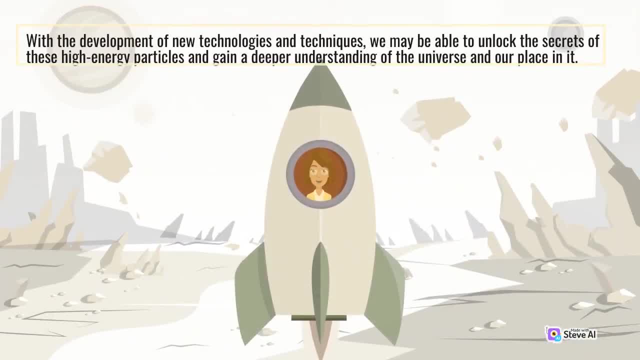 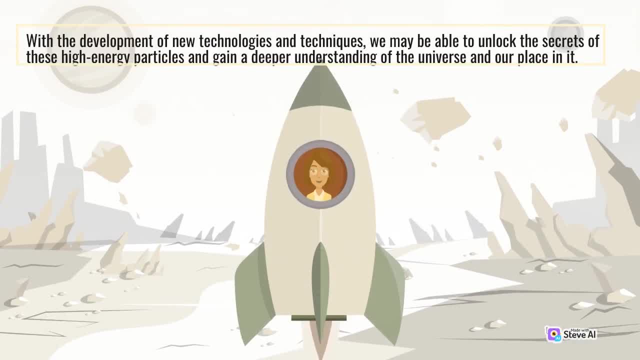 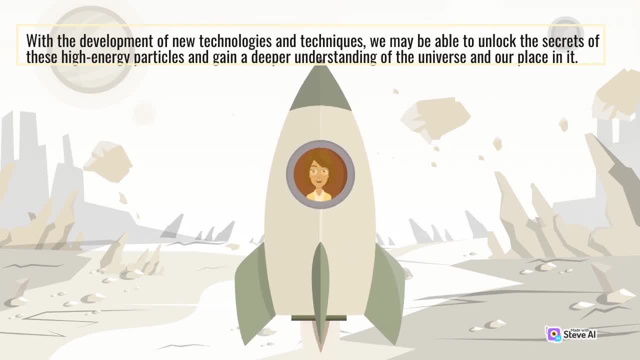 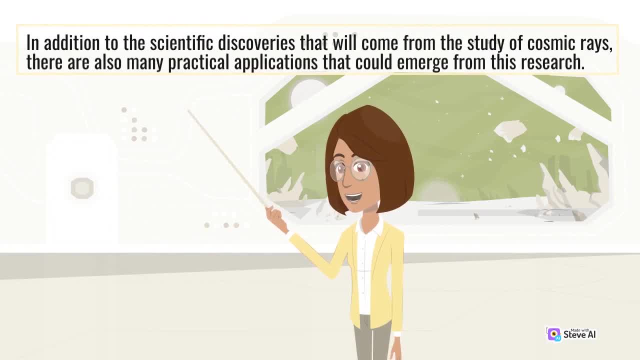 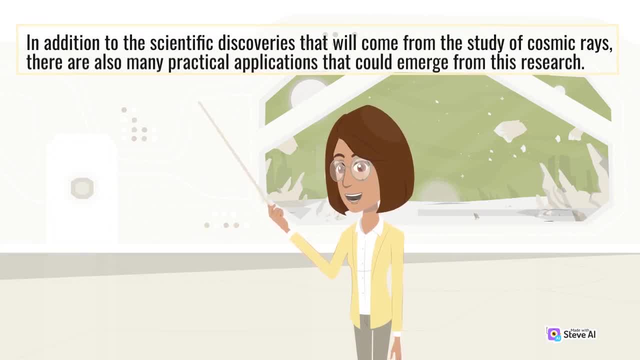 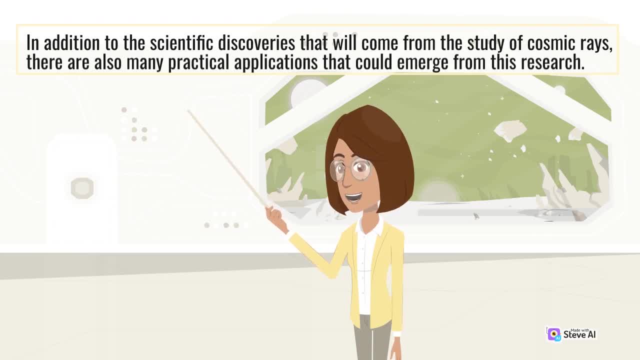 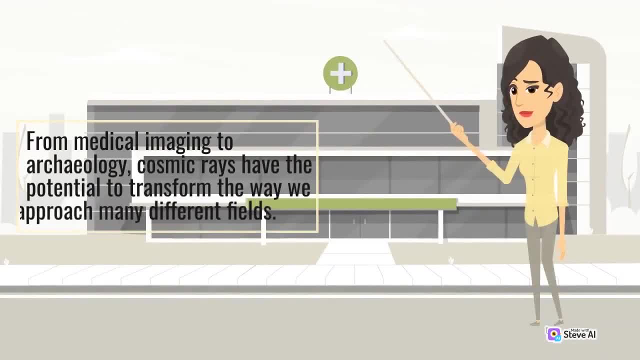 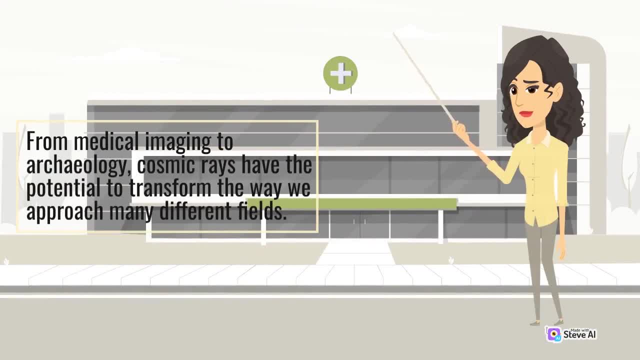 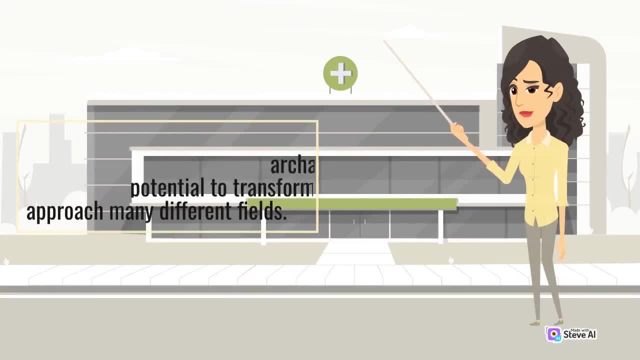 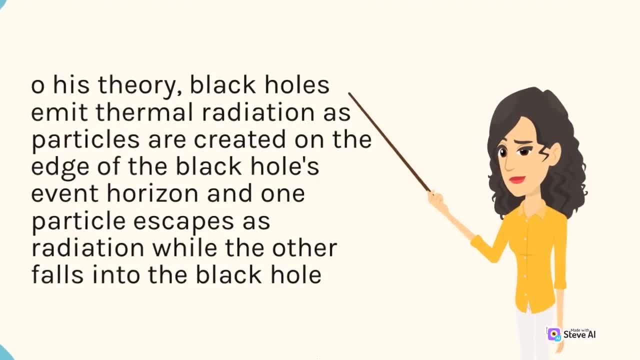 Ultimately, the study of cosmic rays is a testament to our curiosity and our desire to understand the mysteries of the universe. Ultimately, the study of cosmic rays is a testament to our curiosity and our desire to understand the mysteries of the universe. on the edge of the black hole's event horizon and one particle escapes as radiation, while the other 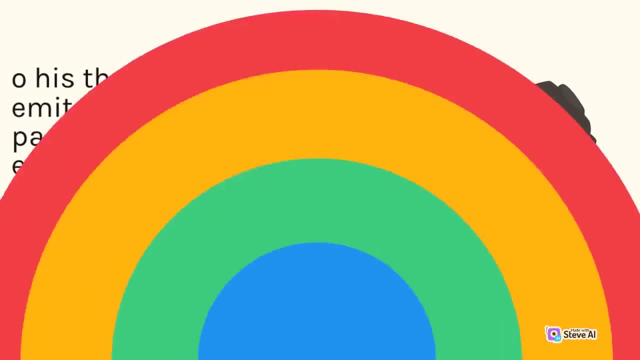 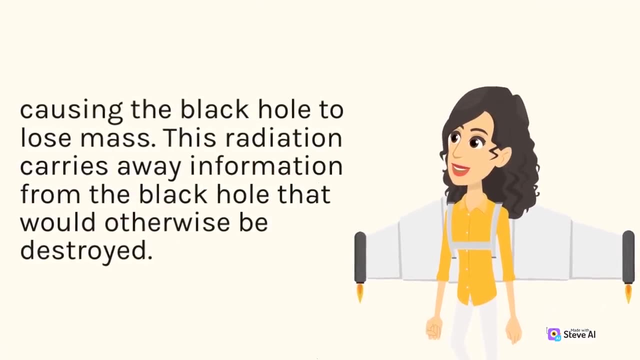 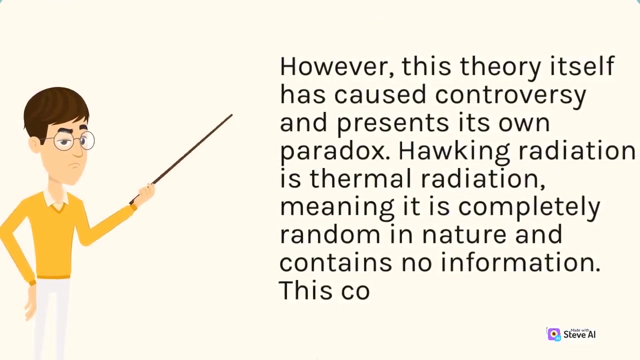 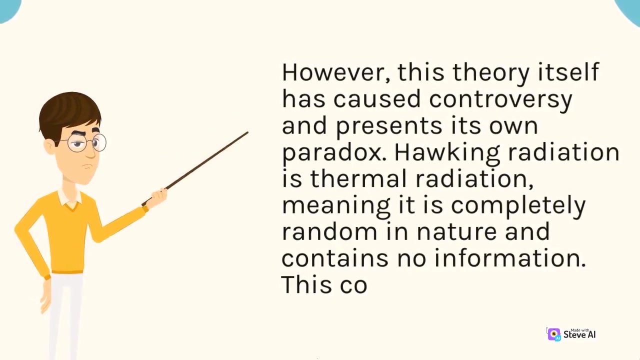 falls into the black hole, causing the black hole to lose mass. This radiation carries away information from the black hole that would otherwise be destroyed. However, this theory itself has caused controversy and presents its own paradox. Hawking radiation is thermal radiation, meaning it is completely random in nature and contains no information. This co 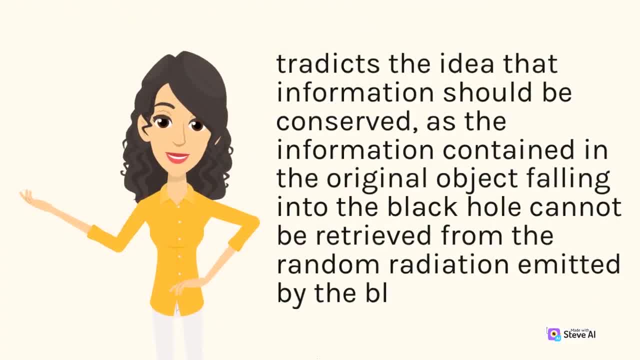 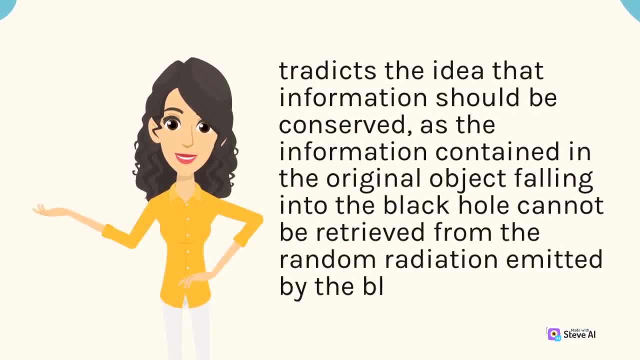 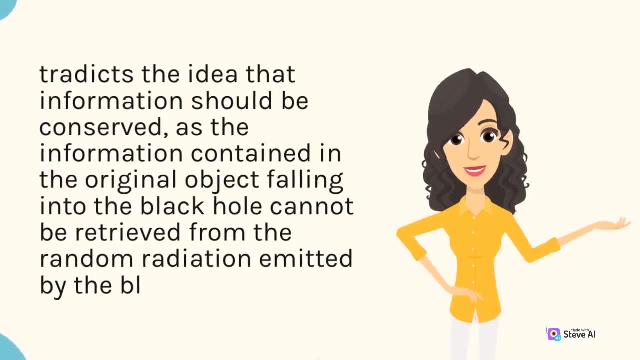 predicts the idea that information should be conserved, as the information contained in the original object falling into the black hole cannot be retrieved from the random radiation emitted by the BL. Predicts the idea that information should be conserved, as the information contained in the original object falling into the black hole cannot be retrieved from the random radiation emitted by. 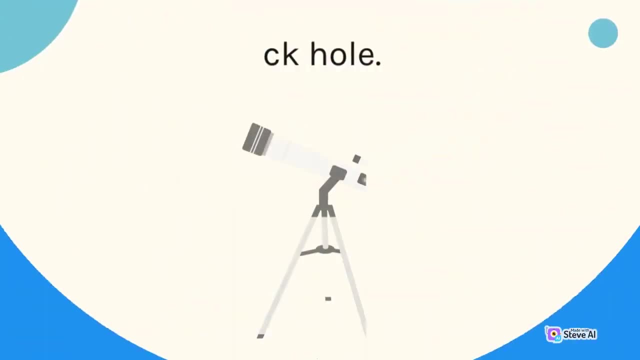 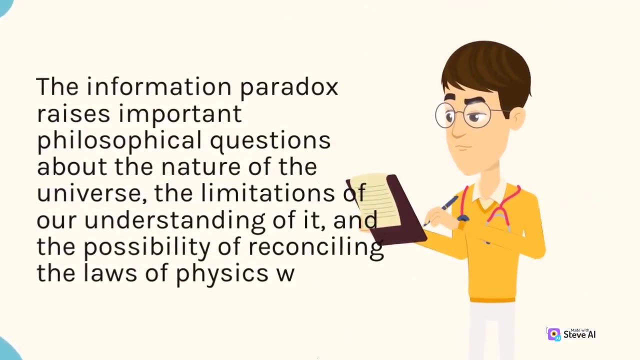 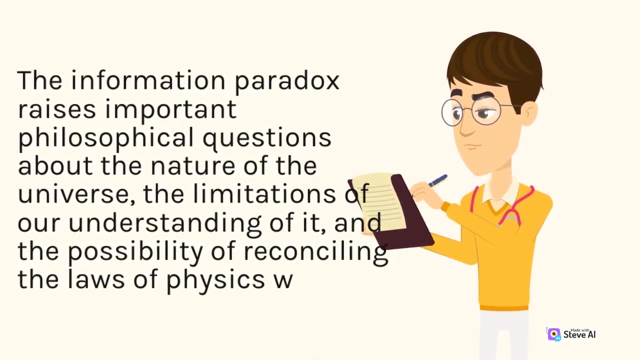 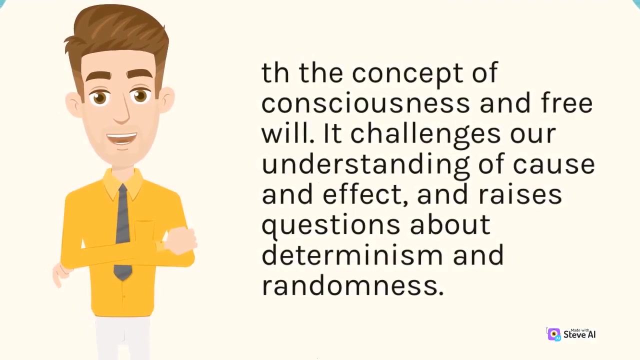 the BL CK Hull. The information paradox raises important philosophical questions about the nature of the universe, the limitations of our understanding of it and the possibility of reconciling the laws of physics, W, TH, The concept of consciousness and free will. It challenges our understanding of cause and 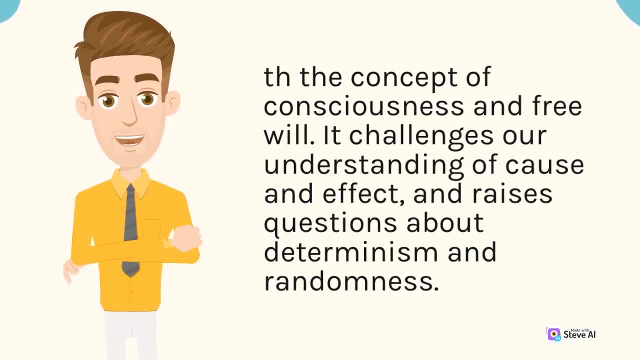 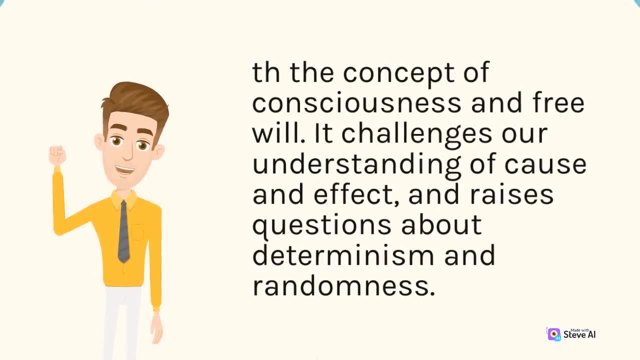 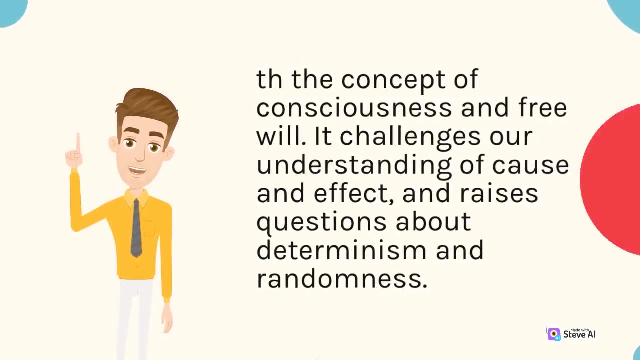 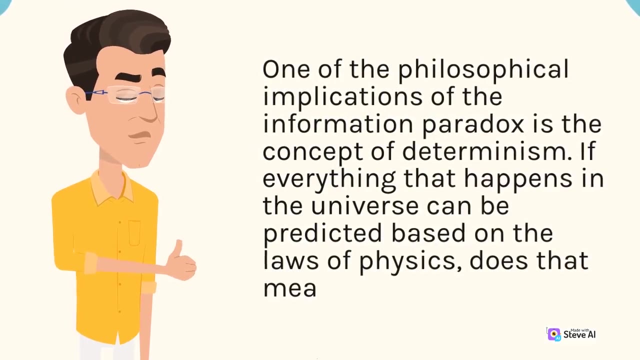 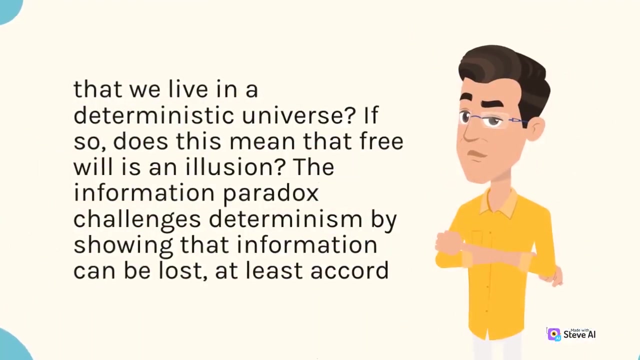 effect and raises questions about determinism and randomness. W K TH Re unwanted versions of this nonsense. talk Any现在 RussianENSU CK Hull. One of the philosophical implications of the information paradox is the concept of determinism. If everything that happens in the universe can be predicted based on the laws of physics, does that mean that we live in a deterministic universe? If so, does this mean that free will is an illusion and we have a fantasy of light because of that? f colours. 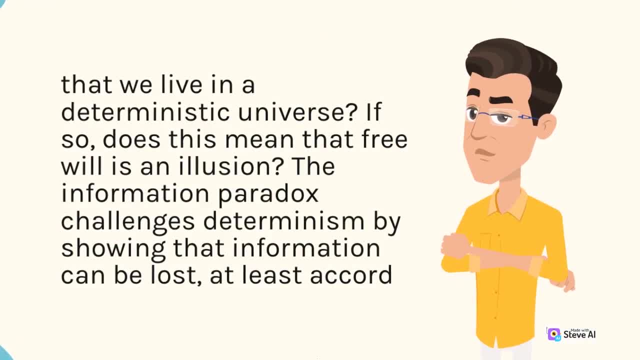 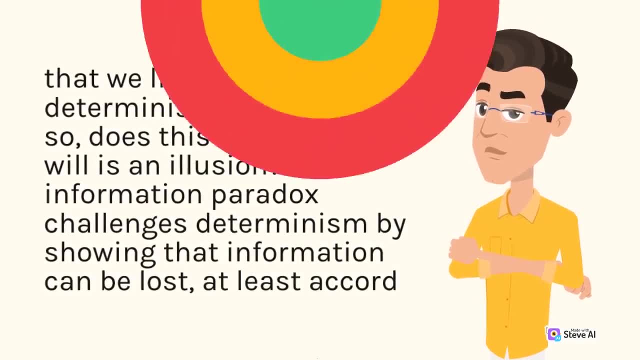 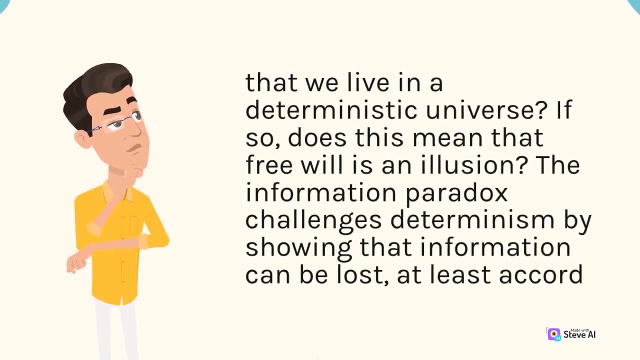 M TH Anesen, Anesen, Anesen- illusion. The information paradox challenges determinism by showing that information can be lost at least a chord, That we live in a deterministic universe? If so, does this mean that free will is an illusion? The information paradox challenges determinism by showing that. 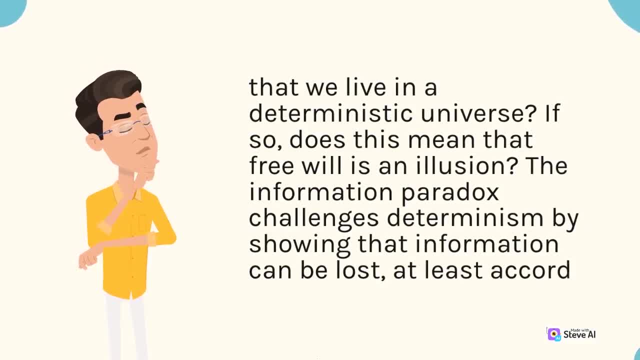 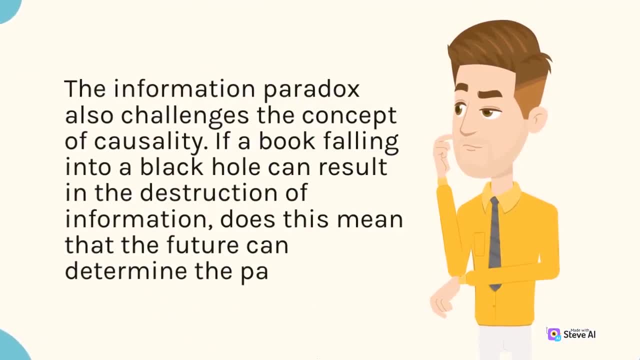 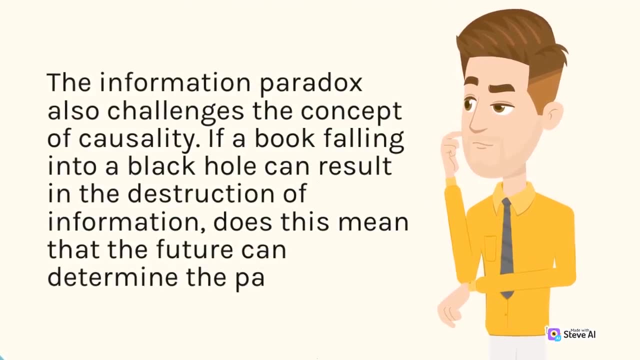 information can be lost at least a chord Ng to the laws of classical physics. The information paradox also challenges the concept of causality. If a book falling into a black hole can result in the destruction of information, does this mean that the future can? 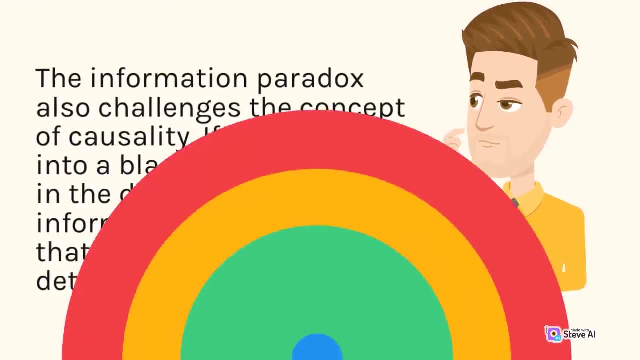 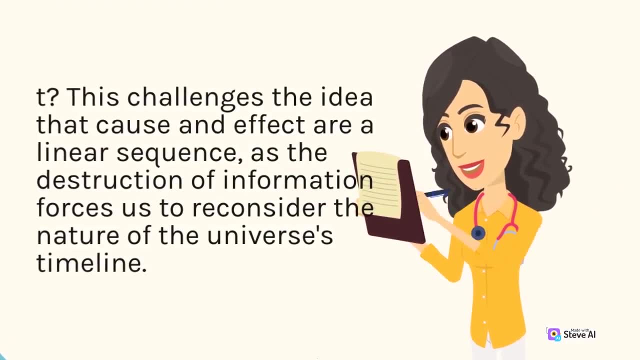 determine the pa. T. This challenges the idea that cause and effect are a linear sequence, as the destruction of information forces us to reconsider the nature of the universe's timeline. T. This challenges the idea that causality is a linear sequence, as the destruction of information forces us to. 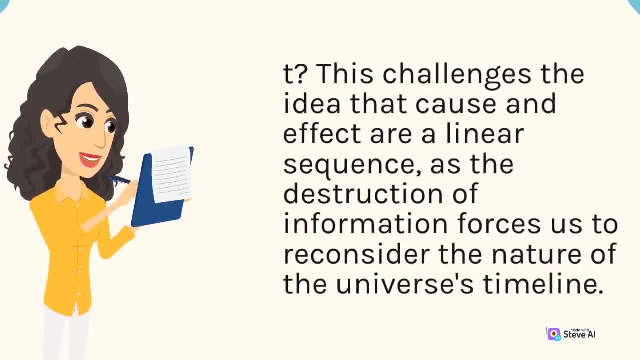 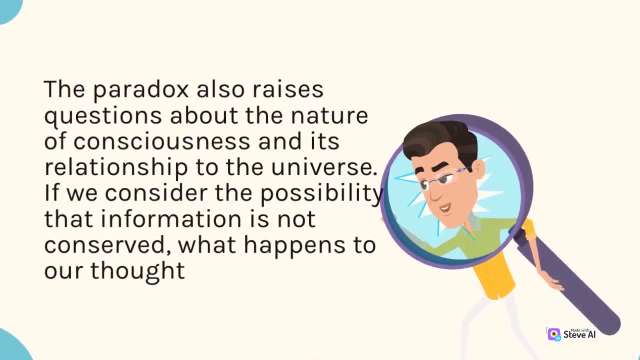 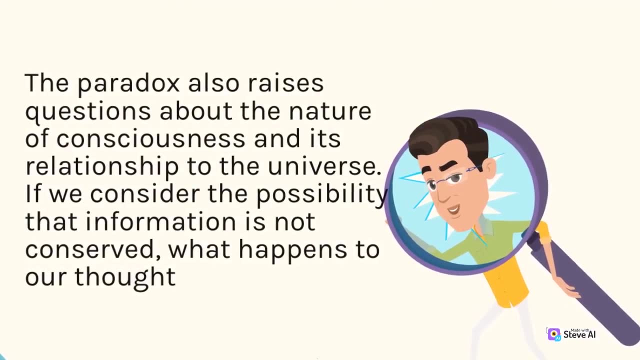 determine the cause and effect are a linear sequence, as the destruction of information forces us to reconsider the nature of the universe's timeline. The paradox also raises questions about the nature of consciousness and its relationship to the universe. If we consider the possibility that information is not conserved, what happens? 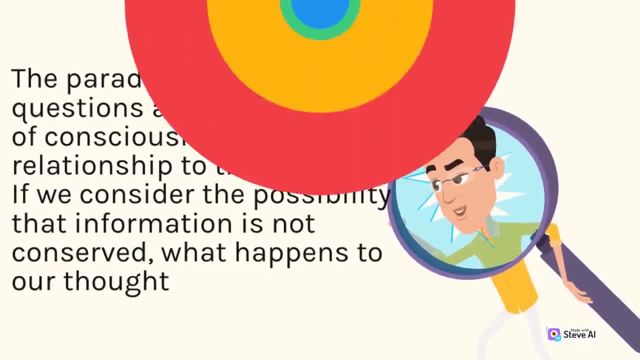 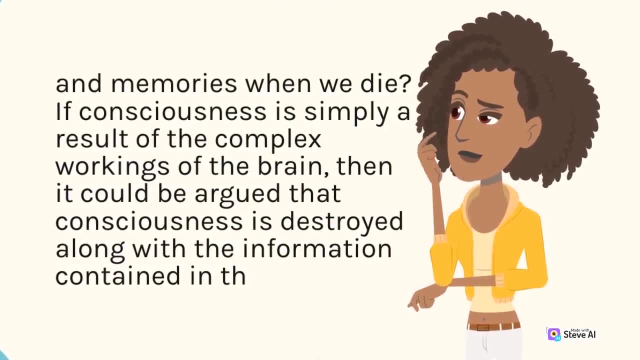 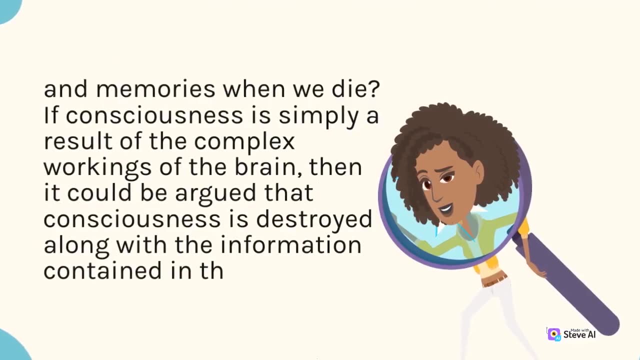 to our thought And memories when we die. If consciousness is simply a result of the complex workings of the brain, then it could be argued that consciousness is destroyed along with the information contained in TH And memories when we die. If consciousness is simply a result of the complex workings, 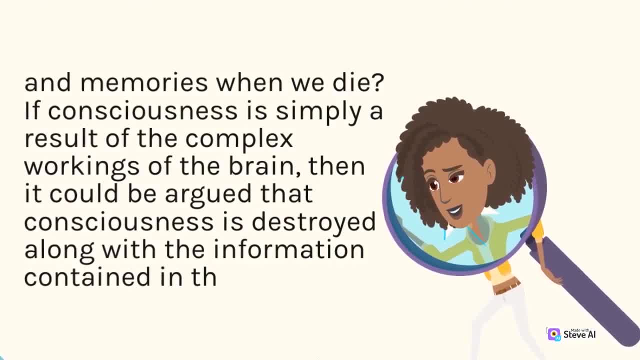 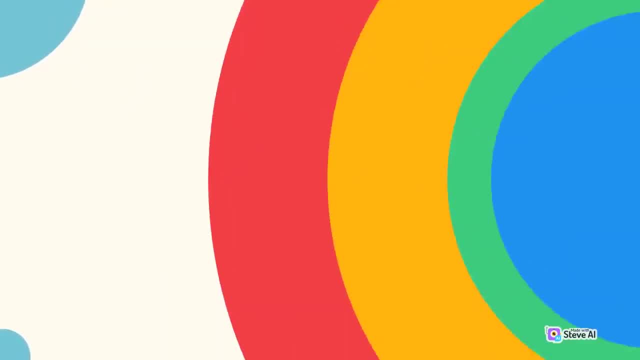 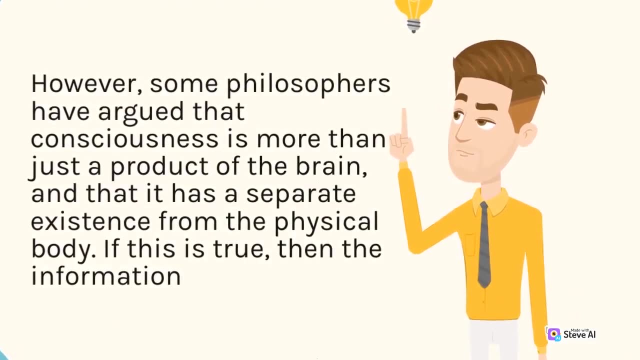 of the brain, then it could be argued that consciousness is destroyed along with the information contained in TH Brain. However, some philosophers have argued that consciousness is more than just a product of the brain and that it has a separate existence from the physical body. If this is true, then the 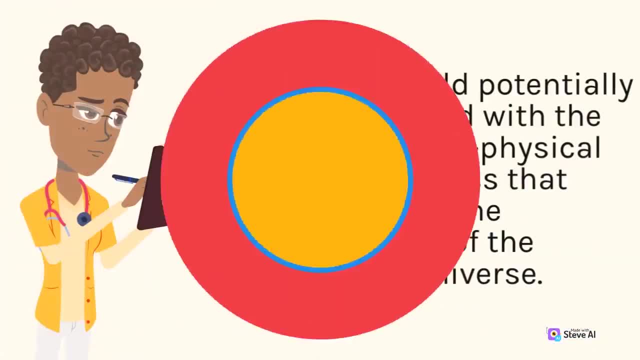 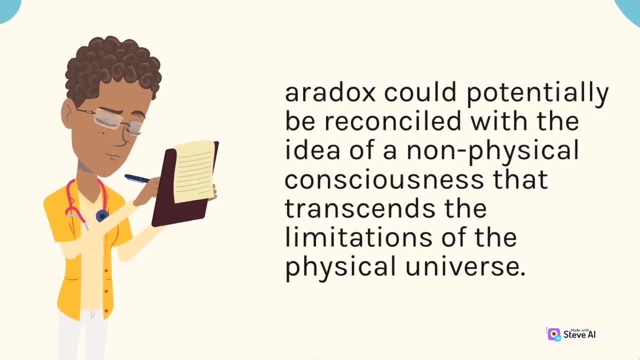 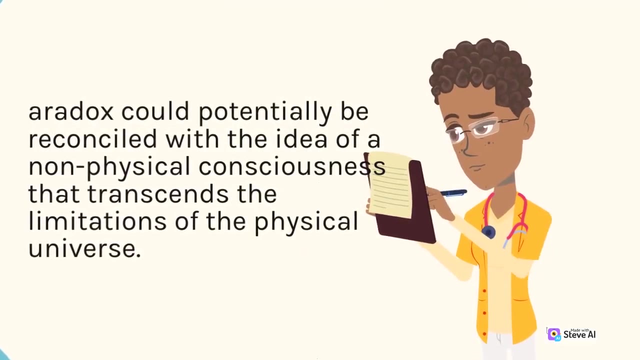 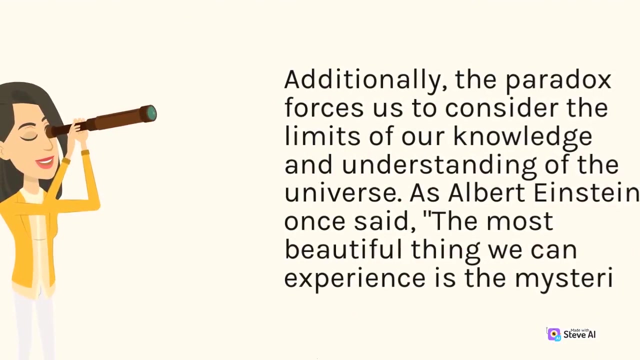 information contained in TH is destroyed along with the information contained in TH. The paradox could potentially be reconciled with the idea of a non-physical consciousness that transcends the limitations of the physical universe. Additionally, the paradox forces us to consider the limits of our knowledge. 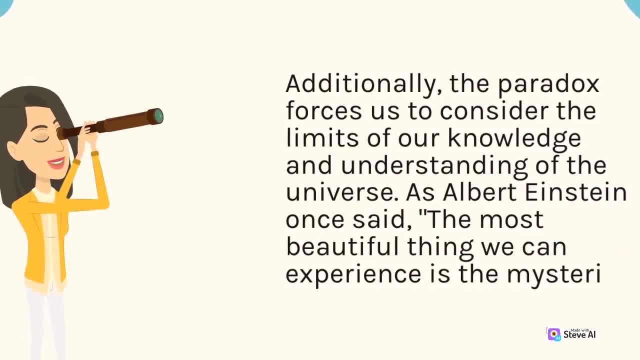 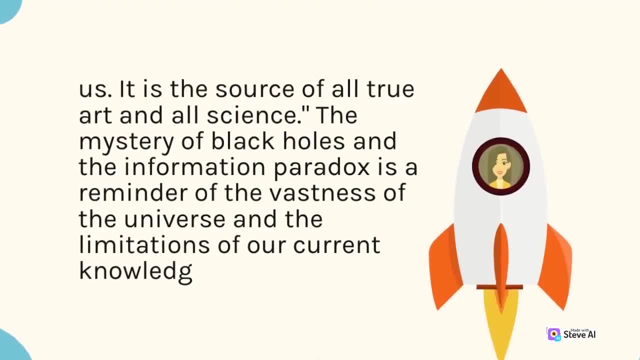 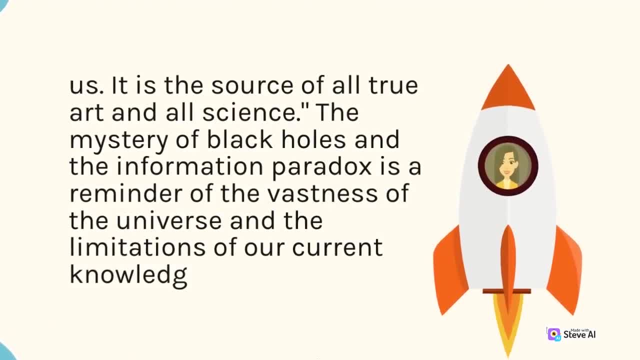 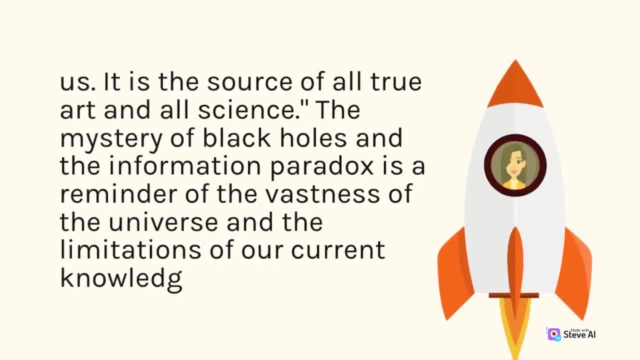 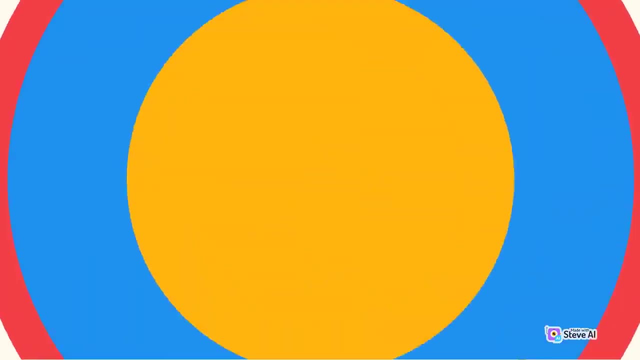 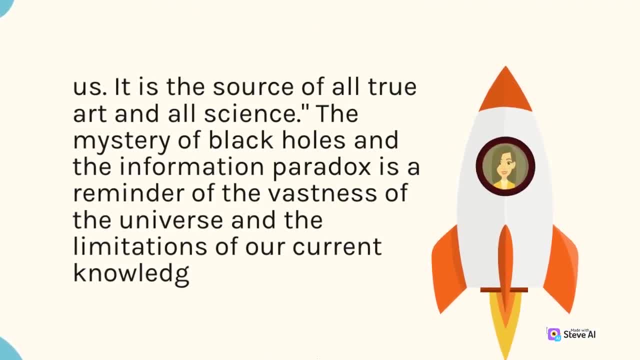 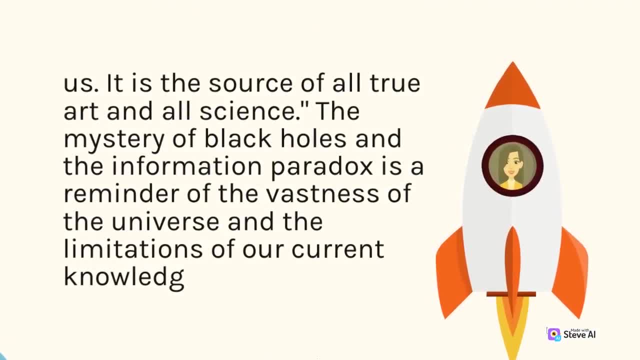 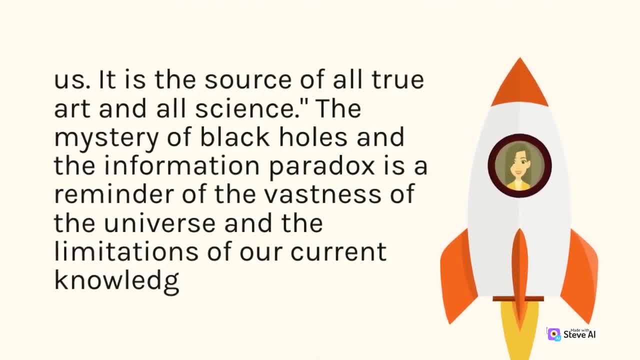 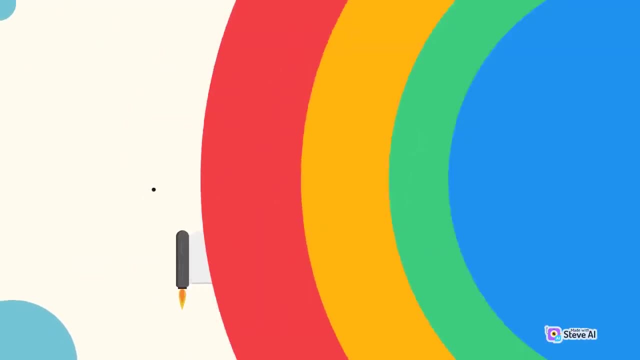 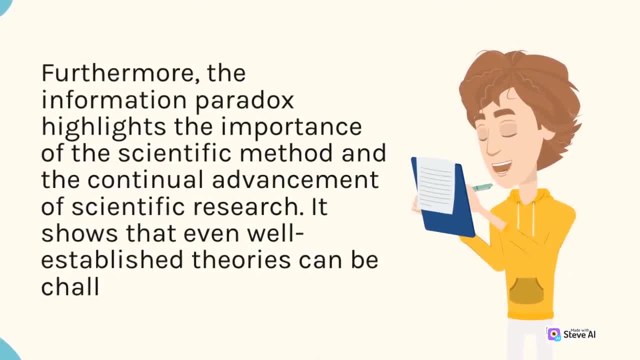 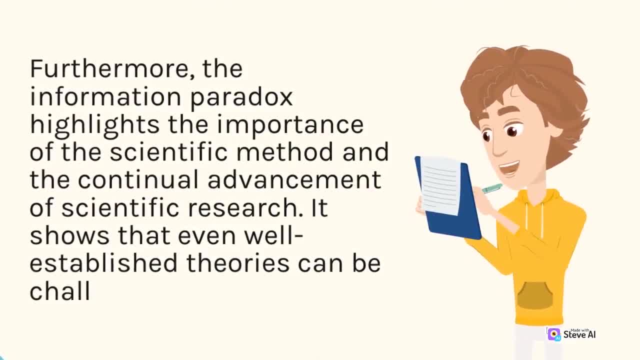 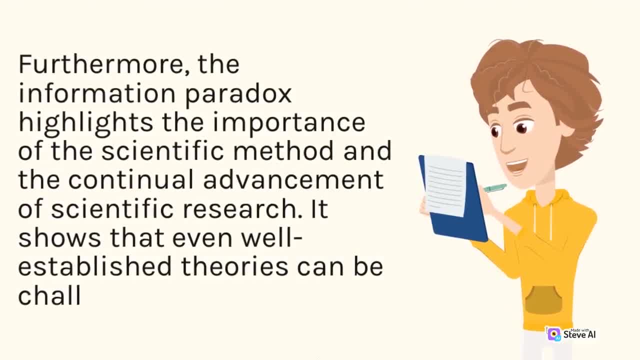 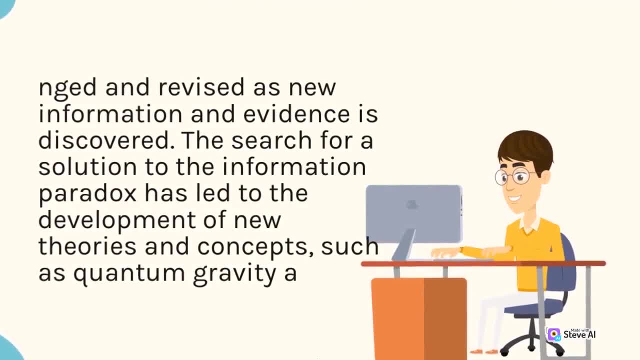 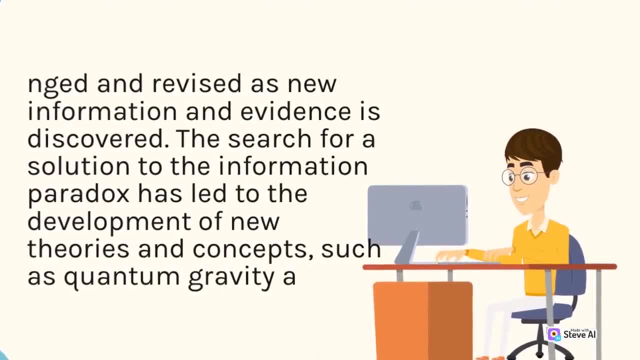 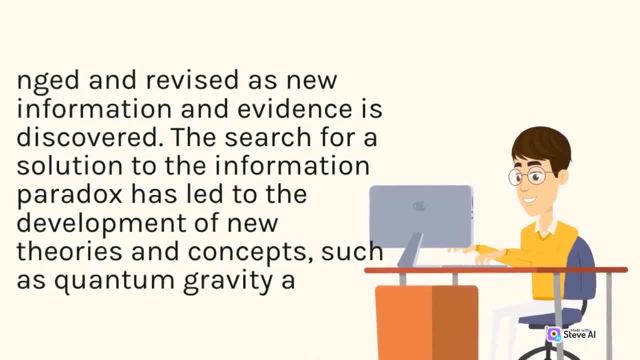 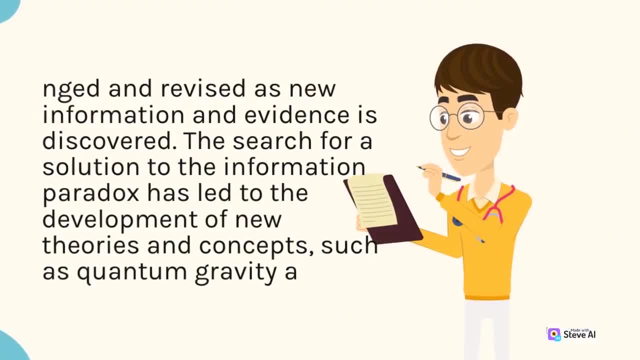 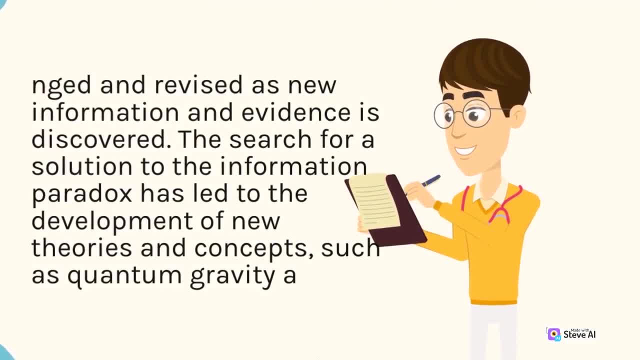 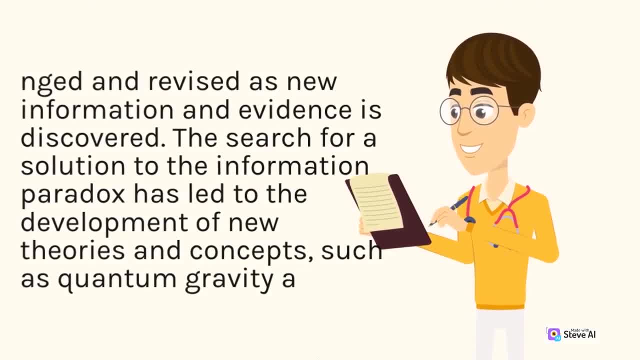 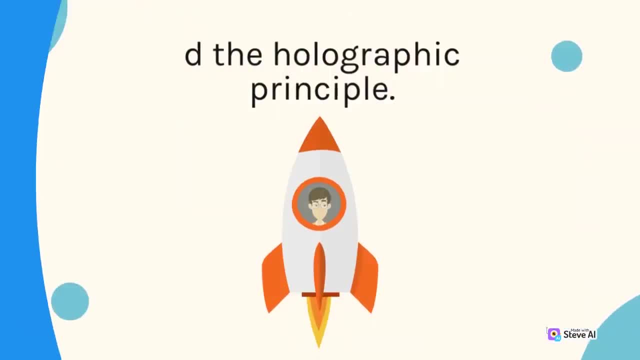 The most powerful thing in the universe is the knowledge and understanding of the universe. The most powerful thing in the universe is the knowledge and understanding of the universe. The most powerful thing in the universe is the knowledge and understanding of the universe. the holographic principle, The information paradox, also has implications for the future. 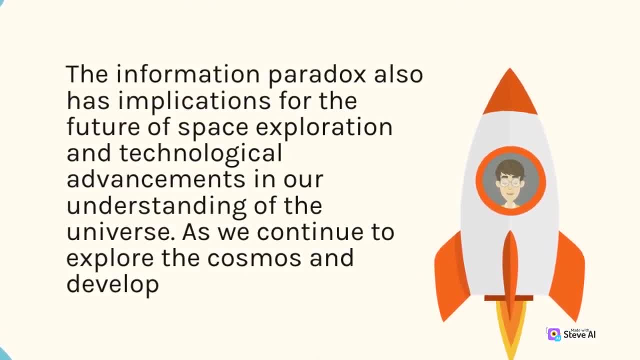 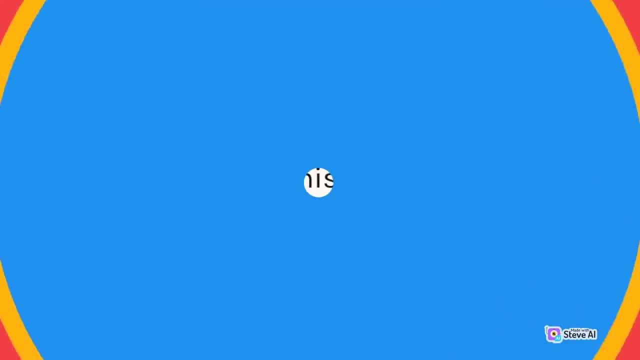 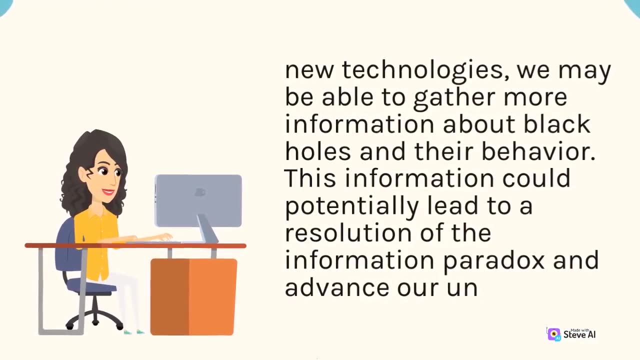 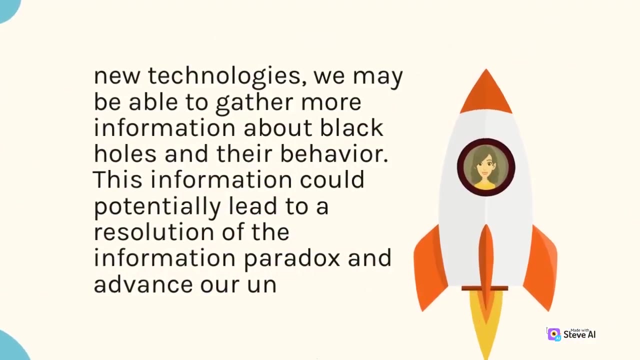 of space exploration and technological advancements in our understanding of the universe. As we continue to explore the cosmos and develop new technologies, we may be able to gather more information about black holes and their behavior. This information could potentially lead to a resolution of the information paradox and advance our own new technologies. We may be 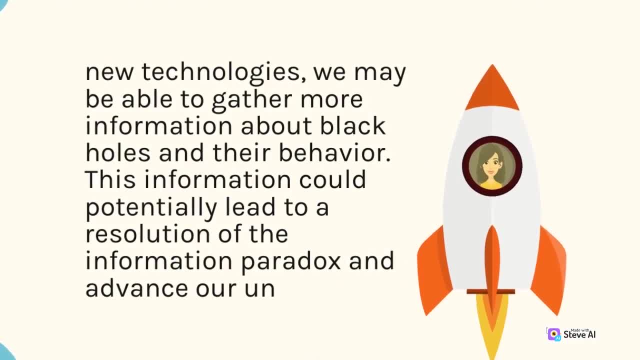 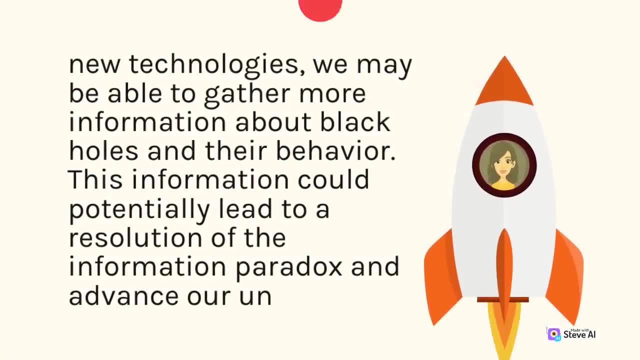 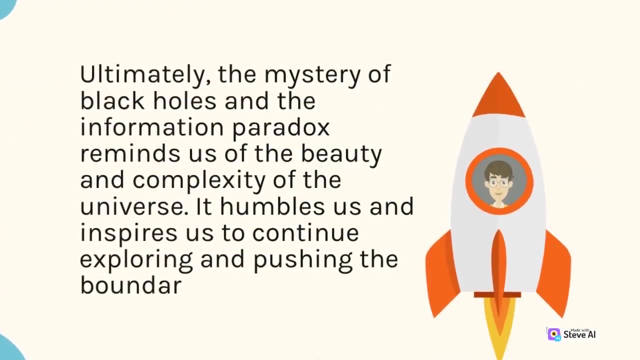 able to gather more information about black holes and their behavior. This information could potentially lead to a resolution of the information paradox and advance our own understanding of the universe. Ultimately, the mystery of black holes and the information paradox reminds us of the beauty and complexity of the universe. It humbles us and inspires us. 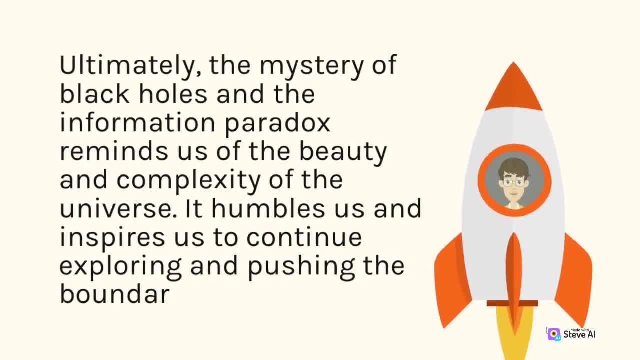 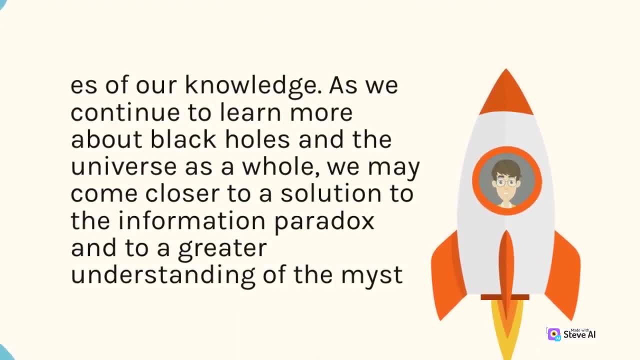 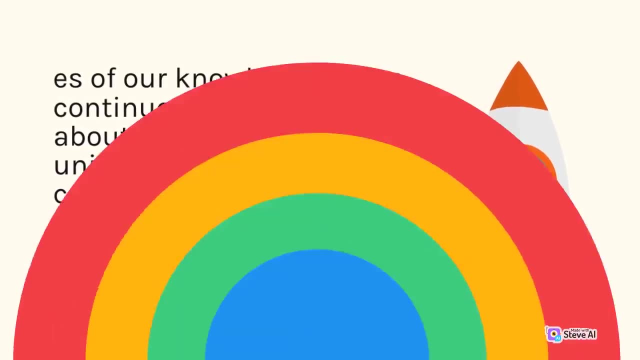 to continue exploring and pushing the bounder. As of our knowledge, as we continue to learn more about black holes and the universe as a whole, we may come closer to a solution to the information paradox and to a greater understanding of the mist. As of our knowledge, as we continue to learn more about black holes and the universe as. 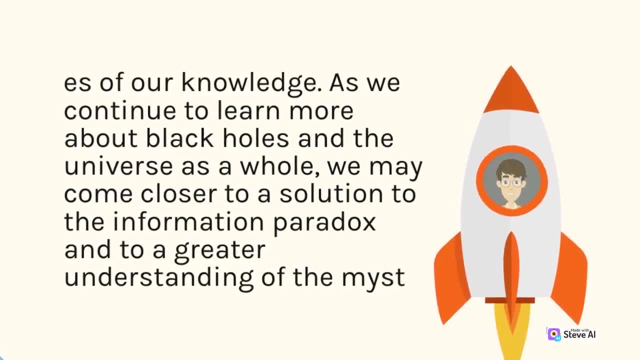 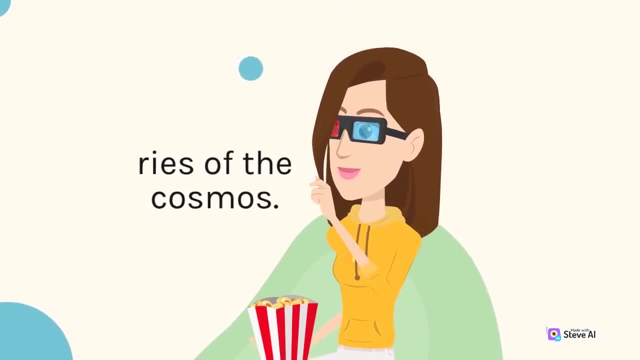 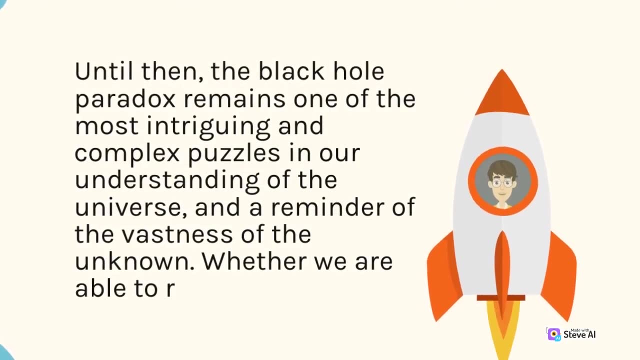 a whole, we may come closer to a solution to the information paradox and to a greater understanding of the mist Reese of the Cosmos. Until then, the black hole paradox remains one of the most intriguing and complex puzzles in our understanding of the universe and a reminder of the vastness of the unknown. 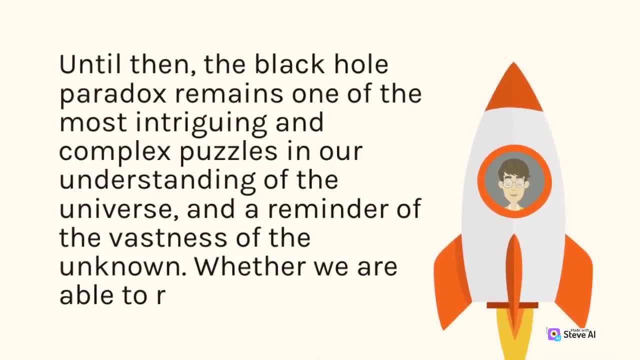 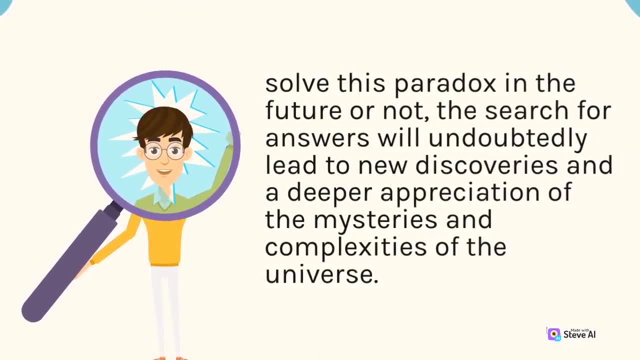 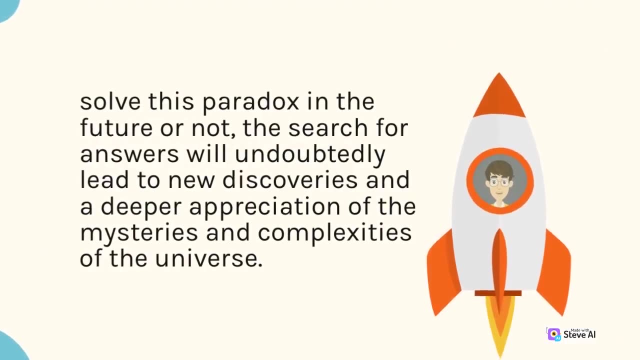 Whether we are able to are Solve this paradox in the future or not, the search for answers will undoubtedly lead to new discoveries and a deeper appreciation of the mysteries and complexities of the universe. Solve this paradox in the future or not, the search for answers will undoubtedly lead.